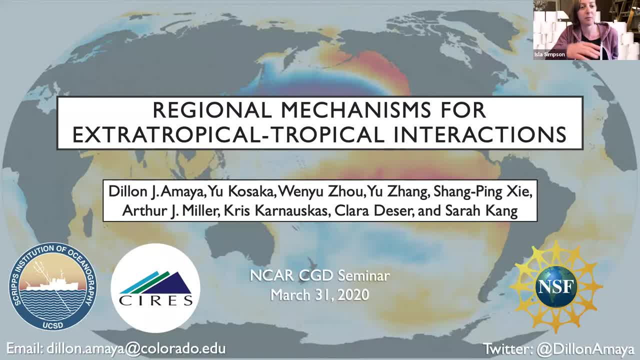 interrupt Dylan, Otherwise we'll leave questions till the end and then raise your hand then as well, and we'll take them in order. So I'll leave it to Dylan. Awesome, thank you, Aila, and thanks everybody for logging on. Obviously, we're always looking for questions. we're always waiting for. 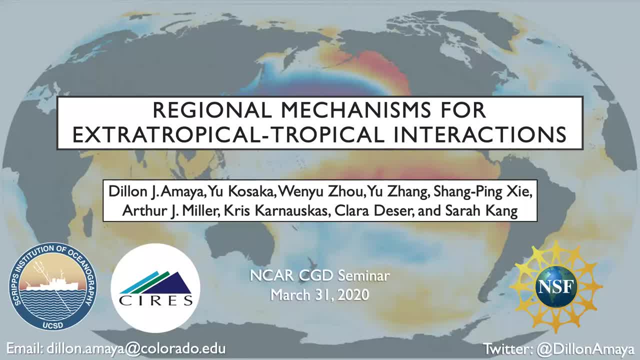 logging on. Obviously, this is a unique situation. Hopefully all the technical hiccups have been fixed and we're good to go. I'll do my best to keep my internet going throughout all of this, but if I drop out, I promise I'll sign right back in. 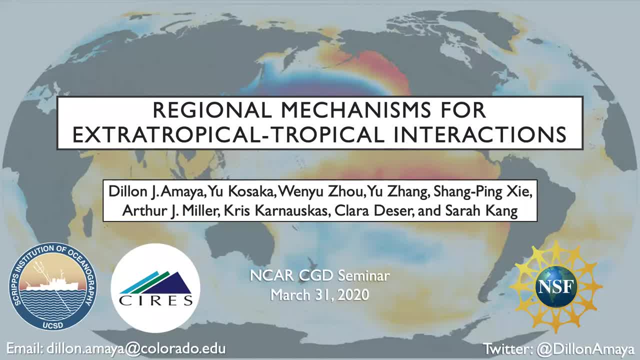 So yeah, as Isla said, I'm a new postdoc at Ceres at the University of Colorado, primarily working with Chris Kanouskis, but Clara Desser has also sort of adopted me in her group in CACS. So, as Isla mentioned, I'm around NCAR a lot when NCAR is open, so I'm looking forward. 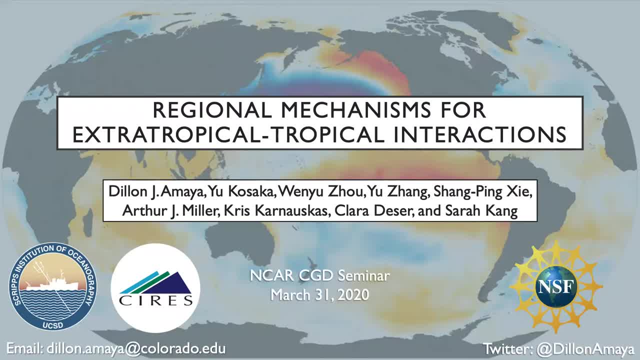 to meeting a lot of you and hopefully discussing research with you all and collaborating, moving forward. But today I want to talk a little bit about- well, I guess a lot about what I've done as part of my PhD work and then, hopefully, if we have time, I'd like to talk. 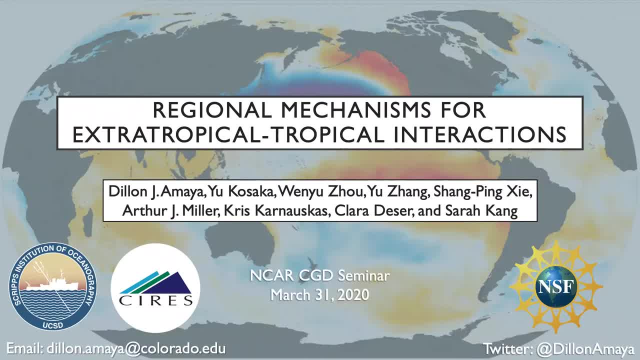 about some of the stuff that I've been doing as part of my postdoc and just sort of motivate what I've been doing. So I'm going to talk about some of the things that I've done in the past and also what I'm looking to do in the future. I sort of want to zoom out for a second and discuss sort. 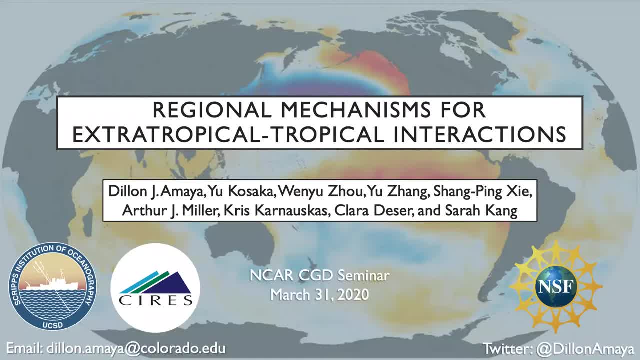 of broadly how the vast majority of research has sort of looked at this problem of extra tropical-tropical interactions and the way they've done that historically. And I'm trying to advance my slides. Let's see, Maybe if I click. how's that? There we go, Okay. So 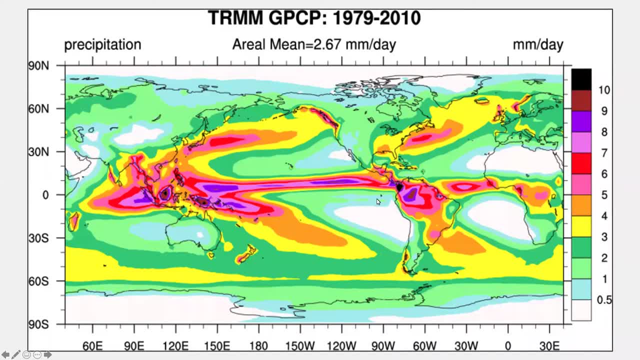 the vast majority of papers that have looked at this sort of topic have primarily been focused on: well, what's governing the position of the mean ITCV, which you can see pictured here, and what sort of like high-latitude climate perturbations influences where the 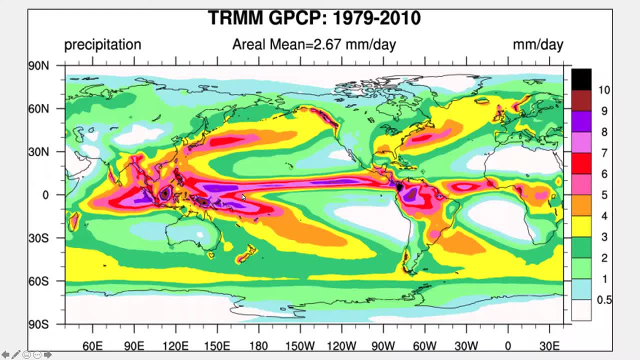 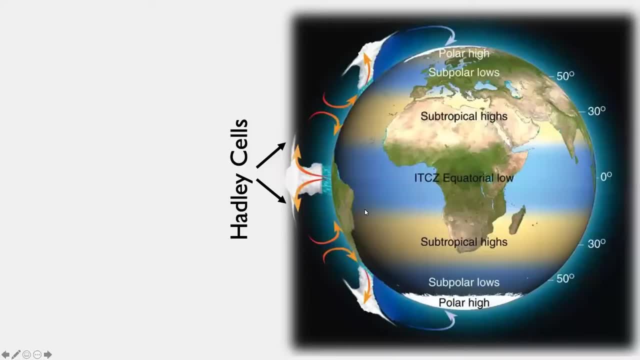 ITCV will be in sort of this equilibrium climate state, And so let's just very briefly talk about sort of this ITCV, sort of zonal mean perspective. We can collapse the atmospheric circulation into this sort of zonal mean view and when we do this we can see these broad. 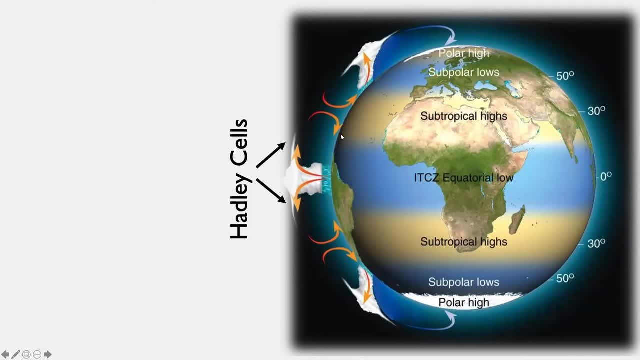 heavy-cell circulations. I exist in both hemispheres where the surface trade winds converge at the surface and that gives you moist convection near the equator, in the form of the ITCV, which is the upward branches of both of those Hadley cells, And this sort of precipitation centroid can be. 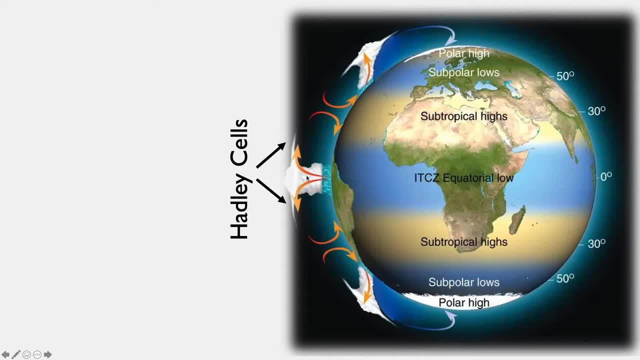 marked where the ITCV is in the zonal mean And if we think about what the atmosphere is doing when it creates these circulations, I mean its primary goal is to transport energy. It's trying to smooth energy gradients throughout the climate system. 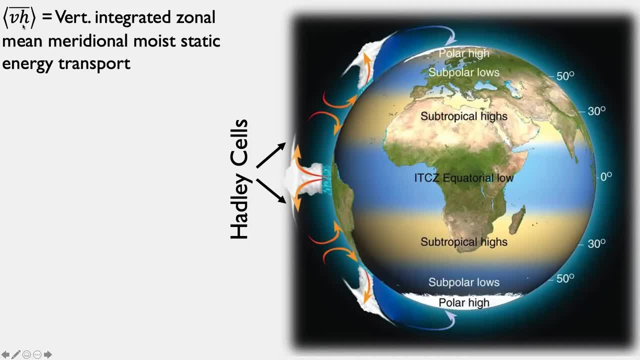 So we can quantify energy through this sort of bracketed VH bar term which will be vertically integrated. zonal mean meridional moist static energy transport in the atmosphere, And in the atmosphere moist static energy increases with height. So if we think about the direction, 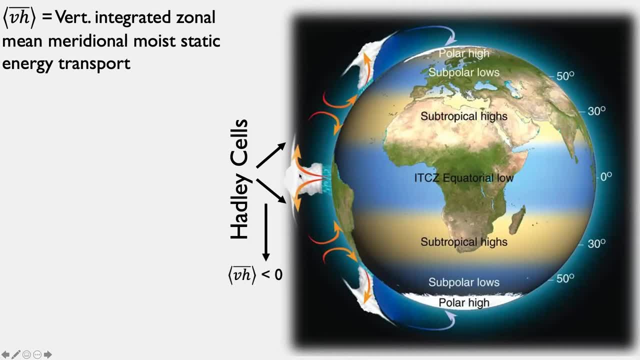 and sign of moist static energy transport in the atmosphere. it's going to be positive in the northern hemisphere and negative in the southern hemisphere, in the same direction as the poleward branches of the atmosphere. So we can quantify energy through this sort of bracketed VH bar term, which will be vertically. 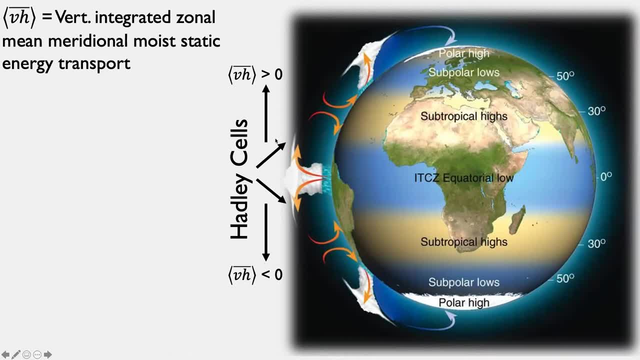 integrated zonal mean, So the Zonal Mean Framework- can be found where the moist static energy transport- meridional moist static energy transport- is zero in this case, So that precipitation centroid can be found where this is zero. But even this picture is a little bit too simplistic, because in 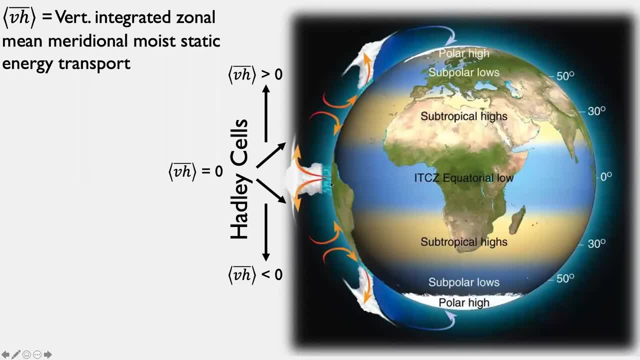 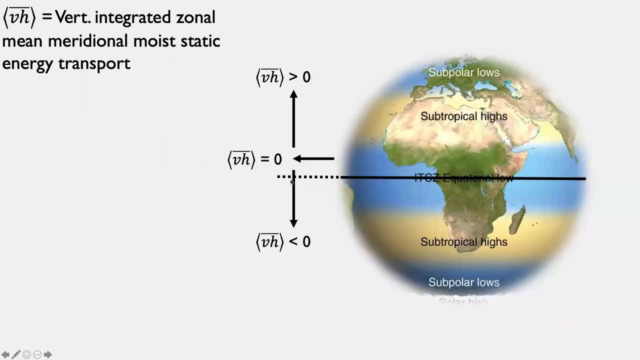 this picture, the ITCV is sitting directly on the equator, And we know that in the real world that's not necessarily the case case. So let's simplify even further and we'll put the ITCZ in a more realistic setting. 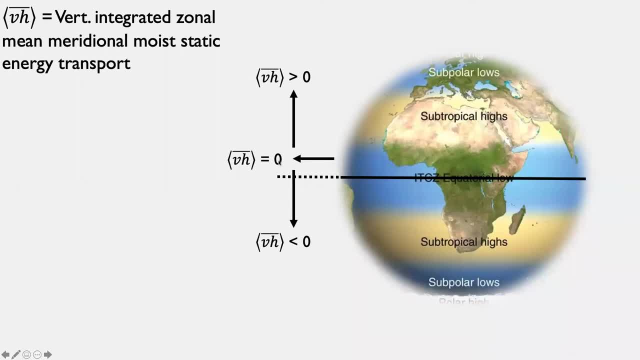 In this case we'll represent our ITCZ by this sort of vertical line here going out into our atmosphere, and we'll push it just a little bit further north of the equator, And now when we do that we can see that our equator as we sort of extend it out into. 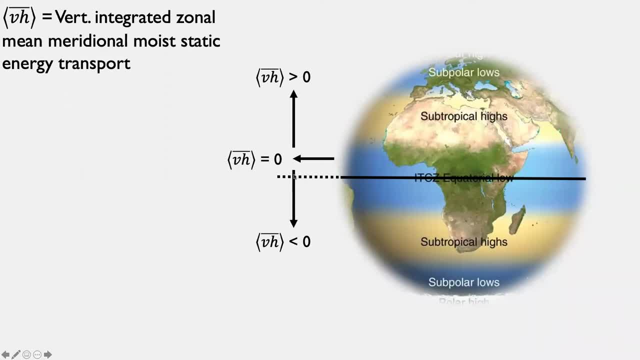 space sort of crosses our upward branch of the Hadley cell in the southern hemisphere. So really the cross-equatorial atmospheric energy transport is negative here. So our atmosphere in the real world in the annual mean sense is transporting energy from the northern hemisphere to the southern hemisphere, because in the annual mean the 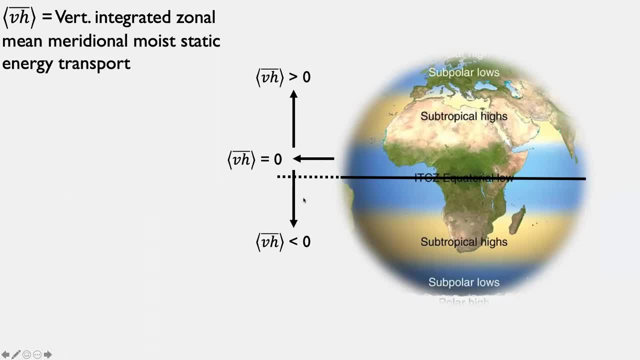 southern hemisphere is colder in this case, And so this leads to this sort of zonal mean ITCZ theory, that the position of the ITCZ is roughly proportional to the negative of the cross-equatorial atmospheric energy transport, And this works. This works pretty well. 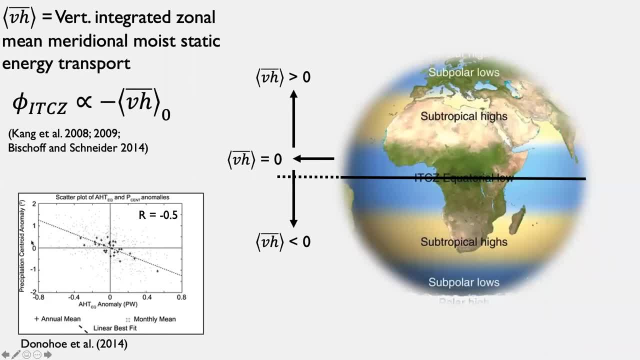 If you look at observations or in long climate model simulations and you look at the sort of the position of the ITCZ relative to the equator and you compare it to cross-equatorial atmospheric energy transport, you can see that they're well negatively correlated. 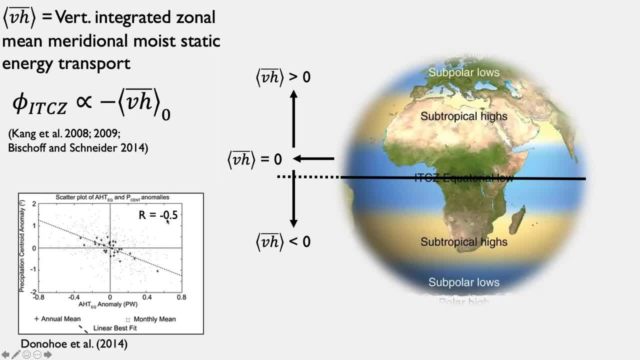 something like minus 0.5.. So this has been one classic way to sort of define what's going on with the ITCZ and it's really useful. You can think about it sort of in a paleo sense. Let's say that we just…. 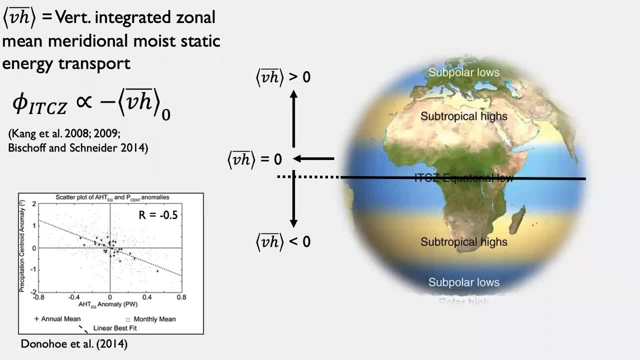 Let's say that we just dropped a massive energy perturbation on, to, say, the high northern latitude. Let's just say we had an ice sheet during the last glacial maximum, for example. And specifically, when I do this in this sort of cartoon sense, I'm sort of thinking about: 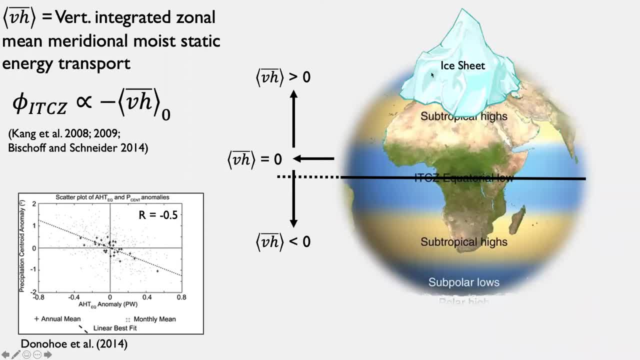 the albedo effect on the climate system and not the mechanical forcing of having a three-kilometer ice sheet, but really just having something large and shiny in the northern hemisphere that cools the entire northern hemisphere. So if this were to happen, the atmosphere wants to adjust to this and wants to transport. 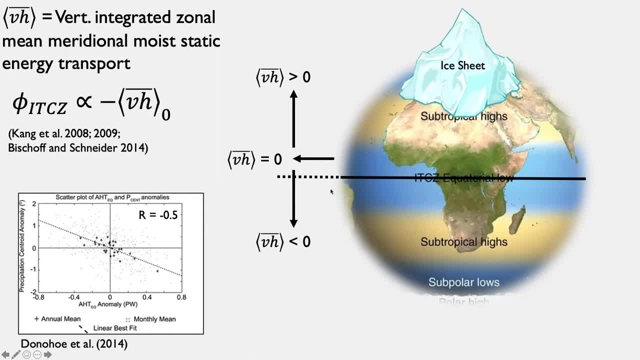 energy from the colder hemisphere to the warmer hemisphere. So if this were to happen, the atmosphere wants to adjust to this and wants to transport energy from the warmer hemisphere, And so what's going to happen is that the ITCZ will shift southward and our cross-equatorial 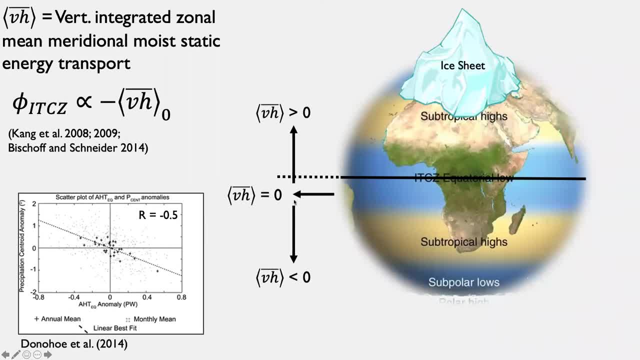 energy transport is actually going from this warmer hemisphere to the colder hemisphere in this case. So this is just a really nice universal way to sort of think about these large-scale atmospheric energy transports. And now we know… So we've sort of established this in the last maybe 15-odd years. 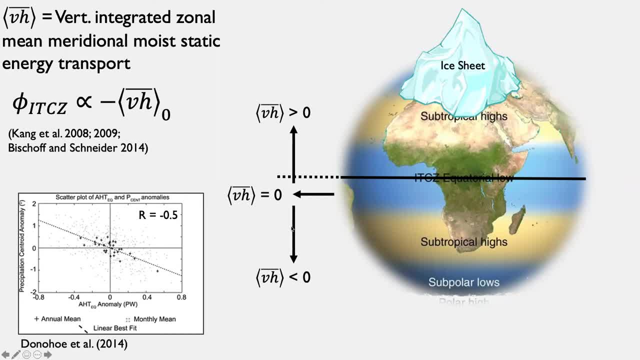 And more recently we've been zooming out even further in trying to understand how ocean transport modulates this atmospheric response. So this has sort of led to this so-called sticky ITCZ paradigm where the Ekman response to this atmospheric circulation shift, if you will, provides oceanic energy transport. 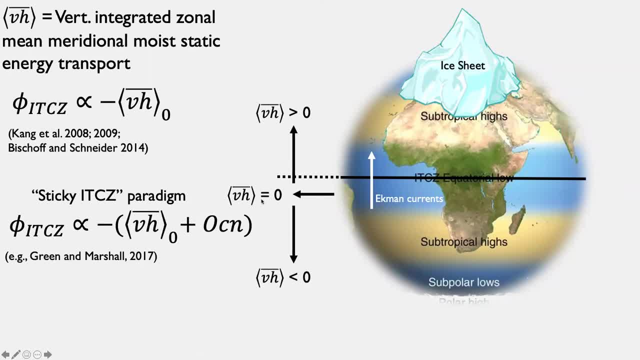 that is in the same direction as the atmospheric transport And because of that the atmosphere actually doesn't end up having to work as hard to smooth energy gradients, because the ocean is compensating for some of that. So ultimately what happens is the ITCZ just doesn't shift as far for a given energy. 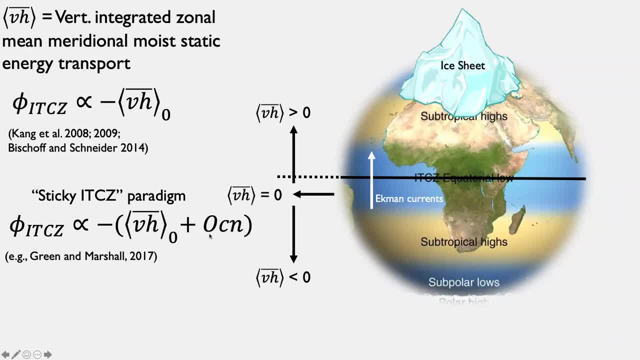 perturbation in the real world, because we have the ocean that compensates for some of that, And so this is just again just a very broad overview of a very diverse and vast array of literature that I find really useful to sort of understand these large-scale energetic. 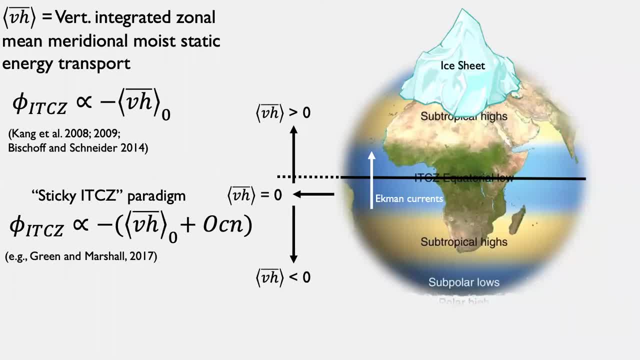 perturbations. Ultimately, what I'm going to be talking about today is not…. Okay, This is not strictly related to this, but I find it really useful to sort of motivate this idea that we need to move beyond this zonal mean perspective. 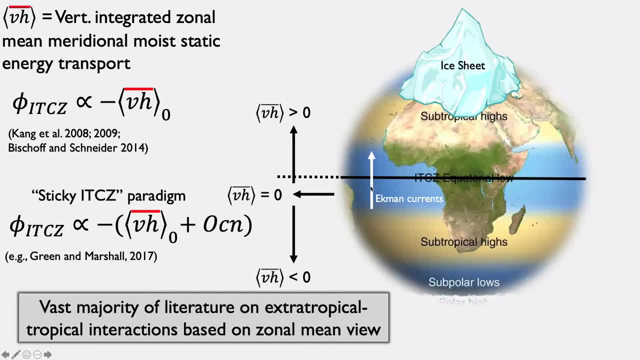 As I said, the vast majority of the literature that has thought about these high-latitude impacts on tropical precipitation, tropical wind and, to some extent, tropical temperature have primarily been focused on this zonal mean view, because it simplifies the problem. 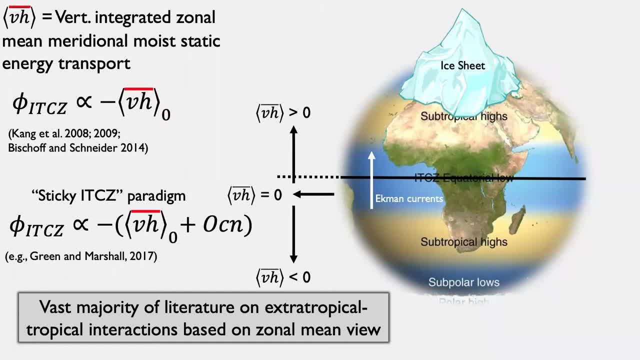 really well, right, It collapses the dynamics and it closes energy budgets. better, It's just… It's more… It's a simpler way to look at things. but we don't look at the zonal mean because we find it particularly useful for the real world. 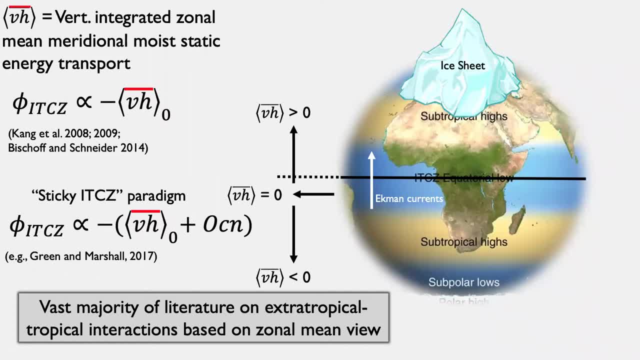 We look at it because it helps us inform our understanding, but we don't live in the zonal mean right. So part of what motivates my research, both as part of my PhD and looking forward as part of my postdoc, is to sort of look at these regional mechanisms for driving these high-latitude. 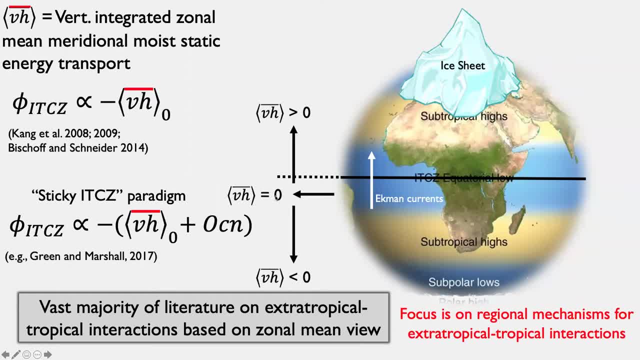 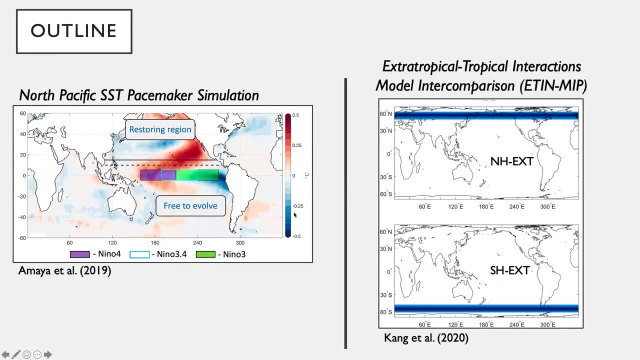 signals down into the deep tropics where they can satisfy in the zonal mean, this sort of large-scale… Okay, …large-scale energetics framework. So to do that, today I'm going to spend… Almost all the talk today will be focused on my PhD work, which was part of…. 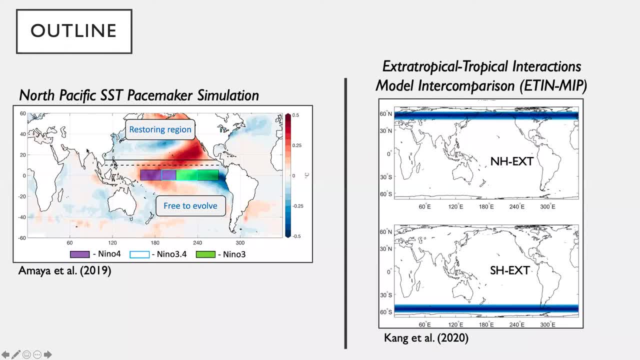 Analyzing part of the simulation, which ended up being a North Pacific pacemaker experiment, and I'll dive into this in much more detail to explain everything that's going on. But I'm hoping that at the end, if I have some time, I'll show some preliminary results. 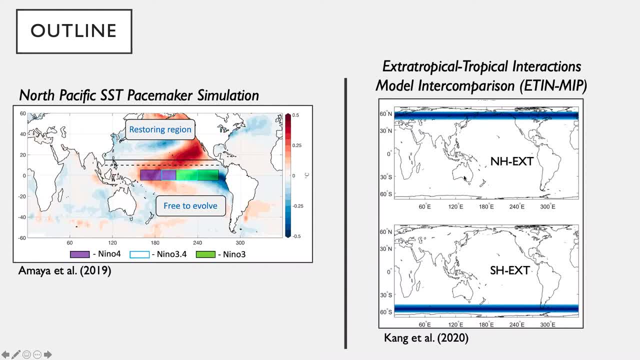 analyzing a different set of simulations that also look at sort of regional… Okay, …mechanisms for high-latitude forcing. So with that I'll just dive right into sort of this first topic, this first set of simulations, and explain one array of literature that has historically looked at regional mechanisms. 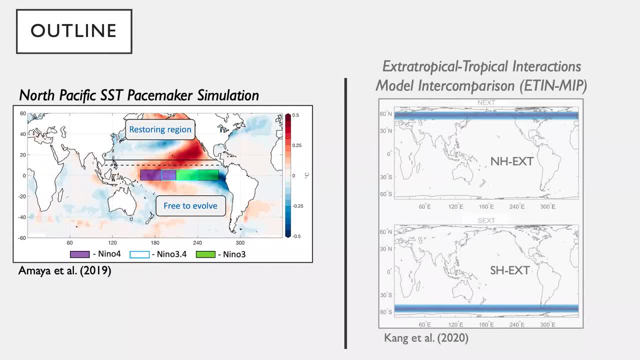 for high-latitude to tropical forcing. And when I say high-latitude, I just mean outside of the tropics, I don't mean like Arctic necessarily. I do mean sort of mid-latitude to extra-tropical, to tropical. Okay, 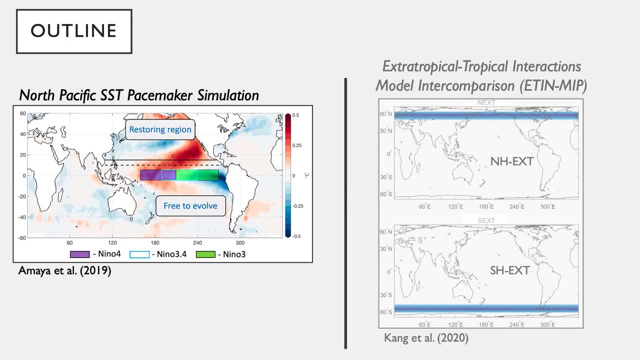 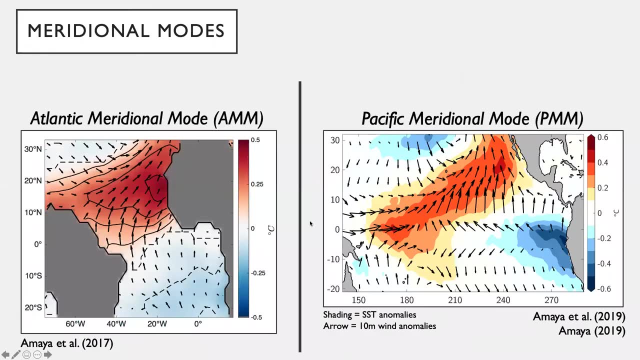 And I'm going to start with the… Okay, …multiplexer interactions And one set of literature that has focused on this for a long time. whether they recognized it or not, or whether that was their purpose, was this group of people that were thinking? 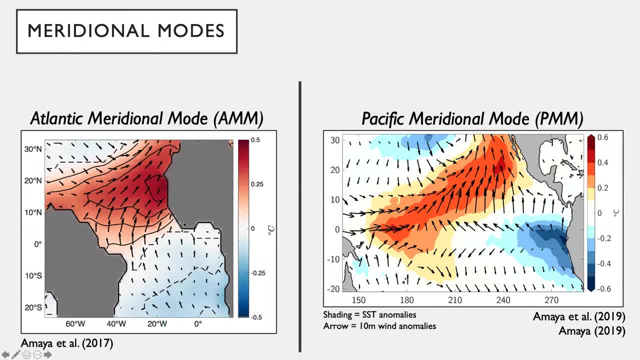 about meridional modes, these modes of climate variability that can be found in the tropical Atlantic, in the tropical Pacific and, to some extent, within the tropical Indian Ocean. And these meridional modes are modes of climate variability, modes of coupled climate variability. 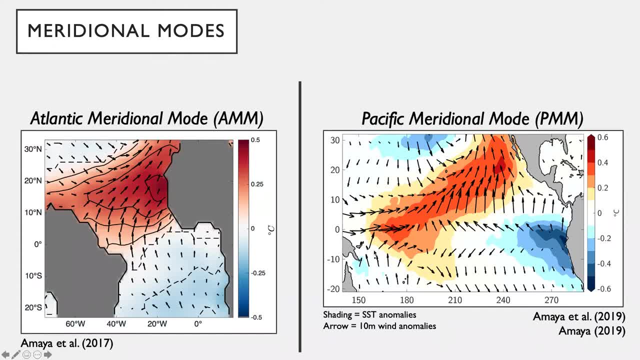 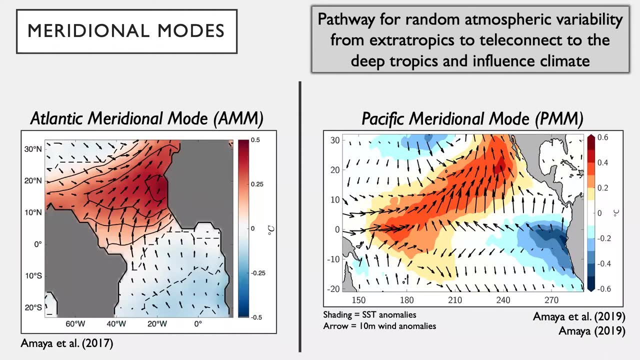 modes of SST and surface winds primarily, but also to some extent precipitation, And they act as pathways. They act as regional pathways for random atmospheric variability from the extra-tropics to make their way into the deep tropics and influence all sorts of climate variability, including. 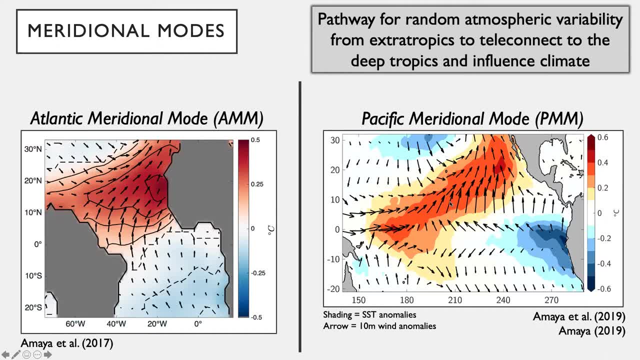 winds along the equator, SST things like ENSO will be the big focus for today, as well as rainfall within the tropics, So I think that's a really good way for these sort of extra-tropical signals to get to the deep tropics. 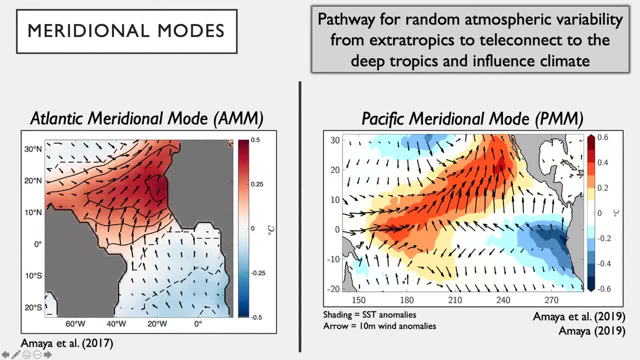 And primarily when we think about meridional modes- and I will mention that I'll be mostly speaking about the PMM today- the Pacific component of this, the high-latitude forcing in this case isn't necessarily energy perturbations. 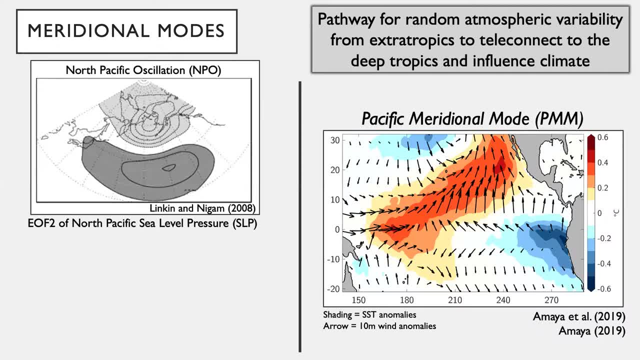 It's really the high-latitude forcing is this sort of stochastic atmospheric variability. that's happening in a transient sense in the North Pacific and it can make its way into the deep tropics. It can trigger all sorts of interesting air-sea interactions. 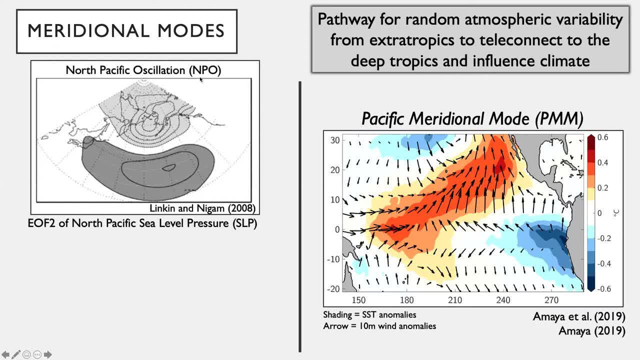 That being said, the atmospheric circulation that we're going to be talking about, this North Pacific Oscillation, can, in theory, be triggered by sort of thermodynamic anomalies at high latitudes, And that's sort of a talk or discussion for another day. 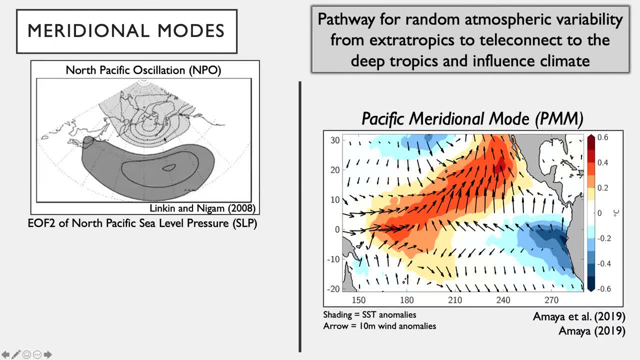 But if anybody's interested maybe we can talk about it at the end. But generally speaking, a PMM event, this Pacific Meridional Mode event is triggered in the wintertime when the North Pacific Oscillation is strongest. This is represented by the second event. 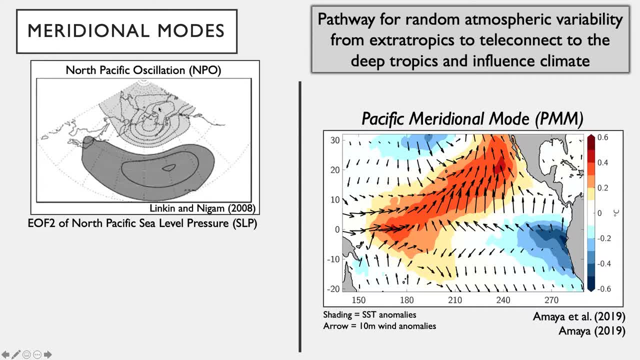 This is the EOF of North Pacific Sea Level Pressure Anomalies and it's just represented by this dipole of sea level pressure anomalies, And so the idea here is that you have a large-scale circulation in sort of the subtropical to mid-latitude North Pacific and it can dip down into the deep tropics and influence the 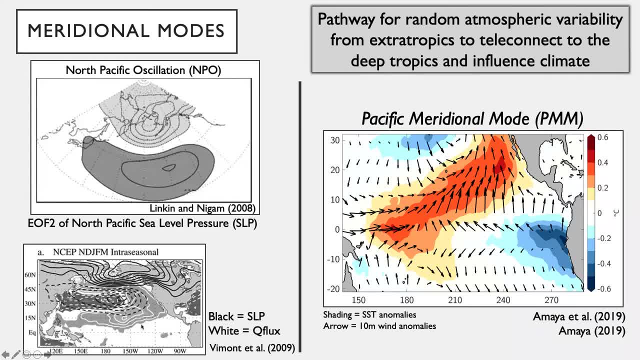 strength of the trade winds. So we can see that impact on the underlying ocean in this plot here. So these black contours are again the NPO, except it's a different phase than what's shown here. It's just the opposite phase. 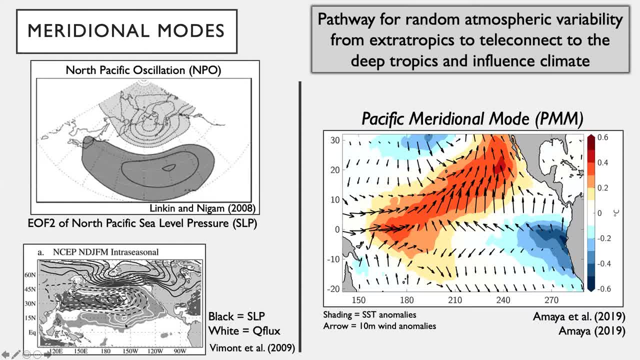 And the white contours are again the NPO. The white contours here are Q-flux, just showing you the direction of energy between the atmosphere and the ocean, And so basically what you can see here is that the southern lobe of the NPO here, if 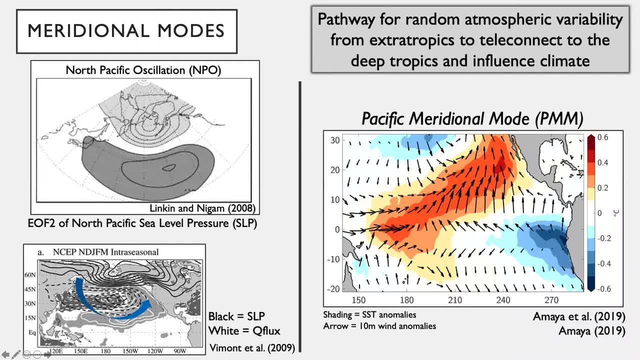 the circulation is going in this direction. it dips down into the deep tropics. It weakens, it anomalously weakens- the trade winds which drives a turbulent heat flux into the ocean and we can see that here, leaving an SST footprint in sort of the subtropical 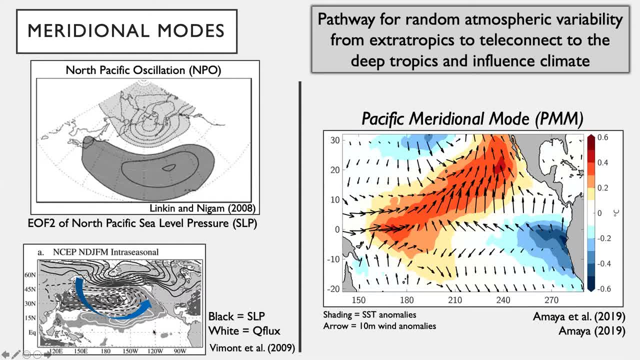 North Pacific, And this all happens sort of in the winter, early time, early springtime, Or it can happen in the winter and early springtime, But what you'll notice is that this Q-flux doesn't extend all the way to the equator. 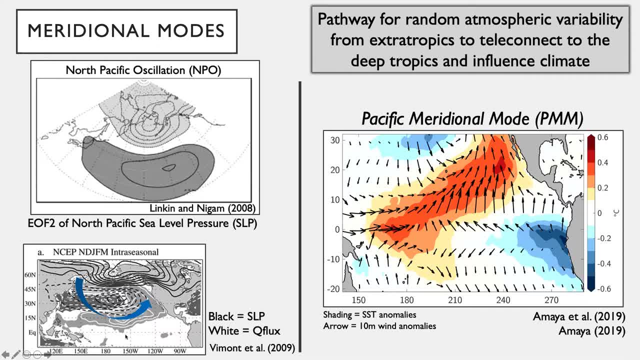 right. These anomalies have not quite made it all the way down to the deep tropics, where they can influence things like wind variability and SST along the equator. There needs to be more information here to sort of drive the teleconnection all the way. 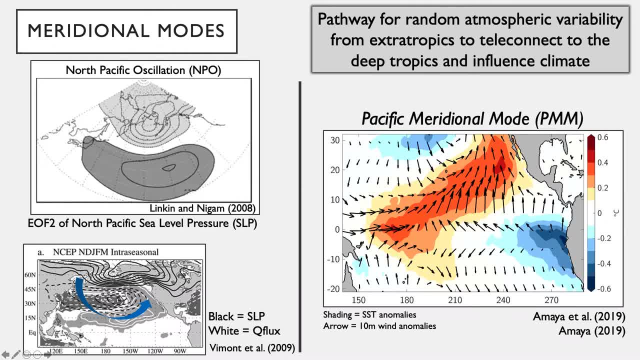 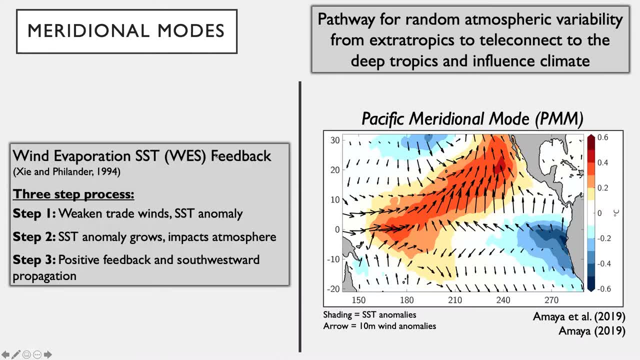 from random atmospheric variability in the extratropics to sort of this deep tropical strip. And the way that this works is through something called wind evaporation, SST feedback or WES feedback. This is one of the primary ways by which these high latitude atmospheric- again I say high- 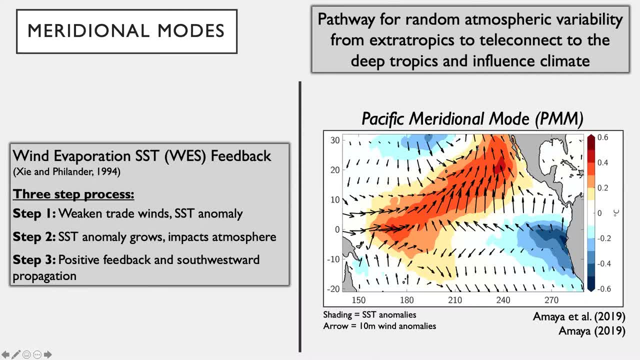 latitude, but I really just mean extratropical atmospheric variability- can make their way into the deep tropics and influence different parts of the climate system. And so this happens in sort of three processes, three steps. We can weaken the trade winds which creates an SST anomaly footprint through turbulent 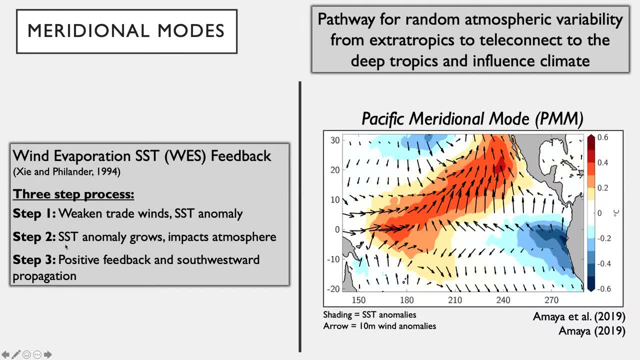 heat fluxes, and that's through the MPO that I just showed. Eventually, these SST anomalies will grow. These anomalies will grow strong enough that they can impact the atmosphere directly And then, once they're big, it generates all sorts of interesting air-sea interactions. 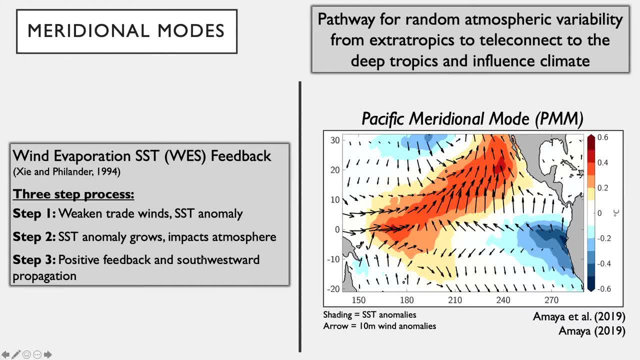 And ultimately it propagates the signal preferentially southwestward, ultimately getting it onto the equator where it can influence wind variability. it can drive westerly wind events which influence equatorial ocean dynamics and ultimately influence ENSO, which is the main focus of 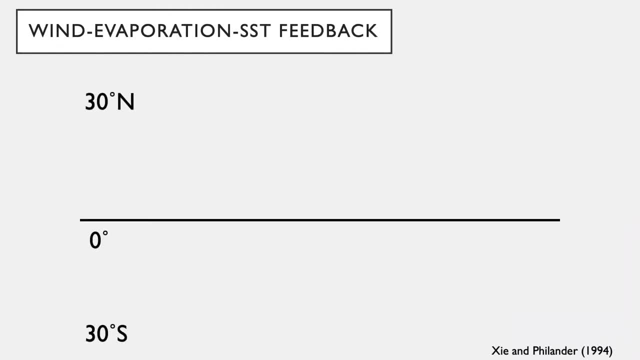 this work. So I do have a couple of questions. So I do want to illustrate that for you, sort of this idea of west feedback, because it is important for the rest of my talk. So the idea again: you have these trade winds. these mean trade winds in the Northern Hemisphere. 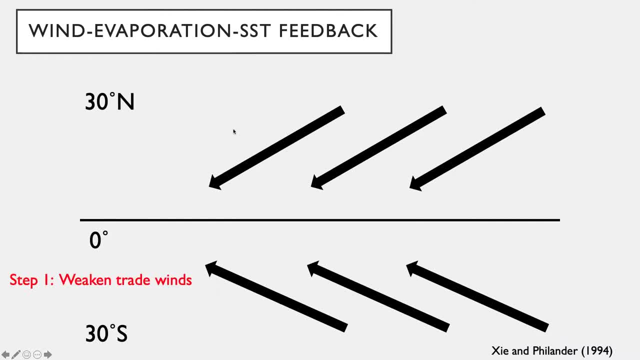 and the Southern Hemisphere. Let's just say that the MPO rolls through and we weaken the trade winds anomalously. in the wintertime We'll have some anomalous southwesterlies in the Northern Hemisphere. This will weaken the mean flow. 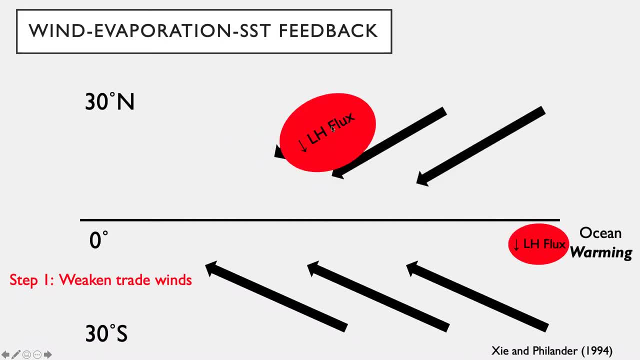 You get a positive latent heat flux down into the ocean and it creates a positive SST anomaly footprint That has not reached the deep tropics. Okay, So let's just say that the MPO rolls through and we weaken the trade winds anomalously in. 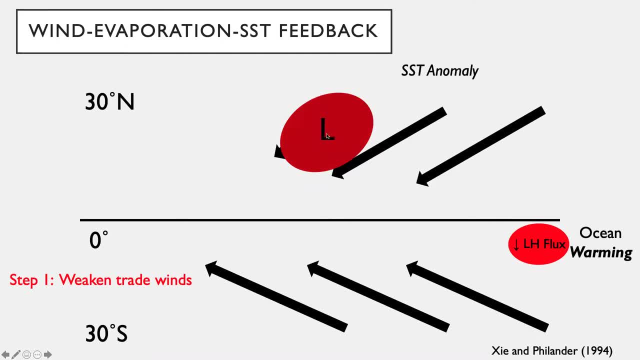 the wintertime We get a positive latent heat flux down into the ocean That has not reached the deep tropics. Eventually this will get big enough right And it'll impact the atmosphere. It'll create a localized low pressure and it'll suck in wind, suck in air from all directions. 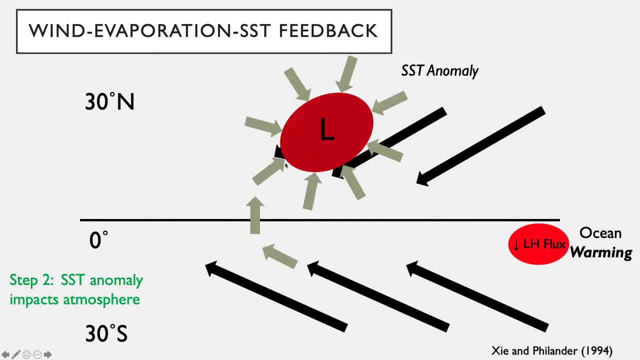 Particularly, it'll drive it across the equator, giving you this nice C-shaped bend in the wind field across the equator due to Coriolis, and it'll have impacts on the opposite hemisphere's wind field. So in this case, in the Southern Hemisphere, these surface wind anomalies will increase. 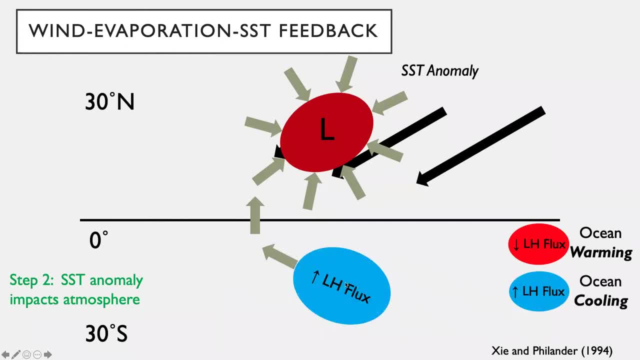 the strength of the trade winds. It'll give you a cooling effect by increasing evaporation at the surface and it'll give you a negative SST anomaly. So this is where meridional nodes really get their name. You get this meridional dipole in SST anomalies and this is sort of one really important component. 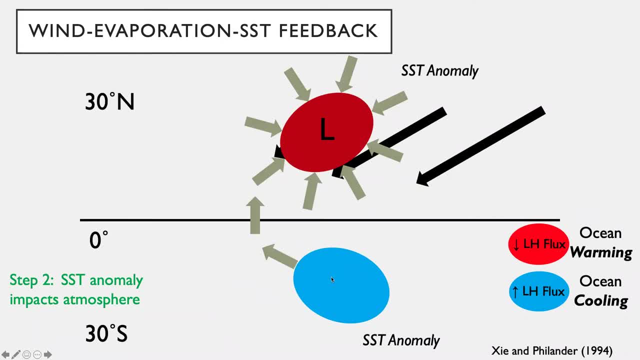 of West's feedback. There's sort of two main components that I really want to hammer home here. One: it can maintain a meridional SST gradient, So in sort of a quasi-equilibrium sense, if we go back and sort of think about our large-scale. 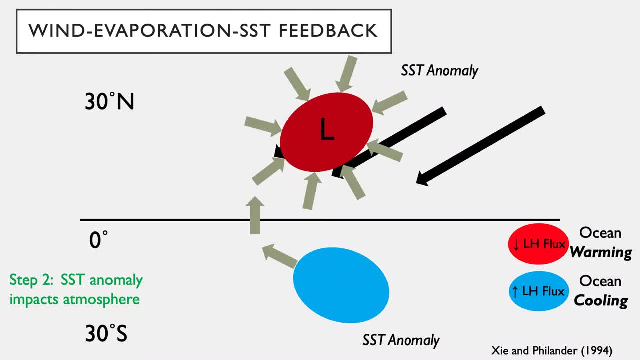 climate response to high-latitude forcing in the tropics. you can maintain a warmer Northern Hemisphere and a cooler Southern Hemisphere just through West's feedback, in a quasi-equilibrium sense, which is cool, If we can get to the Etten-Mip results. I'll show you some evidence of that. 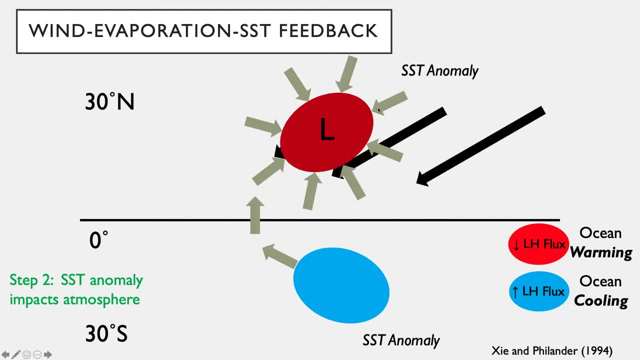 The second really important component of this is more of a transient response. This sort of drives the signal from the subtropics down onto the equator And the way that happens is we consider the effect of these surface wind anomalies On the mean flow after the SST field has grown big enough to impact the atmosphere. 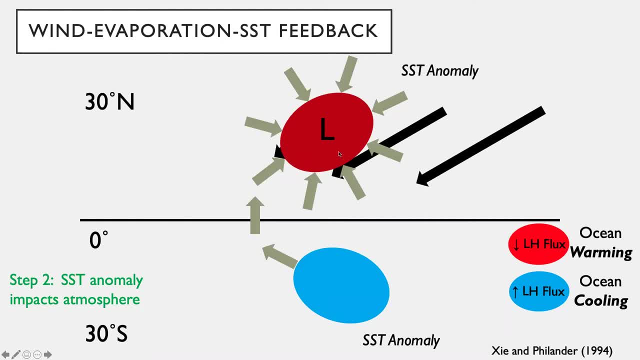 So what happens is that on the southwestern portion of this SST anomaly, these surface wind anomalies are preferentially going to weaken the trade winds, whereas on the northeastern portion you're actually preferentially strengthening the trade winds. So you end up with this sort of dipole of turbulent heat flux anomalies where you reinforce 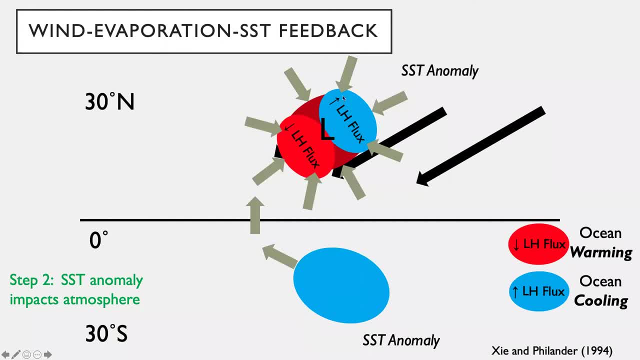 the warmest SSTs on the southwestern portion, but you cool them or you damp them on the northeastern portion, And so the net result is that the whole thing is going to propagate southwestward, And I don't know if I can toggle back. 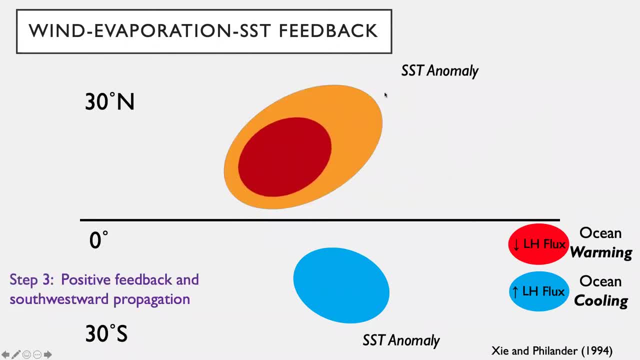 Yeah, let's see if I can toggle back. So this whole thing will just propagate southwestward and it'll sort of leave in its wake a dampened SST signal. So this is the transient teleconnection part that gets you that extra-tropical wind variability. 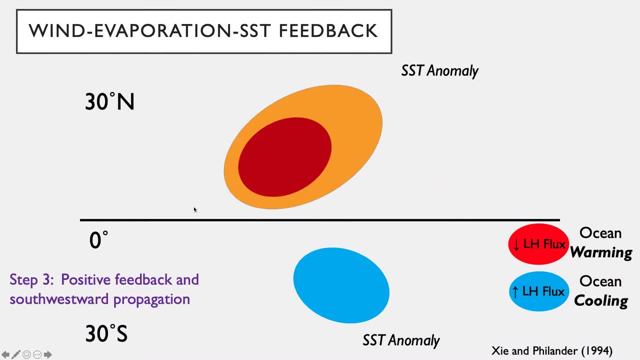 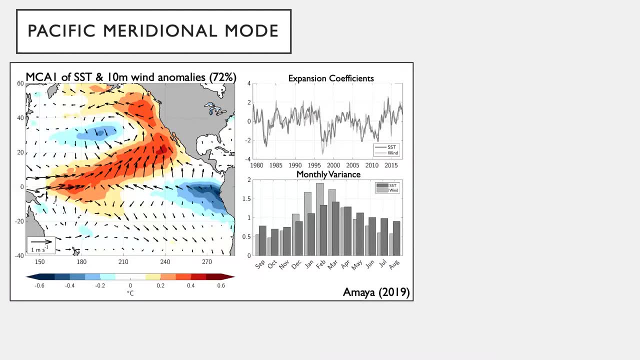 teleconnecting its footprint basically down into the deep tropics where it can influence all sorts of things. So you can quantify all of this using statistical methods. People often use these maximum covariance analyses. This is the first MCA of Pacific SSTs and surface winds. 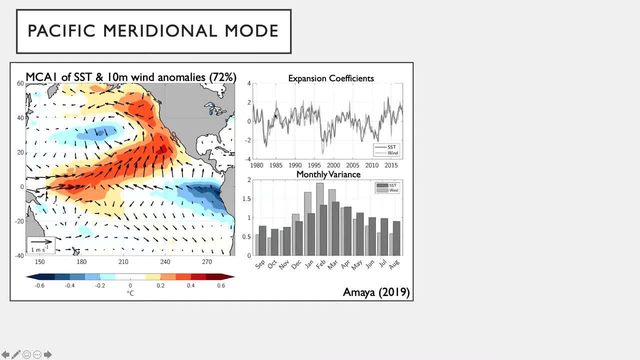 And you can see that the time series that explain this variability have all sorts of timescales involved. There's seasonal, inter-annual are the primary timescales, but the CATL is also important. People have argued that the CATL variability is also important here. 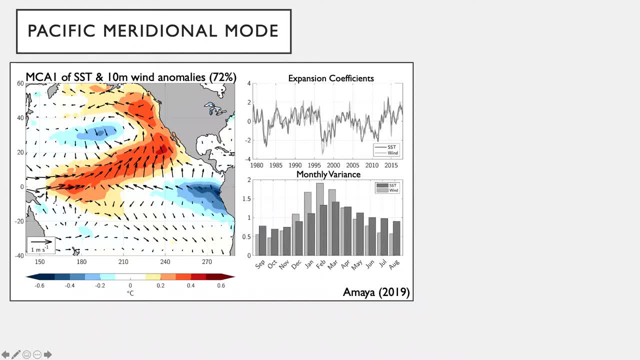 But what makes the PMM in particular really important is that it's not just about the weather. The PMM in particular really interesting is that it drives this wind variability around the dateline, So you would think that it could be potentially important for driving El Niño or La Niña. 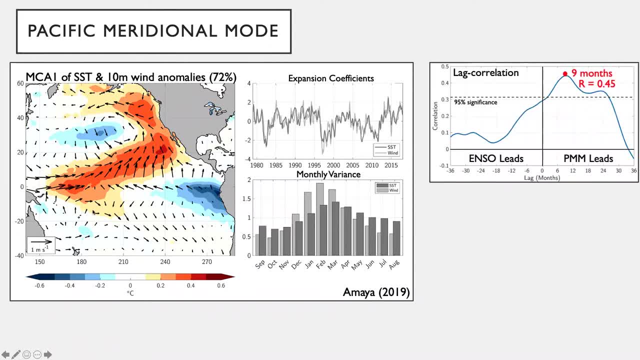 variability sort of in the following year. And if you look at a lag correlation analysis between ENSO and the PMM, you can see that the maximum correlation is when the PMM is leading by about nine months. So that holds The idea that if you generate a PMM in, say, the winter of year one, the PMM is going to 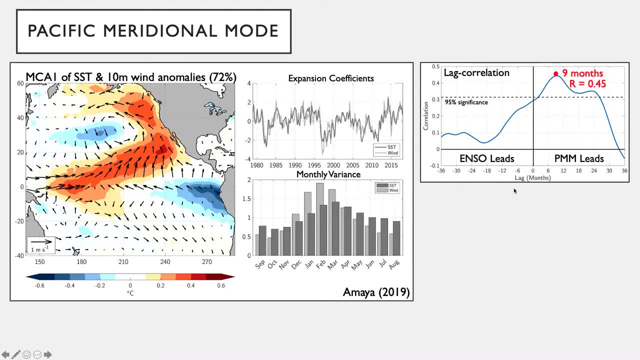 peak, say in the spring of that same year, And then in the following winter. you favor ENSO conditions in this case, And so this is really exciting. This is a really interesting and useful tool that we are hoping to leverage, because if 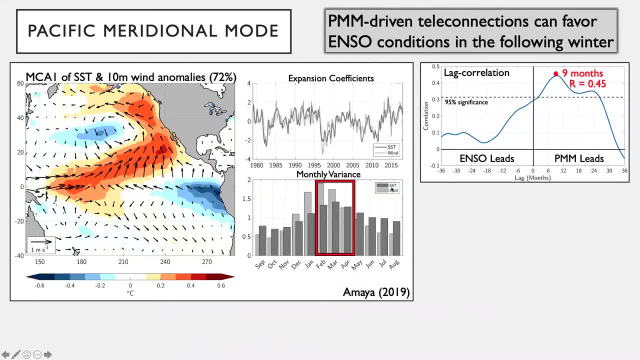 we think about when the PMM is peaking, it's peaking in the spring. If we look at sort of the monthly variance of SST in the time series, it peaks in the springtime And historically, if we look at models and the way that they can predict ENSO, this is. 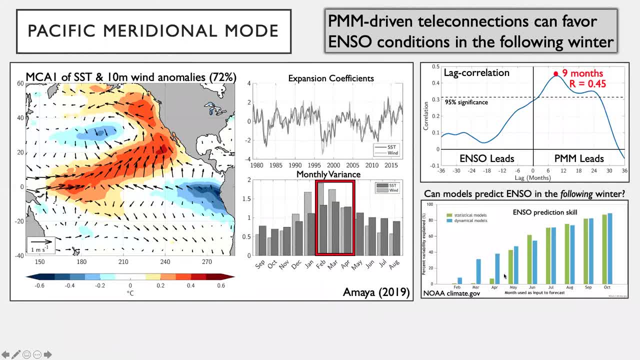 just sort of a metric for different statistical or dynamical models and their ability to predict, forecast ENSO at different leads. we don't have great skill during the springtime, right This idea of the spring predictability barrier, And so if we can leverage, if we can improve our understanding of the PMM-ENSO relationship. 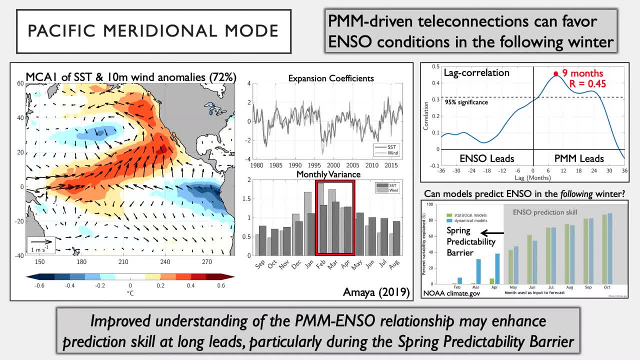 during this time of the year. potentially it can enhance our prediction skill of these long leads, particularly during the spring predictability barrier, And so I sort of I want to talk this up because I do think it's important, but I also want 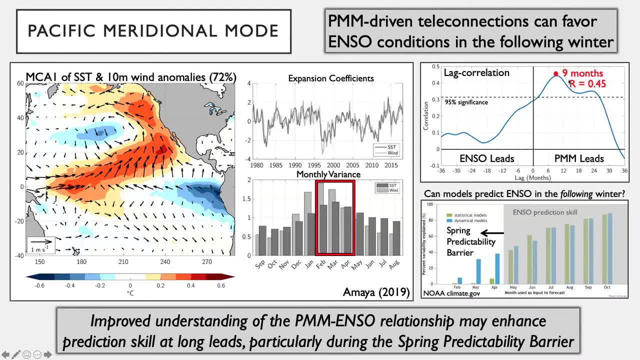 to keep context, that if we're looking at sort of the statistical relationship between the statistical relationship and observations, it's still it's not a first order process, right, The PMM's influence on ENSO is not a first order control on ENSO variability, but it 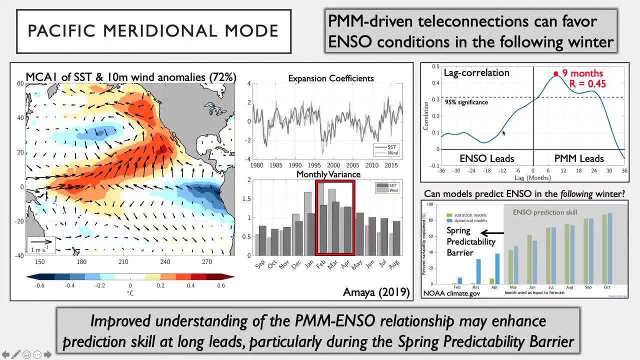 is important. This correlation is significant and it's just adding more and more, more and more useful tools that we might be able to use to improve our predictability of ENSO. So the goal as part of my research for my PhD was to quantify the importance of we 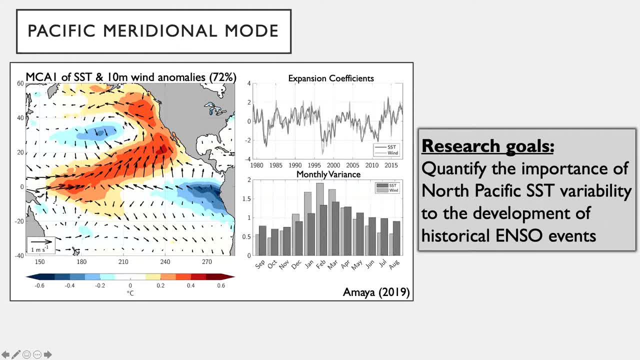 say, North Pacific SST variability, And what we're ultimately going to do is look at North Pacific SST variability, But keep in mind that in the subtropical North Pacific most of that SST variability is driven by these changes in the wind. So really we're trying to isolate the extra tropical wind forcing on the SST field by 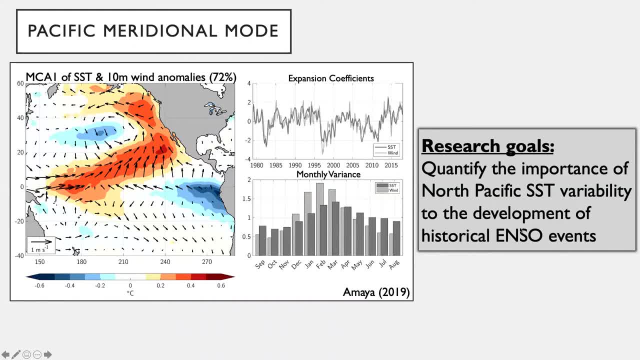 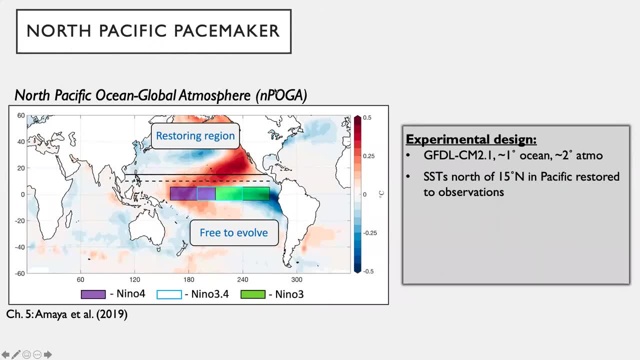 forcing our models with that SST field, basically. So the way that we're going to do that is by running a North Pacific pacemaker experiment, which we call NPOGA here, North Pacific Ocean, Global Atmosphere, And basically what we do is we take GFDL, seam 2.1, it's a one degree ocean, a two degree. 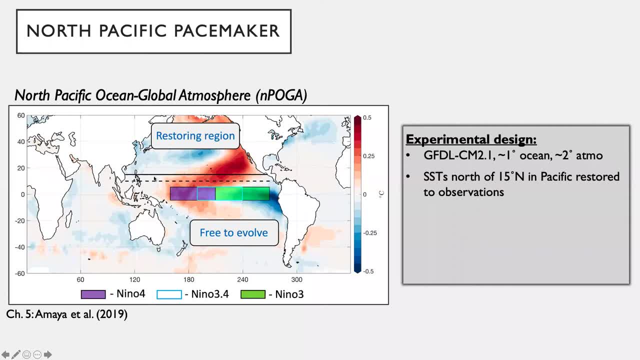 atmosphere and we heavily restore SSTs north of this black line, about 15 degrees north, And we restore them back to observations, whereas everywhere else in the model is completely free to evolve and do whatever it wants And it has a fully dynamical ocean. it can do whatever it wants. 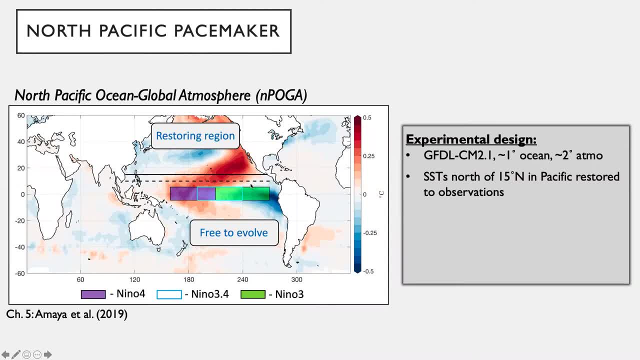 These pacemaker experiments have been used in a variety of different contexts in, say, the North Atlantic and also in the tropics, but this one here is just for the North Pacific. Okay, So the way we can picture this is if we just take a point within our box and we compare. 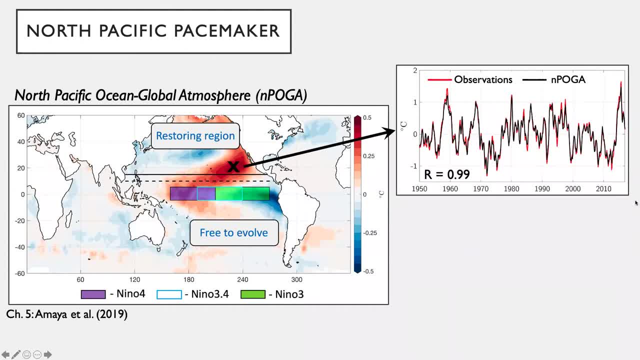 the model to observations over time, then they're basically the same thing. So this just shows that the restoration is working, whereas if you take a point outside the box, that is, in a region where you don't think the North Pacific is important for its 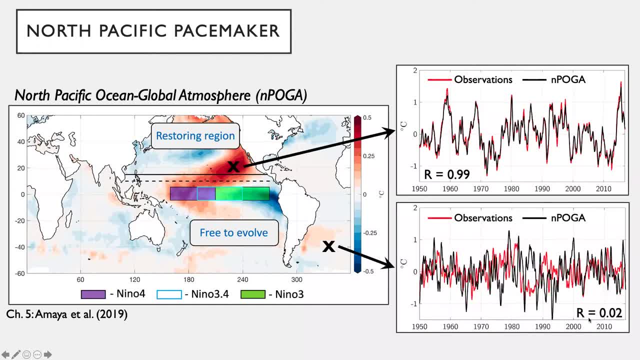 variability. you wouldn't expect them to be correlated at all And in this case they're not. So if we do this enough times, in this case we're going to do 10 ensemble members from 1950 to 2016.. 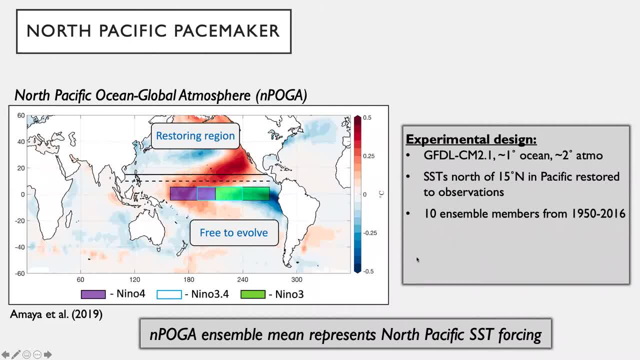 The ensemble mean will hopefully cancel all of the random internal variability between these ensemble members. assuming we have enough to span sort of the breadth of internal variability, Then the ensemble mean should represent North Pacific SST forcing on the climate system, And the goal is to see how well we can reproduce the real world just given information about. 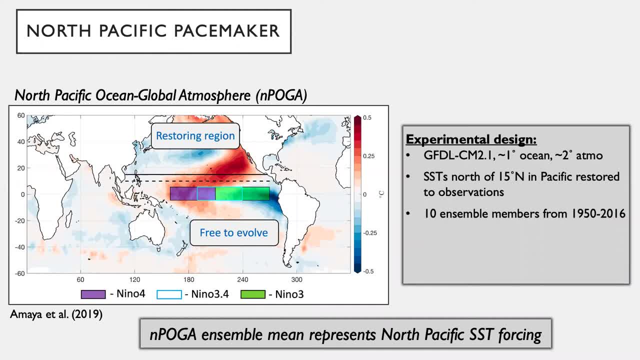 the real world in the North Pacific, Sort of importantly also to sort of isolate the impact of some of these observations, the impact of sort of local SSTs outside of our box, on the wind field we need to compare to an atmospheric only simulation where we don't have an ocean, to sort of couple back. 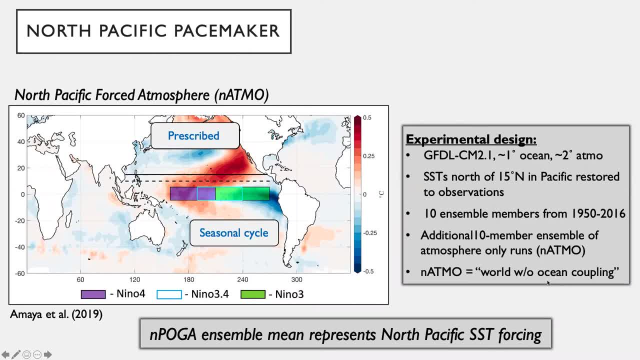 to our wind field. So the way that we do that is, we run an additional 10 member ensemble of atmosphere only runs where we just take an atmospheric model- in this case GFDL AM 2.1, and we force the exact. 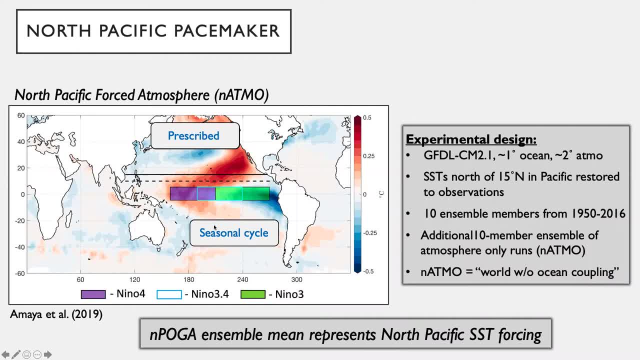 same SSTs in the same domain in the North Pacific, whereas everywhere else is a seasonal cycle. So if we get any wind variability outside of our box, it's due to the winds that we prescribe within our box. And if we compare the winds between the coupled run and the uncoupled run, we can get a sense. 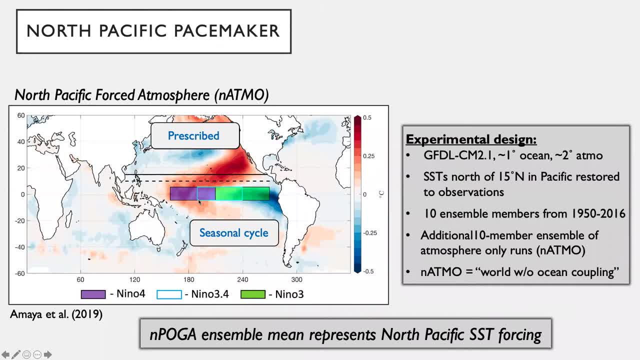 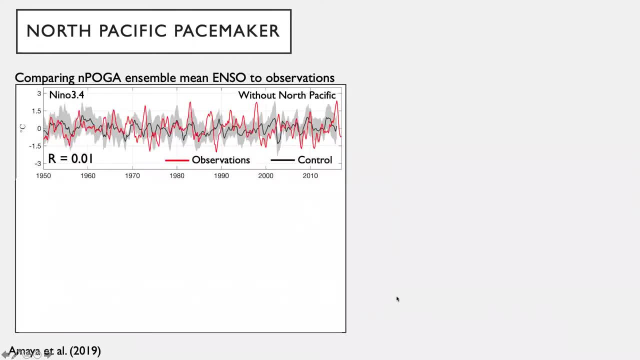 of how important things like air-sea feedbacks are within the tropics, things like WES feedback, Bjerkne's feedback, these sorts of things, All right. So just jumping right into the results here. The goal again is just to see right off: how well can we reproduce observed information? 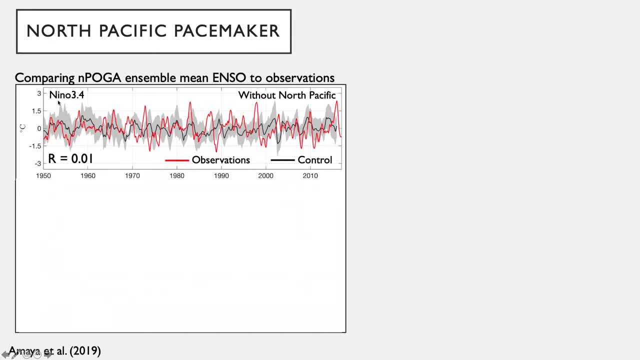 from the North Pacific. So this is the red line. here is observations. This is the NENIA 3.4 index. The black is a control simulation that we've ran that has no information about the real world whatsoever And obviously it's not correlated to the real world at all. 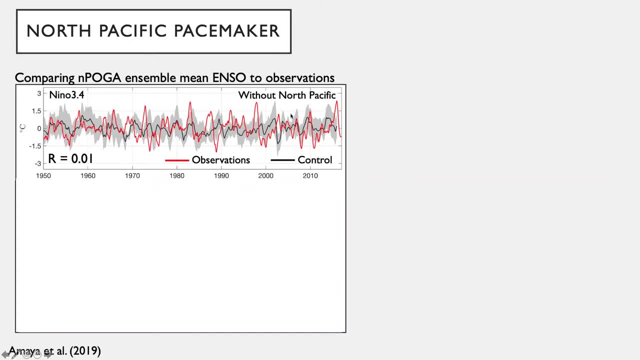 And the question is: when we provide information from the North Pacific, how well do we get back the real world? In this case, this is the world with, in the ensemble mean of our pacemaker simulation, You can see that our correlation goes up to about 0.3, which is about 0.1. 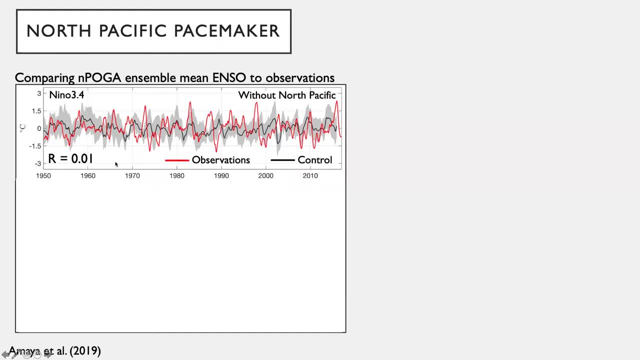 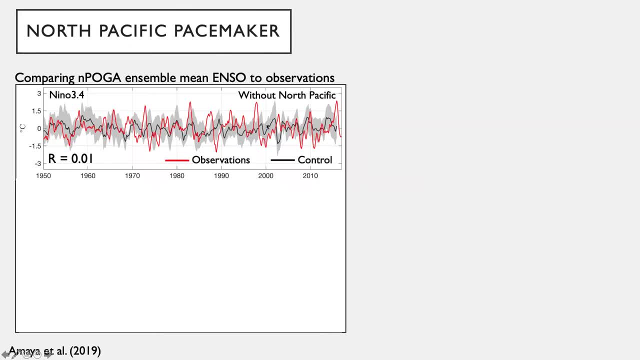 And then we have the NENIA 3.4 index, And then we have the NENIA 3.4.. So, as you see here, this is the end of the memb观 analysis. You can see that we can take multiple statements that are related to the data and then we can come to a particular information piece just a little bit later. So if I present this as the overall through the just another sample here, then there is a very simple but what would be helpful for users to sc? pnept the解 González. 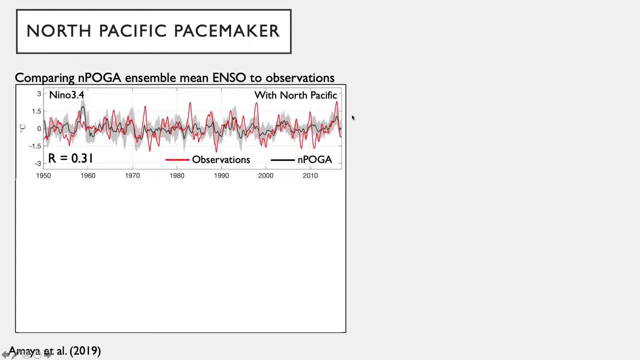 Mı, none at all. And the question is: when we provide information from the North Pacific, how well do we get back the real world? In this case, this is the world in the ensemble. mean of our pacemaker simulation, You can see that our correlation goes up to about 0.3, which again isn't super exciting. 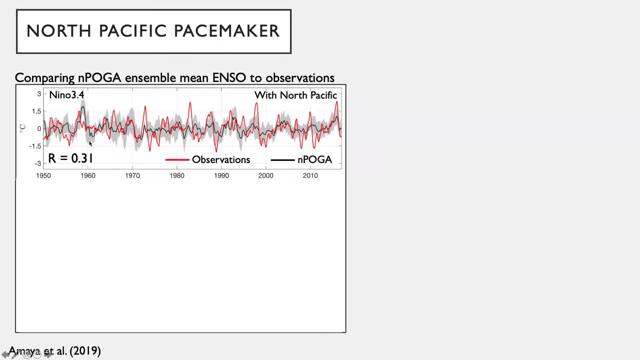 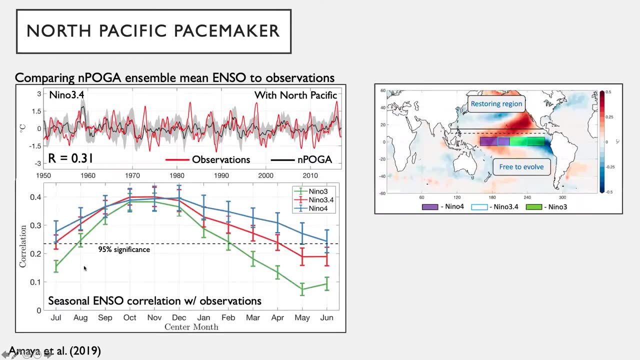 But I think there's a lot of neat information to sort of pull out here for a second. We can separate this, this variability, into seasons to see how well we're reproducing ENSO variability as a function of sort of lead time, and we can. 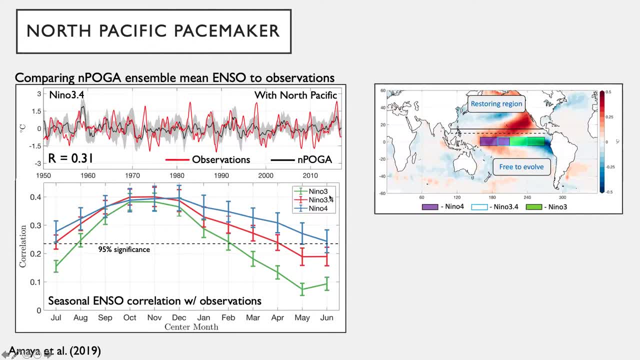 also look at different Nino indices to see if we have sort of a central versus eastern Pacific ENSO component here. Basically, what you'll see is that we significantly reproduce the real-world El Nino ENSO variability in the fall and in the winter time, with peak correlations of about 0.4 and sort of. 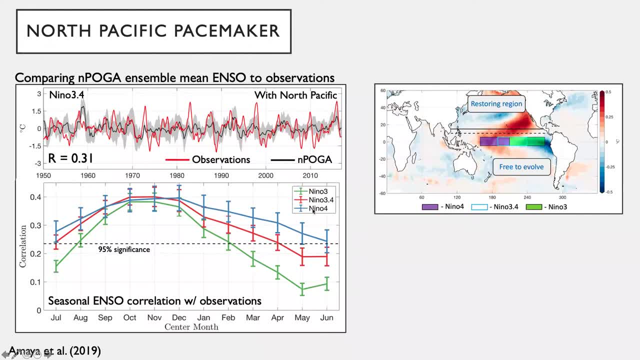 looking at the Nino 3 versus Nino 4 region, sort of eastern Pacific versus central Pacific, you can see that we get a lot more of the variability for a lot longer in the Nino 4 region. So that sort of speaks to maybe to some. 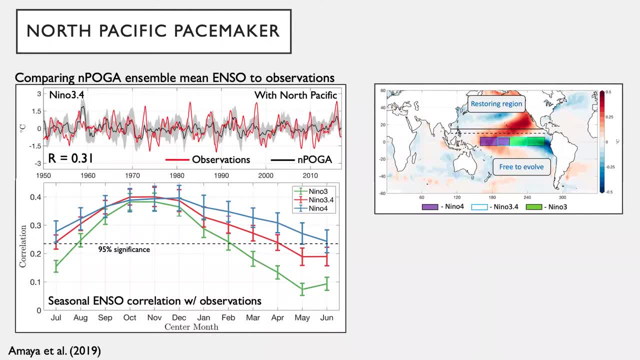 degree speaks to ENSO flavor preference for this sort of forcing. So we explained about 16% of the variance and I would argue that's actually right about where we would we had hoped to go If we go back and we look at our sort of lag. 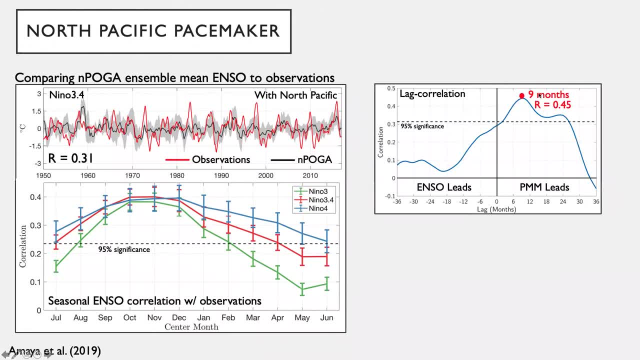 correlation in the real world, we can see that the Nino 3 versus Nino 4 region is about 0.4.. So if you look at the Nino 3 between the PMM and ENSO in the real world, 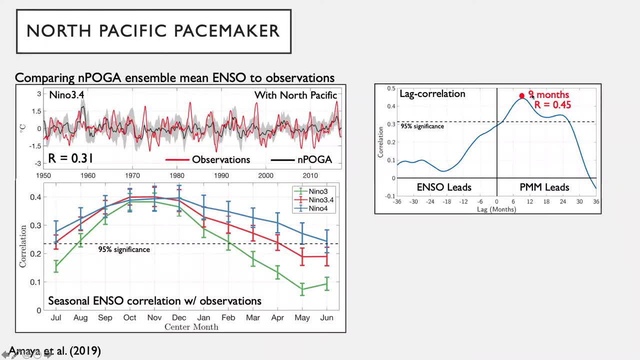 the correlation is about 0.45 for this nine month lead. So our simulations. we're never going to reproduce the world perfectly because, as I mentioned, this is not a first order process control on ENSO. Our goal was to be able to reproduce a correlation something much closer to this, about 0.45, and we're 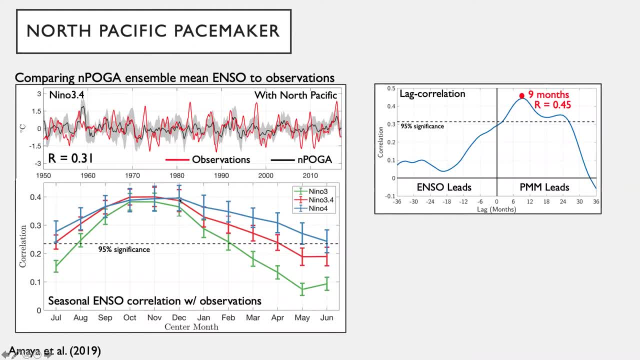 doing that here We get a correlation of about 0.4.. So I think our model simulations in this sort of lag sense are doing really well. So it seems clear that the coupled simulation has some skill at reproducing ENSO in Borea, fall and winter. So what evidence of these sort of 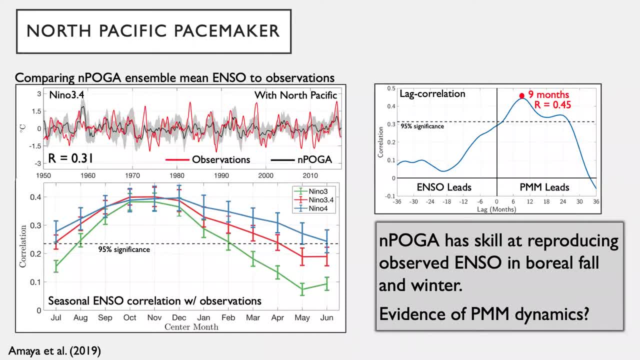 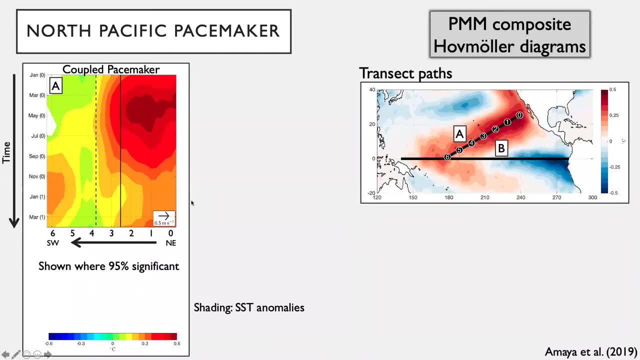 PMM dynamics. what evidence of WES feedback? do we have that sort of drive, that teleconnection to the lower latitudes? The way that we're going to look at that is through this Havmuller diagram. This is a, as I said, a Havmuller. 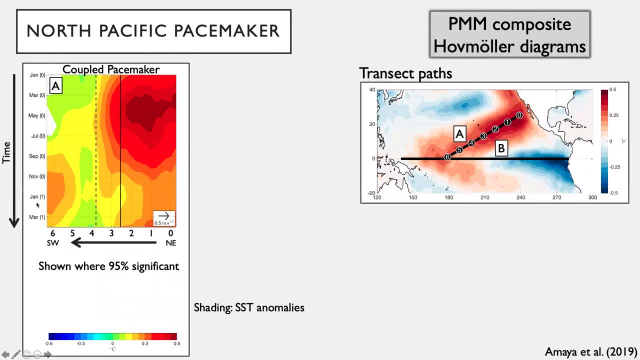 diagram that shows the evolution of an average PMM event in the coupled model, And so it evolves in time on the y-axis and it evolves in 2D space on the x-axis. So it's following this transect A here, So going from point zero to point six point. 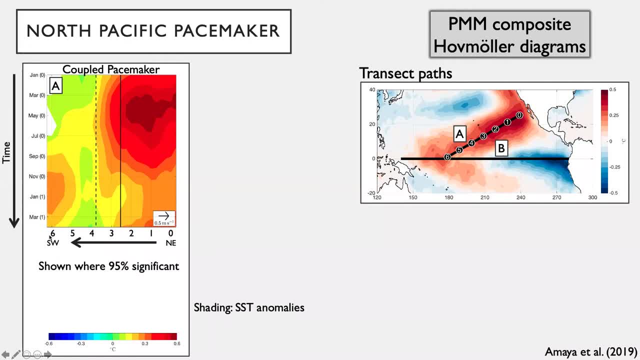 zero point six. we're going from the northeast to southwest. The model is restored in this- just to the right of this vertical black line here in the Northeastern Subtropical Pacific, It's completely free to evolve outside of this. this dashed line here and in between is a buffer zone. We have a 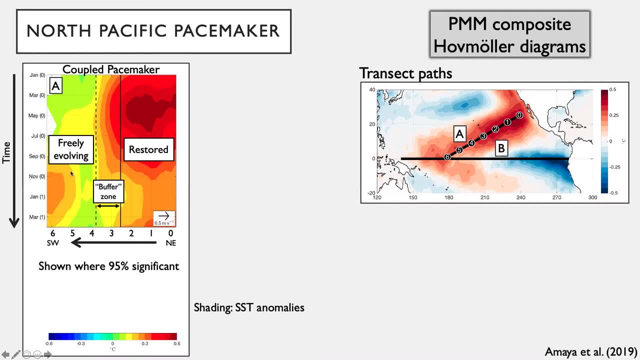 linear drop-off in our restoration rate. So the model is completely free to do whatever it wants over here and it's constrained- at least the SST is constrained- over here And again we're evolving in this northeast to southwest transect And this is the average I 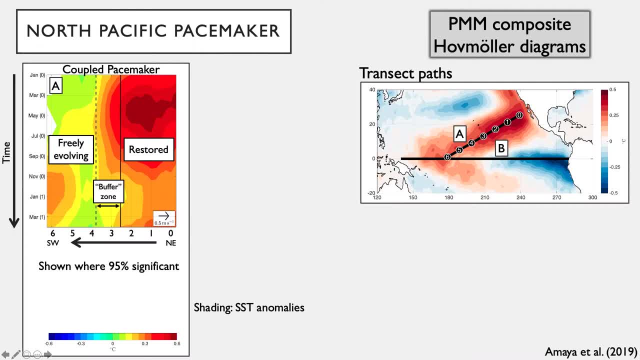 should mention. this is the average of 17 positive PMM events from 1950 to 2016 and this is across 10 members. So we have a hundred and seventy independent samples here. So this is SST that I've plotted here. I'm going to add zonal. 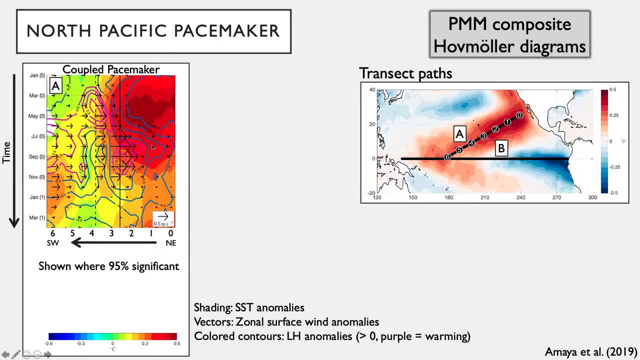 surface wind anomalies, and then I'm going to add latent heat flux anomalies on top of that as well. So the colored contours are latent heat flux anomalies and the purple is ocean warming in this case. So purple is a positive latent heat flux. So this is a pretty messy graph, but I am going to step through it pretty. 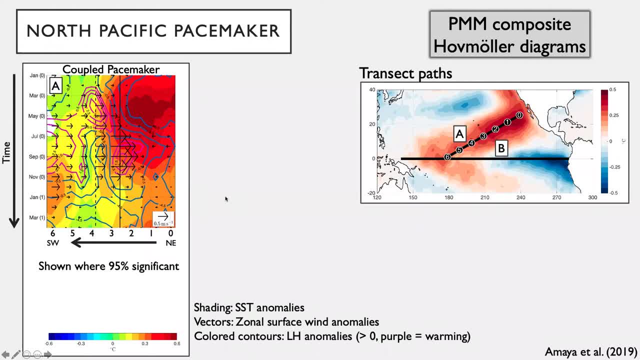 carefully and just sort of focus to you, what you should, what the most important features are. So, for one thing, if we look at the evolution, it peaks. the PMM in this case is peaking in the springtime in the sort of the subtropical North. 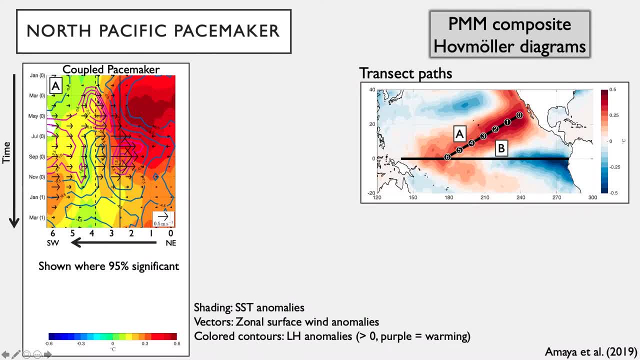 Pacific And about that time we can see the sort of this tongue of positive latent heat flux anomalies and westerly zonal wind anomalies and positive SSTs. These anomalies begin to extend outside of our restoration region and propagate in time southwestward down, closer to the equator, closer to that. 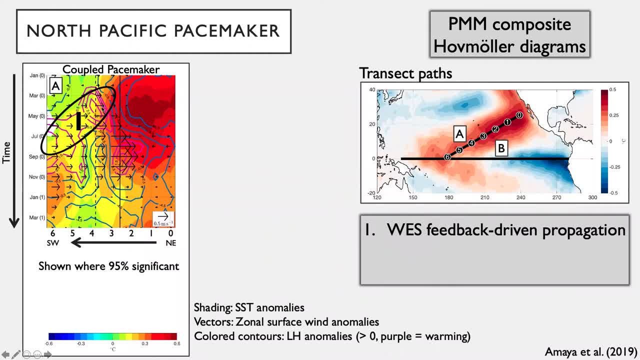 point six here right around the dateline, And this is: this is pretty indicative of WES driven propagation that I showed in that cartoon schematic earlier, This idea that if you weaken the trade winds you reduce evaporative cooling at the surface and you increase SSTs and that whole thing is going to propagate. 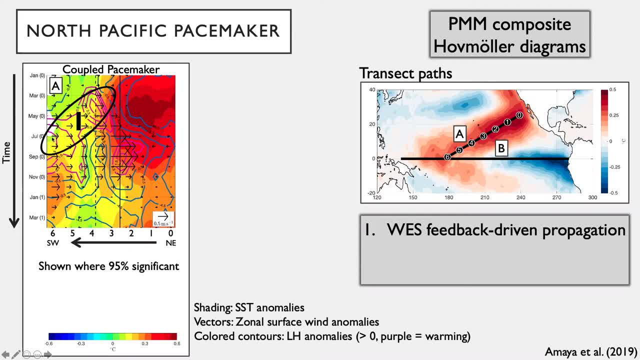 southwestward Eventually, once we get on the equator, these zonal wind anomalies I started to grow slightly and these SST anomalies definitely start to grow along the equator So we can look at more of an equatorial hoglular at this. 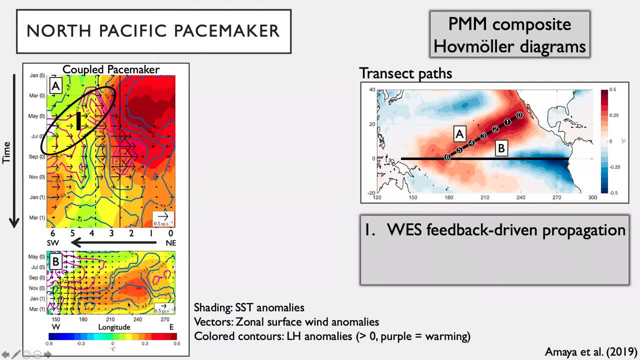 transect B. This is just going to be three south to three north average down here And we can watch the evolution of SSTs along the equator and surface wind And basically you can see is the is sort of the time evolution of a classic. 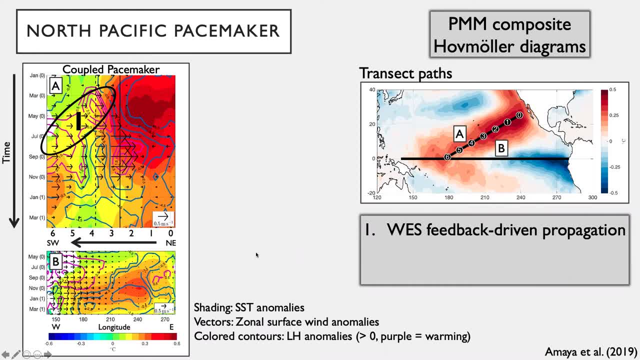 El Nino event, which which sort of indicates to me that Bjørkny's feedback is being kicked off here. So they say this: just by forcing this model a with information from the North Pacific, we're able to drive coupled interactions outside of our box. 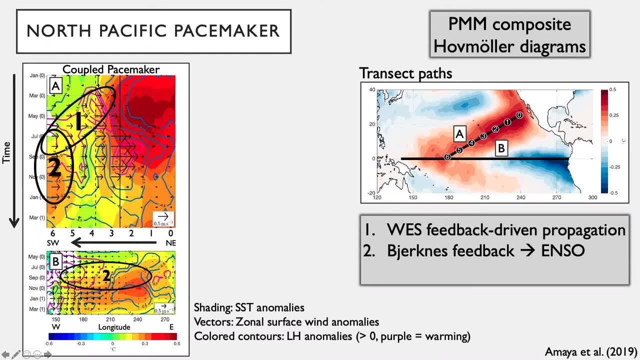 down to the equator where it can trigger ocean wave dynamics, flatten the thermocline in sort of the central eastern Pacific and drive El Nino variability- in this case an El Nino event. So that by itself I think is really neat. And then sort of the third thing to focus on is sort 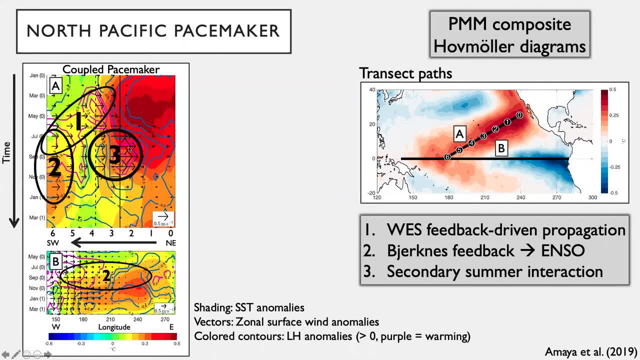 of this resurgence, the secondary summertime interaction, where you get a resurgence in the wind field, And we'll talk about that in more detail here in a second. But, as I mentioned, it's important to compare to the uncoupled run, because then we can say whether the wind 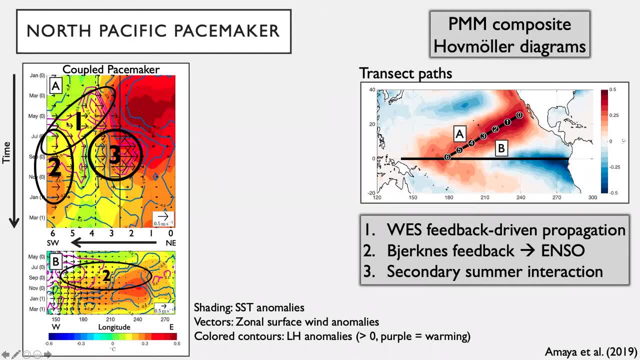 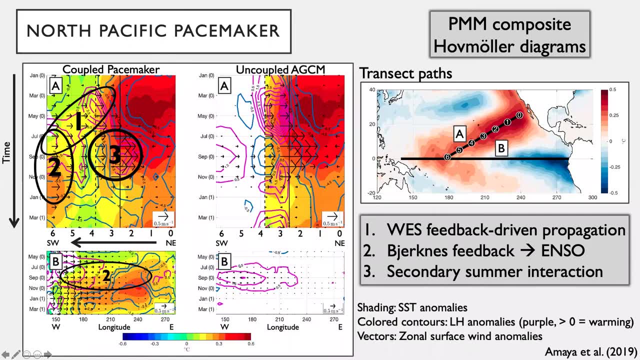 variability outside of our box is due to coupled feedbacks, or maybe it's just a downwind response to having prescribed warm SSTs, basically. So here's the uncoupled AGCM run: same Hopmuller, same contours and everything, And basically what you can see is that in this one region 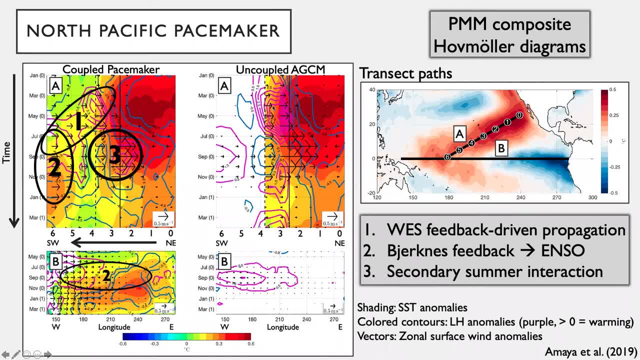 where I'm claiming we have WES feedback-driven propagation, the model does not reproduce these winds at all. So what that says is that the winds in the coupled run are completely due to local SSTs. So that basically confirms that WES feedback is happening here in the springtime. But what is? 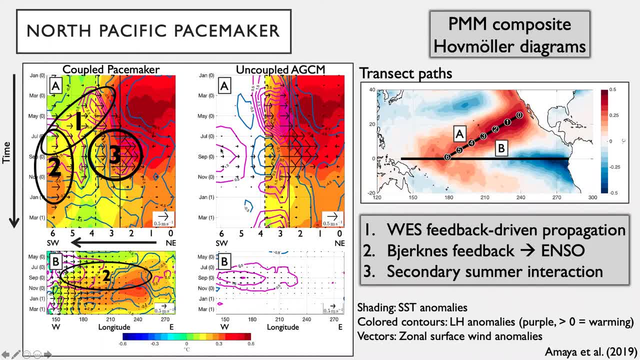 really interesting is that during the fall time- late summer, early fall- you get a. you do get sort of an uncoupled- I say that loosely uncoupled- from the local SST wind response very near to the equator. 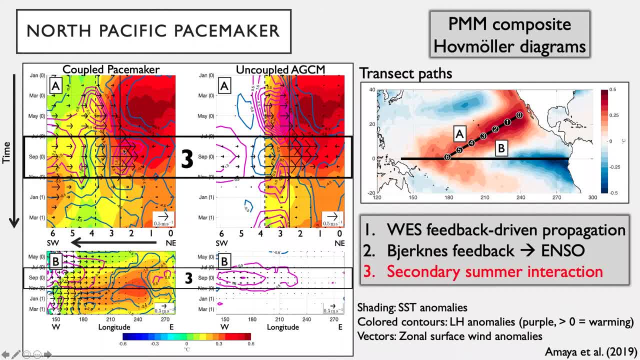 And it happens during this sort of secondary summer resurgence of the wind field downstream. So it says that on the equator at least, some of the wind variability is due to SSTs from the subtropical North Pacific. So let's analyze this in a little bit more detail. I'm going to focus. 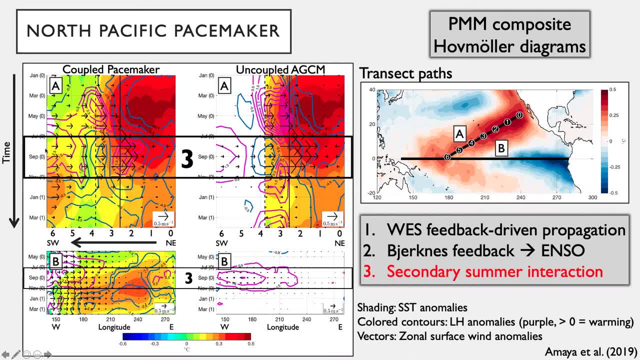 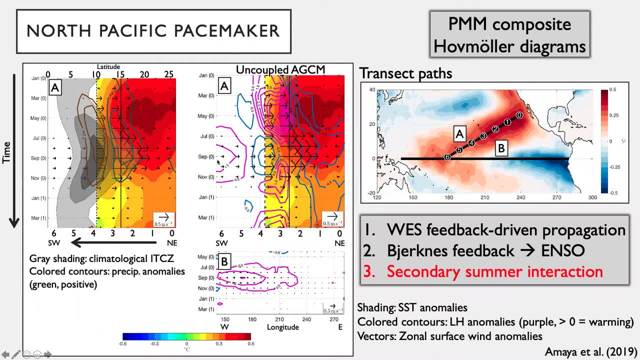 in sort of a 2D sense. I'm going to focus on just August through AOS, So August through September in this box, and we're going to look at XY space. Oh, just sorry. one more thing. Why is this happening? 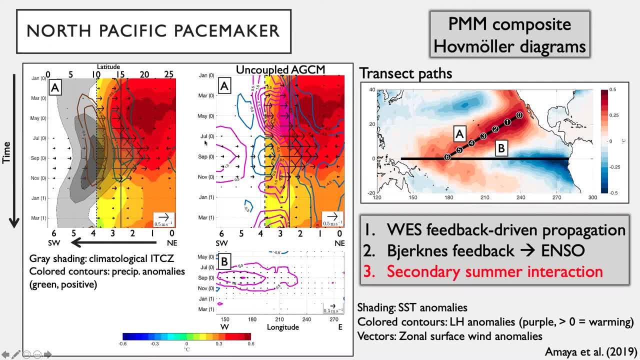 We can look at precipitation to get sort of an idea of what's going on here as well. This is the uncoupled run, and the colored contours here are precipitation anomalies. The gray shading is the zonal mean climatological ITCV, and this could just give us some hint as to 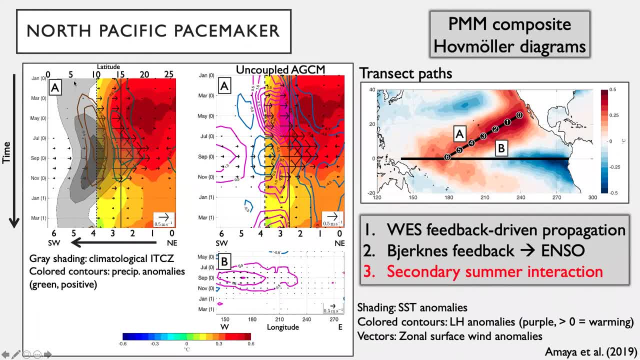 what's going on here in the uncoupled run? Basically, what's happening, I think, here is that during the winter time, when the ITCV is as far south as it's going to be, it's not particularly sensitive to these off-equatorial SST anomalies. 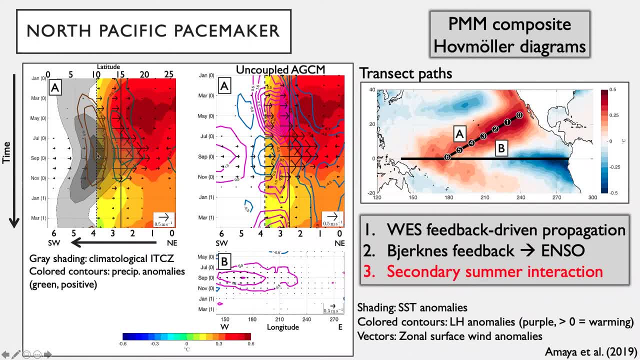 But as it migrates further northward, say in the late summertime, early fall, it becomes much more sensitive to these warm SSTs and you can see through the precipitation anomalies you get this northward shift in the ITCV that corresponds with sort of this downstream surface wind response near. 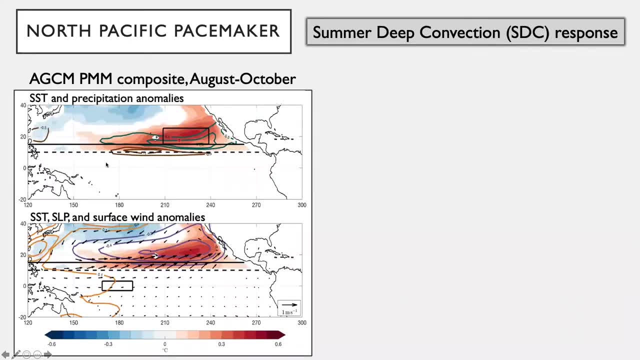 the equator. So now let's look at this in 2D space and get a better sense of what's going on. This is again August through October, so ASO, excuse me, This is the uncoupled run. so this is where we restore SSTs and everything else out there. 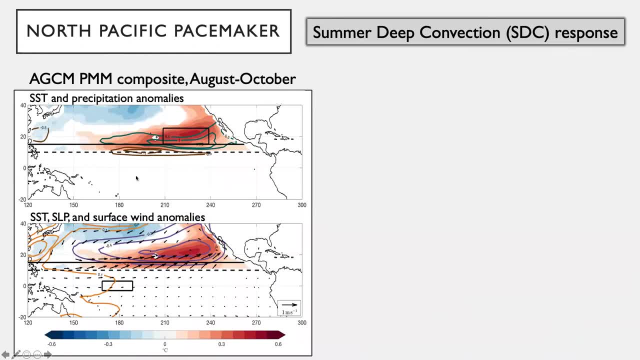 This is the uncoupled run. so this is where we restore SSTs and everything else out there. As you can see, outside the box, there is no. there are no SST anomalies, which is why it's white Colored contours. here are precipitation anomalies. You can see that northward shift in the ITCV. 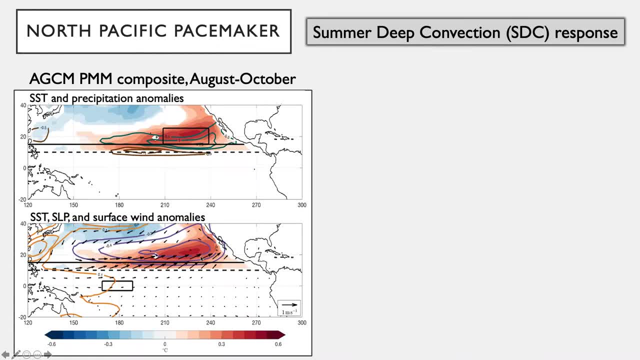 In response to the enhanced convection in the off-equatorial region, you get upper-level heating which gives you- you end up getting a gill solution to an off-equatorial heat source, basically. So you get this large cyclonic circulation response to that increased heating at height. 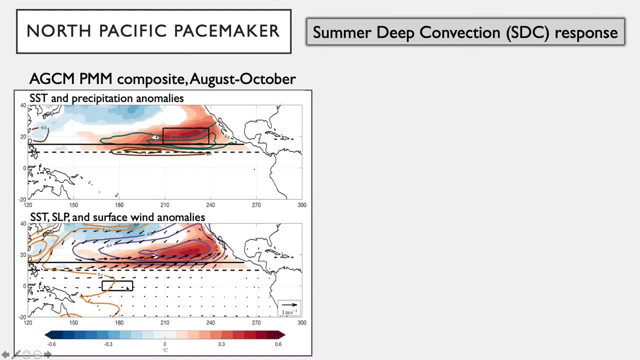 And that large circulation equator driving wind variability on the equator. So at least some of this variability in the real world and in the coupled model is driven just by sort of subtropical, warm North Pacific SSTs. And I should keep, I should mention that again. this is happening in a model where there's nothing. 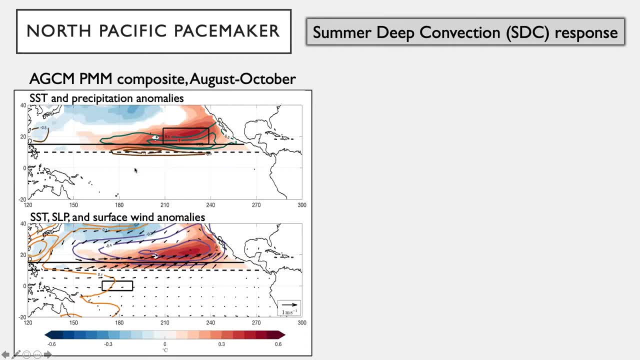 competing with it in the tropics. If you have really strong warm anomalies along the tropics, the ITCC doesn't want to shift as much, because you have sort of a tug of war. what's going to win? So this, that is one sort of caveat to all of this. In the model, though, you can see how well 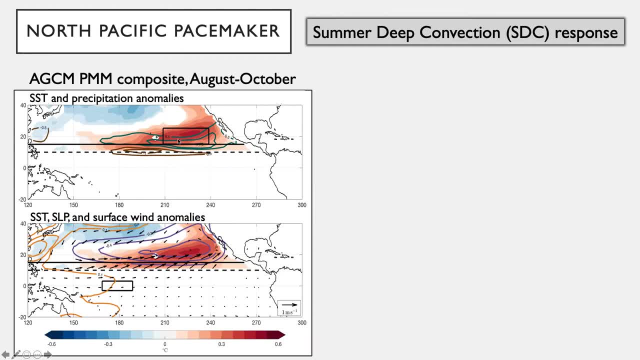 how much this is going to drive wind variability by comparing SST anomalies averaged in the subtropical box, comparing it to zonal wind anomalies averaged around the dateline where westerly wind events are thought to be important for ocean kelvin wave generation and, ultimately, 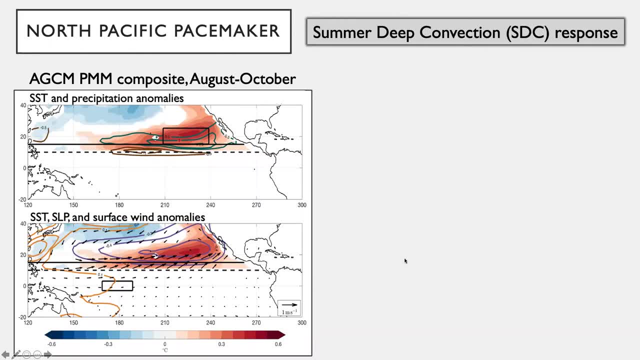 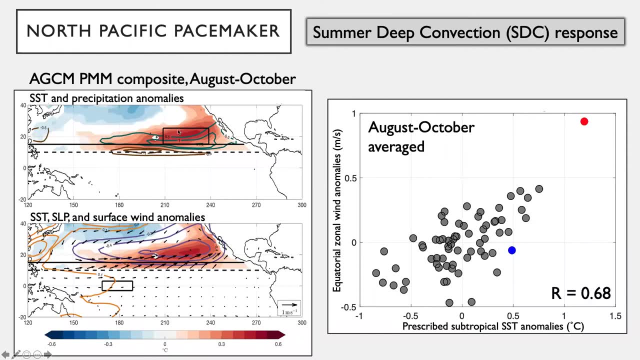 ENSO dynamics. That's here. hopefully, there we go. Basically, you can see that in the model these things are obviously positive. You can see that in the model these things are obviously positive. They've correlated that the warmer you have the stronger, the warmer you have subtropical SSTs. 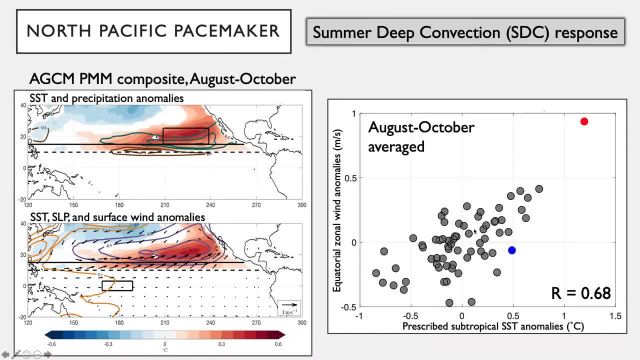 the stronger the zonal wind anomaly along the equator. And I do want to point out one particular value here. This one way up here, this is 2015, when the PMM was the largest it had ever been on record. The 2015 PMM was huge. What's interesting about this point is that, if we go 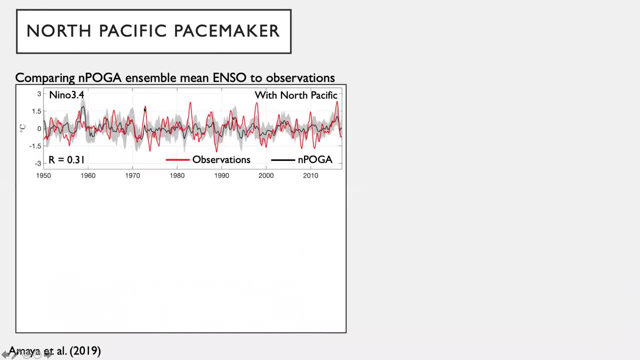 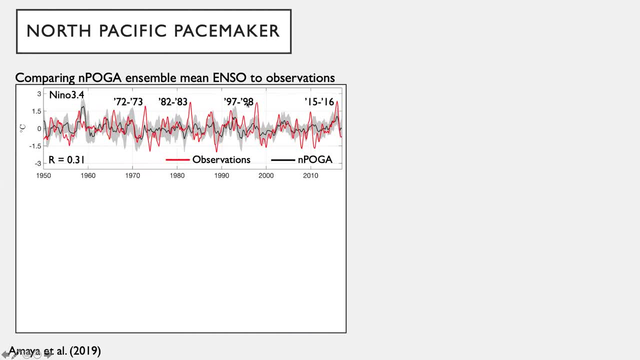 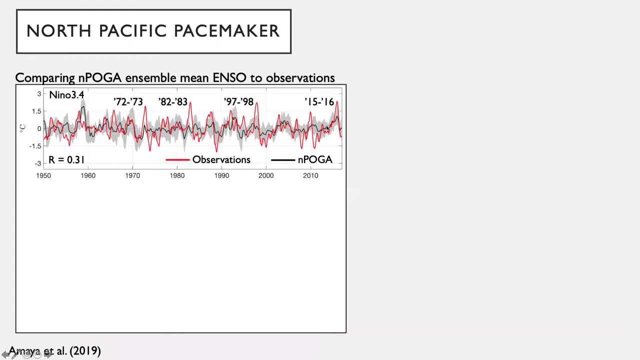 73,, 82,, 83, or 97,, 98,, but our model does a very nice job of capturing sort of the timing and relative magnitude of this weak 2014-15 El Niño, as well as the extreme 2015-2016 El Niño. So we 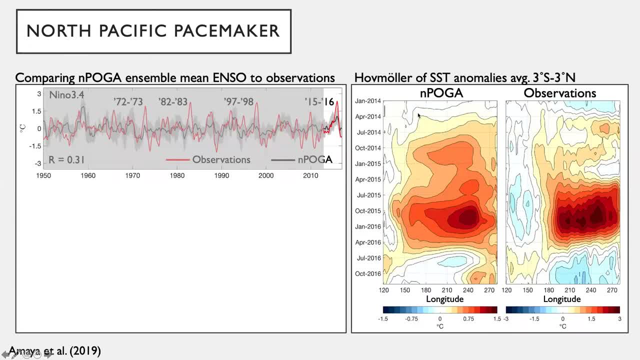 can look at that in Hofmuller space just to get a sense of what's going on. This is a coupled run. This is a coupled run- Three south to three north. SSD Hofmuller and this is in observations, So we can see that we get the timing, onset and relative magnitude of the 2014-15 El Niño. 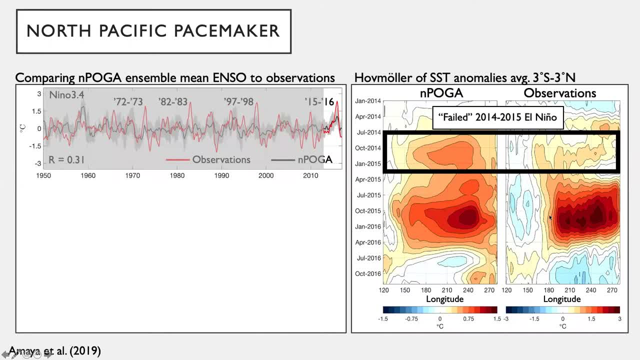 So we can see that we get the timing onset and relative magnitude of the 2014-15 El Niño And then again the timing relative magnitude and actually, to some extent, the termination and transition to a weak La Niña here for the 2015-2016 El Niño. So why is this? Why is the 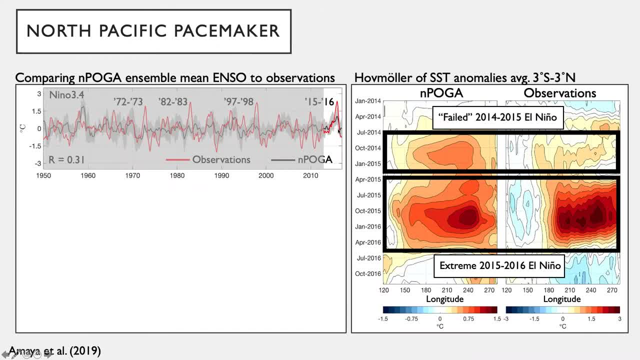 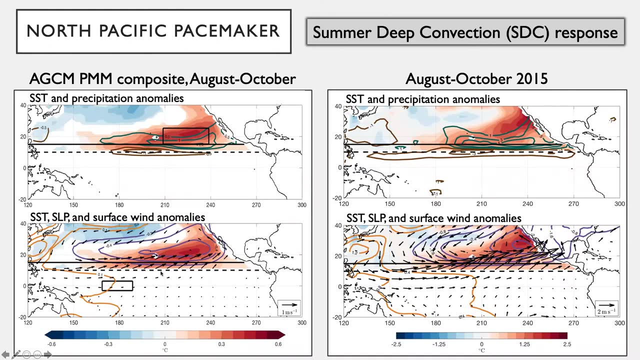 model doing particularly well with this particular El Niño event. Part of the reason is because of part of the reason is because of how strong the, How strong the PMM it was during that, during that preceding spring, so during that spring of 2015. if we look at our, this is just our composites again of the PMMs impact on. 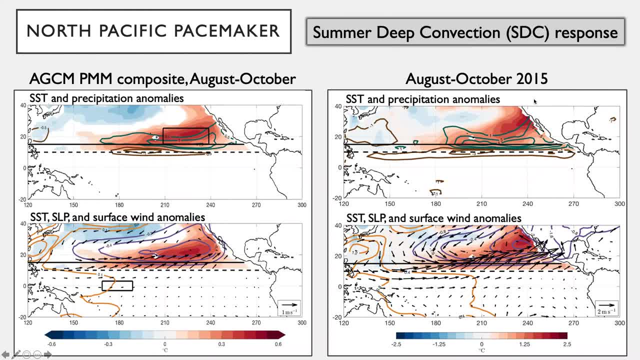 the late summertime atmosphere, and this is comparing it just for 2015. it basically looks like an enhanced version composite, and for what it's worth. I should mention that the composite doesn't really change if you remove this event, so the composite is not overly weighted by this particular event, but 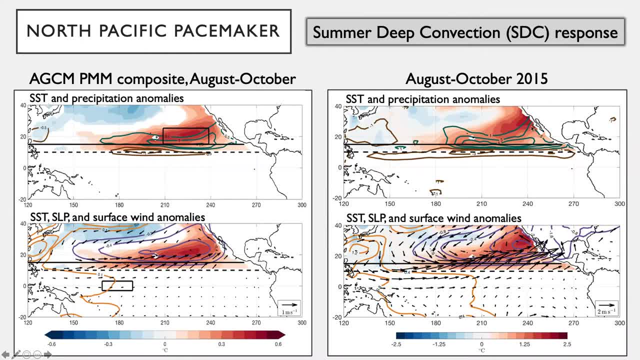 the point I want to make here is that the 2015 event was massive. the subtropical anomalies were something like two, two to half degrees above normal, and this, this would have driven a large sort of downstream atmospheric response that projects on the equator. it would have triggered. it triggered, I would have. 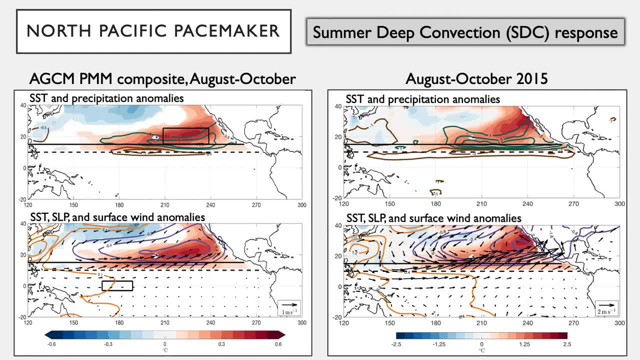 it would have sort of pushed the distribution of random westerly wind events towards El Nino favorable, and that's sort of what. that's what that's. the goal of these PMMs, so to speak, is to enhance, sort of load the dice in an instance of the climate change, and then we can see that it's a little bit more. 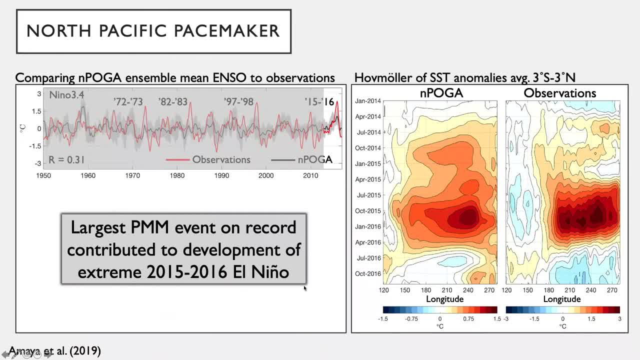 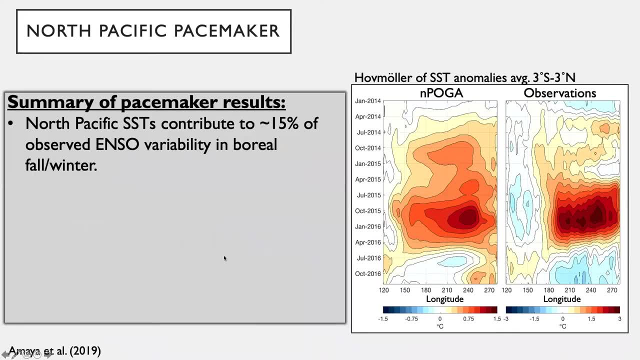 in favor. so again, the largest team of the record contributed- almost certainly contributed- the development of this extreme 2015 2016 El Nino. so I'd like to summarize these pacemaker results: North Pacific SSTs contribute to about 15% of observed ENSO variability in boreal fall and winter. and going back to thinking, 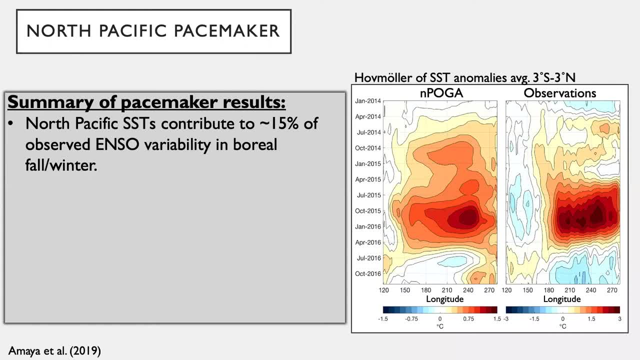 about these regional mechanisms for extra tropical tropical interactions. in this case we're not as concerned about how do high latitude energy or temperature perturbations get to the deep tropics we're interested in how does, how does extra tropical atmospheric variability imprint on sort of the subtropics and then make its way to the 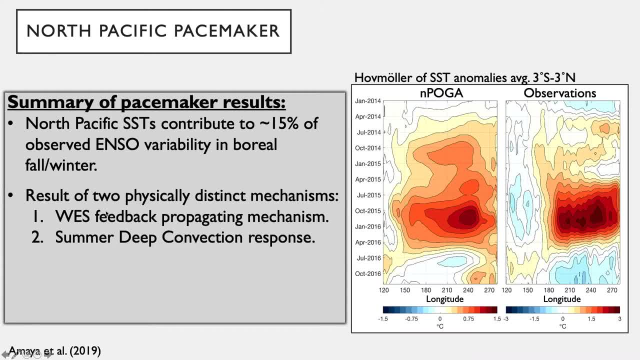 deep tropics where it can influence climate, things like ENSO- and it does that primarily through two physically distinct mechanisms. one is this west feedback propagation and the second we're calling this summer deep convection response, this potential for the ITCZ to shift northward due to 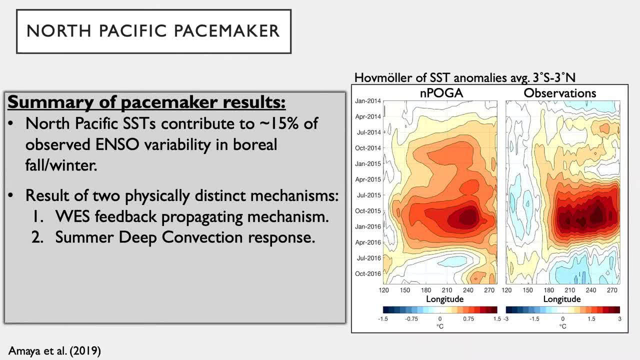 warmer, a warmer subtropical North Pacific, and this happens in the summertime, because that's when the ITCZ is closest to the subtropical and the subtropics and I should say boreal summertime, and it can drive as sort of a downstream, locally uncoupled wind response that enhances the likelihood of 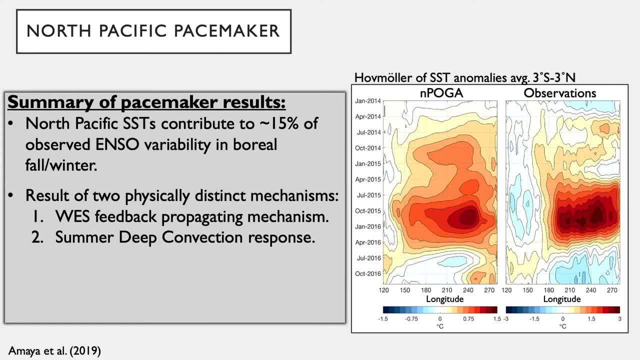 westerly wind events around the dateline. and again, if we think about individual events, the extreme 2015 1619 El Nino was preceded by the largest PMM on record, which contributed to its development. so for this, the last 10-15 minutes were preseeded by the largest PMM on record, which contributed to its development. so for the last 10-15 minutes, 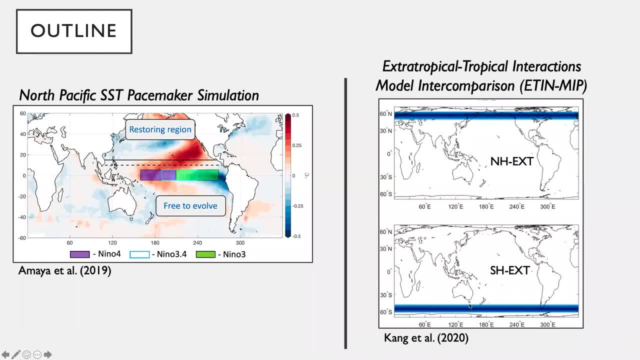 the presentation today I'd like to show some extremely preliminary results from an analysis I'm doing of this extra-tropical-tropical interactions model in an inter-comparison project, this ETENMIP, which is an amazing resource for the community to look at sort of these regional mechanisms in detail. It was 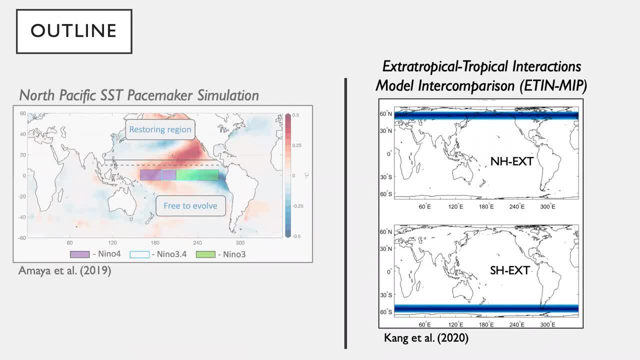 spearheaded by Sarah Kong, who's at UNIST in South Korea, as well as a vast array of great scientists from all over the world, So this is a really great data set. I can't sing its praises more, and I'm really looking forward to singing. 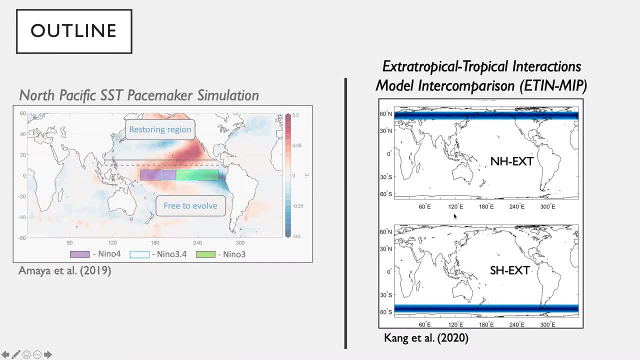 my teeth into it more. But I do want to treat sort of these next results as sort of more of like a group meeting, because I'm sort of interpreting them, not necessarily on the fly. I've looked at these a lot but I would be more than 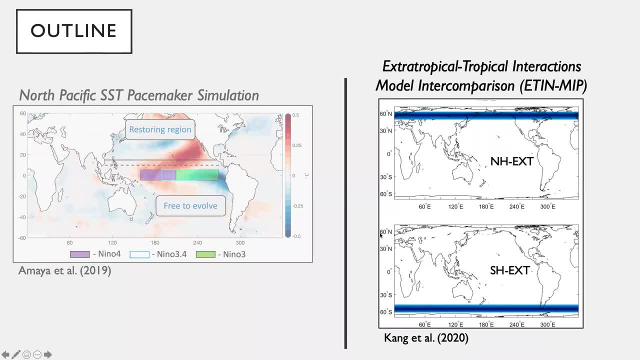 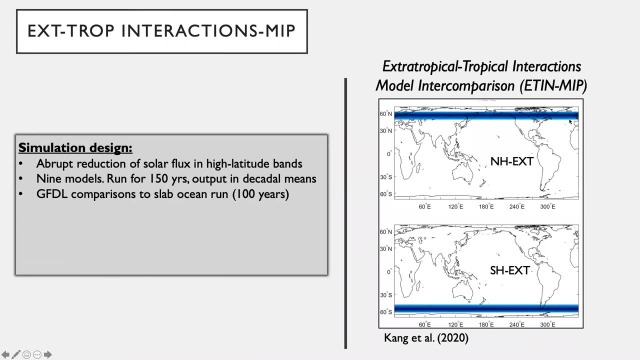 happy to hear people's suggestions and observations as we go through this a little bit further. So just to give you some context about what is going on in ETENMIP: it is a MIP, so it's a protocol for a variety of models to follow There. 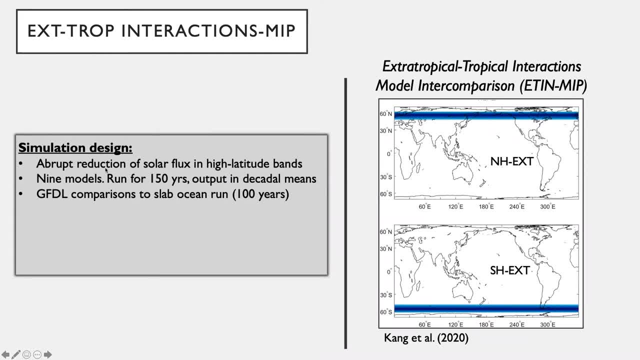 are nine models and what they do is they abruptly reduce top of the atmosphere solar insulation and high-latitude bands- and these are those bands in the Northern Hemisphere and the Southern Hemisphere- and they just hold that fixed and they run the model for 150 years. It's a coupled model, so 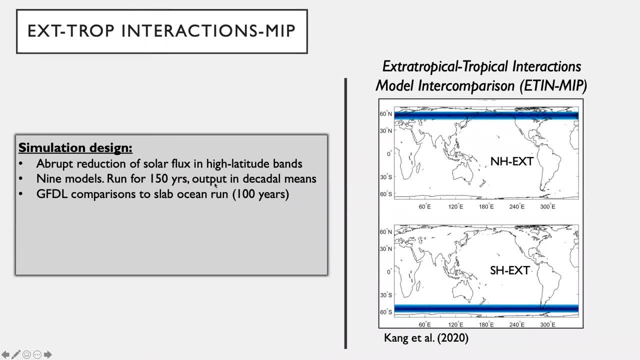 there's a fully dynamical ocean and they output into cato means, which is a bit of a headache, but I'm working on getting the first 20 years of data for a variety of reasons, And then we can also compare the dynamical ocean. 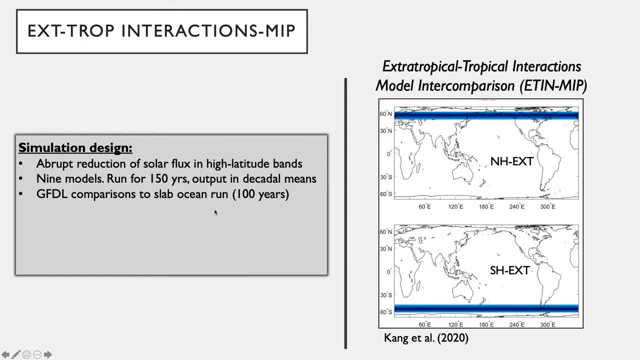 runs to a slab ocean run to sort of diagnose air-sea interactions. but there's only one model that did a slab ocean run and they did it for a hundred years and that was GFDL. So the goals of analyzing ETENMIP here are: 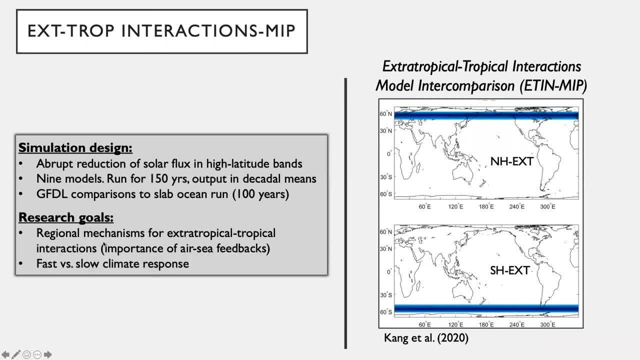 to well, I want it to load. there we go. the goals are to again look at regional mechanisms and sort of in a more general way, and then we can look at the generalised or maybe more idealised framework of extra-tropical-tropical. 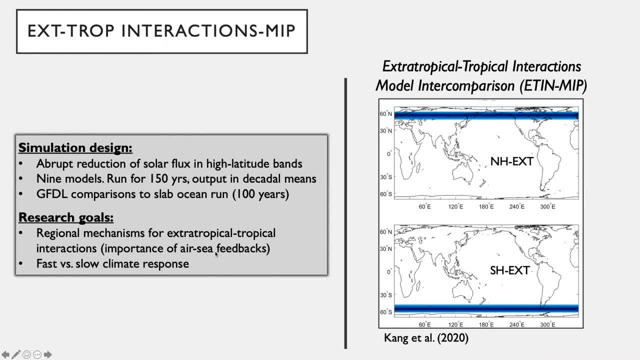 interactions and also assess the importance of regional air-sea feedbacks in driving these signals around. And then another goal, because we have sort of a longer time series of what's going on here. I'd also like to look at sort of the fast versus slow climate response. So how does the atmosphere adjust? very 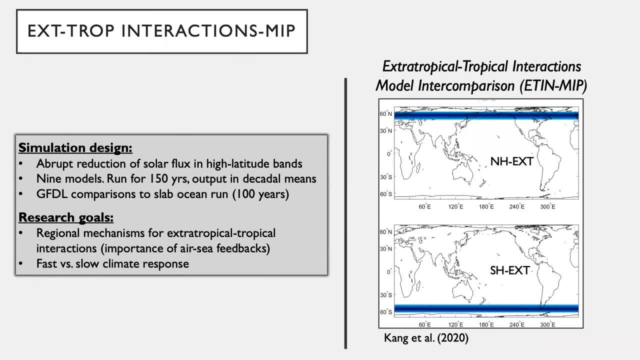 quickly and then, once the ocean starts to catch up, how does that influence the dynamics of the climate? And that's really the general idea of what's going on. I think ETENMIP might be a really useful tool to look at this fast versus this, transient versus more. 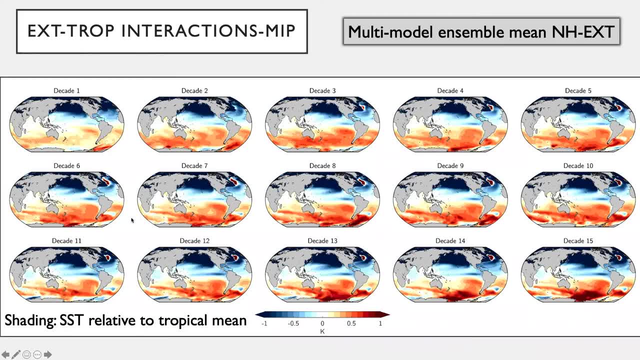 equilibrium response. So, very quickly, here are the decadal mean, northern hemisphere, extra-tropical SST responses. And keep in mind that all of the SST that I'm going to show you today are relative to the tropical mean. Basically, when you reduce insulation at the high latitudes, you get global cooling. But there are 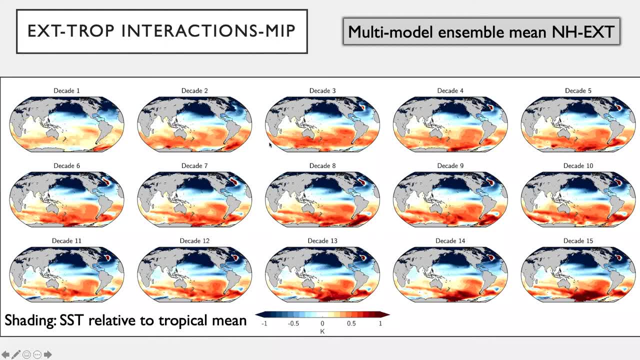 gradients, because not everywhere cools at the same rate. there are patterns. So this is a I'm going to show you a little bit of a just sort of emphasizing those patterns as gradients And you can see, going from decade one all the way to decade 15, the large scale pattern is set really quickly. So the atmosphere. 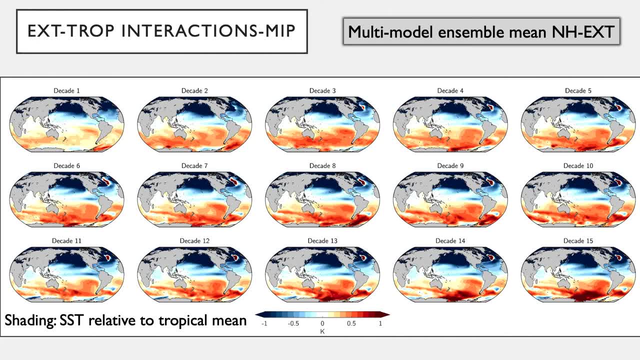 adjusts on the order of maybe- I mean really fast like a year, maybe two years. So you don't see much of the atmospheric adjustment to get sort of this broad inter-hemispheric SST gradient. But what you do see is over time you see a more defined sort of La Nina-like response. 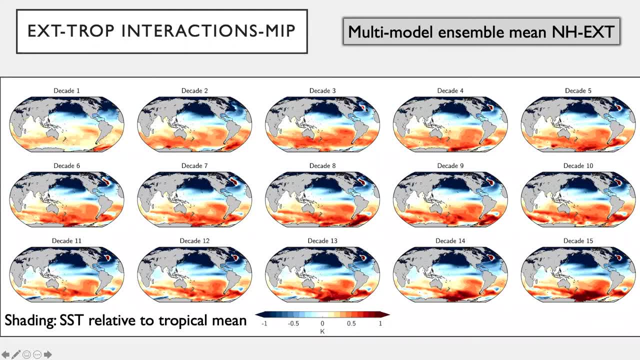 You also see sort of this warm- I don't want to call it a warming hole, but it's. you see this warming patch right here south of Greenland that we tend to associate with North Atlantic deepwater formation, as sort of the ocean begins to spin up. You also see sort of this Belus patch, which I 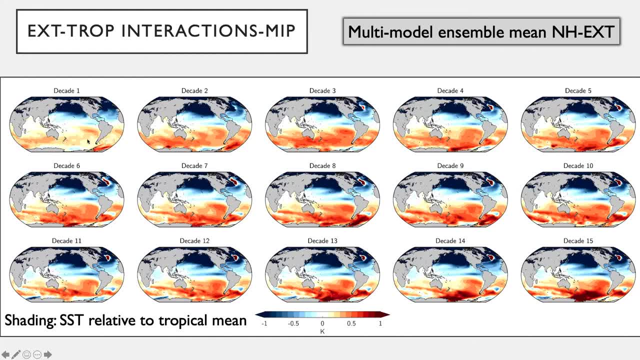 think is interesting, as the Malvinas current extension is doing something interesting over time that you don't see in the first decade. So I'll primarily be looking at just the first decade versus the 15th decade- and there's a lot of adjustment between that- And I'll also be 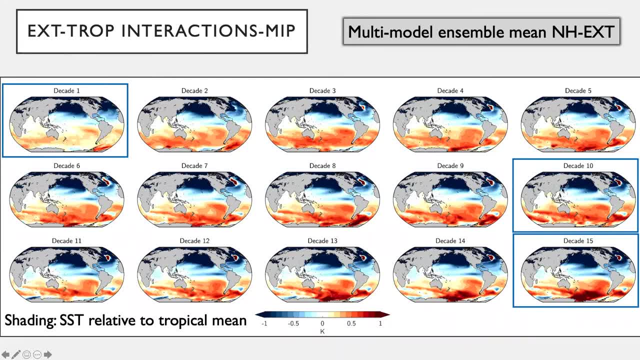 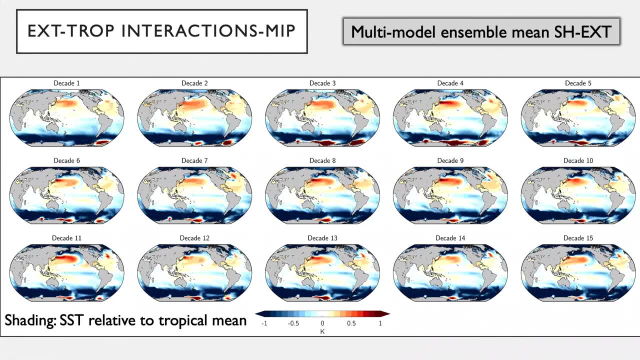 comparing to the 10th decade. When we look at the slab ocean runs. How am I doing on time? Okay, we're doing good. So this is the same idea, but for the southern hemisphere experiment I'm not going to dwell on. 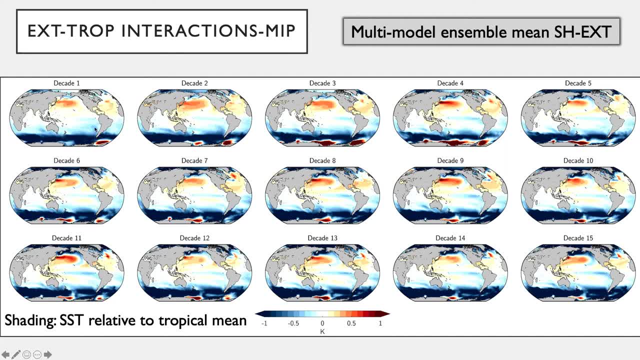 this one too much, but I just wanted to point out the same sort of features, that in the first decade it's more of just this large-scale inter-hemispheric SST gradient, whereas in the last decade you get a much more defined La Nina-like pattern here. And I should mention again that all of 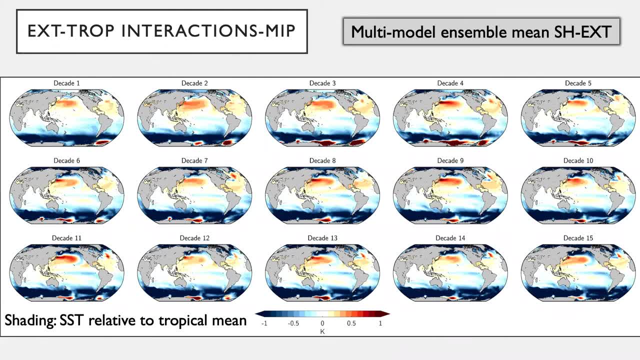 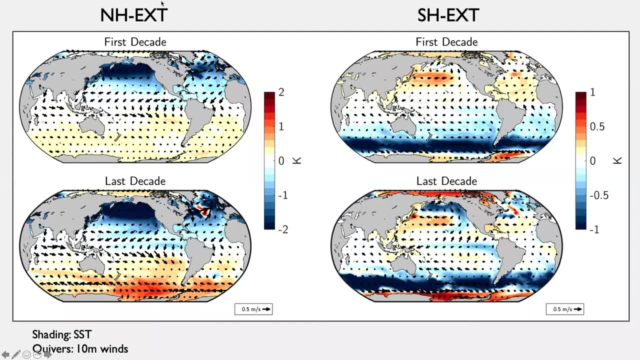 itted. this is one that, Alright, my computer cut out there. All of what I'm showing you here is the multi-model ensemble mean. So it's all 9 models averaged together. So here's the first decade and the last decade for the northern hemisphere and the southern hemisphere. 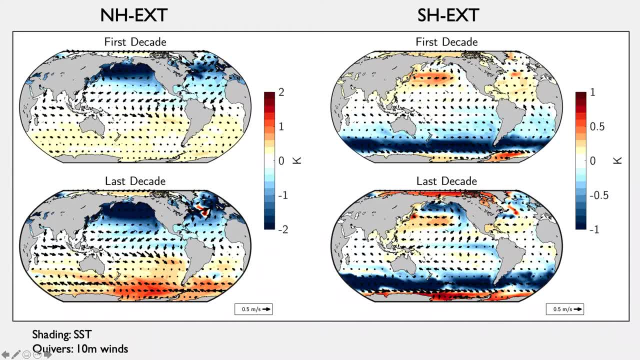 experiment with surface winds and a couple really interesting features that I want to point out here. For example, in the first decade you can see that the winds are purely cross-equatorial in the Atlantic and the Pacific And you get this beautiful C-shaped bend in the winds associated with Coriolis. 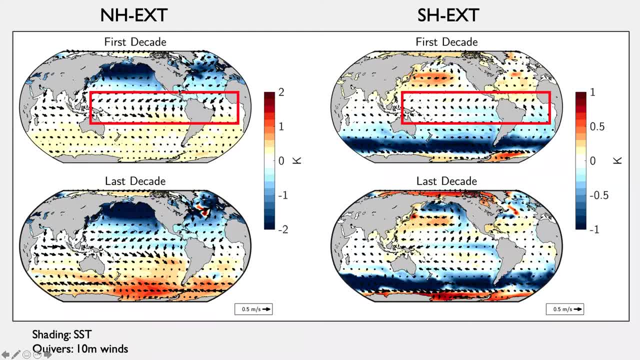 that large-scale sort of zonal mean response of the Hadley cell circulation to move energy to the colder hemisphere. In this case, because the surface winds are cross-equatorial, going southward that means the poleward branch or the upper branch of the Hadley cells is. 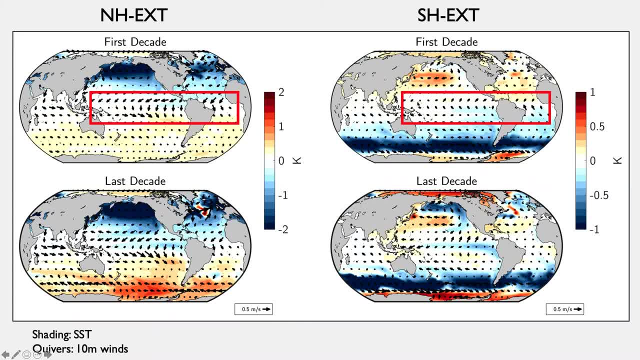 actually going towards the northern hemisphere. It's going in the opposite direction. So this is the energetic framework at play here. The atmosphere is adjusting to transmit energy from the warmer hemisphere to the colder hemisphere- Okay, whereas in the last decade, something really. 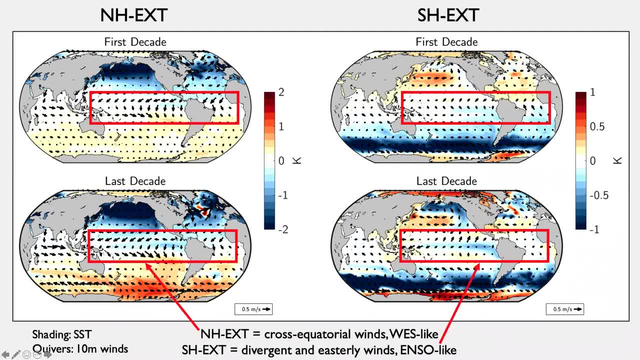 interesting is happening between the northern hemisphere and the southern hemisphere experiment. The northern hemisphere experiment is much the same: You still have that sort of large-scale cross-equatorial flow, whereas the southern hemisphere experiment, the winds are more divergent off the equator in the Pacific. 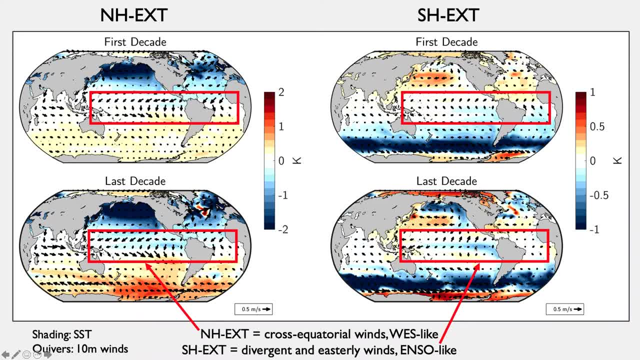 They look much more ENSO-like, much more La Nina-like. So it's possible that those winds are actually not responding to this large-scale inter-hemispheric temperature gradient, but they're responding to more local SSTs, which indicates that SST feedbacks might be more important for this. 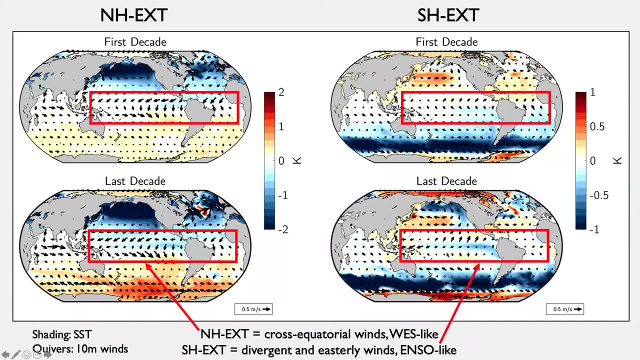 southern hemisphere experiment, Potentially ocean dynamics as well. So we can look at ocean dynamics a little bit more closely. Let's see: Click, Oh, here we go. So what I'm going to do for the rest of this talk is actually: 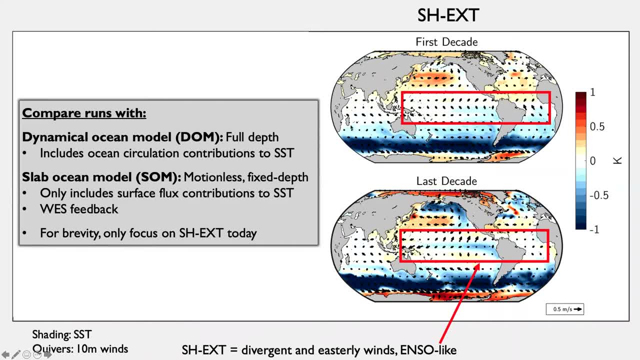 just focus on the southern hemisphere experiments just for brevity. Hopefully I'll follow up with a future talk someday and I'll show you guys the full results. but just I'm going to focus on the southern hemisphere for today. for the rest of the talk, 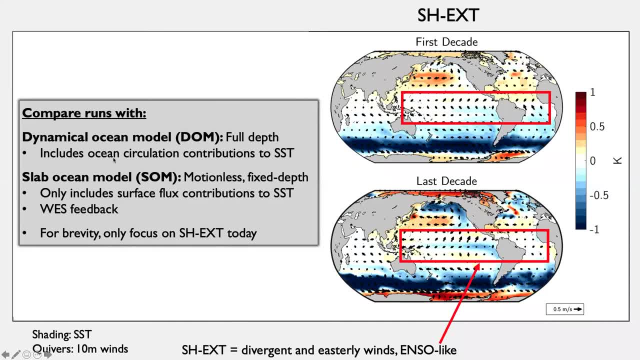 And we'll compare to a dynamical model which has a full-depth ocean, includes ocean circulation, and compare it to a slab ocean model which is a motionless, fixed-depth ocean and only includes surface flux contributions to the SST. So a comparison between these two will. 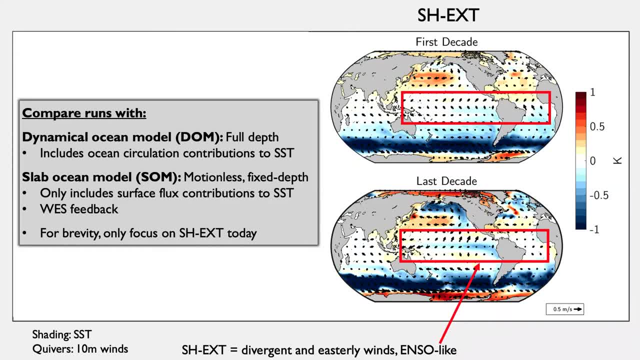 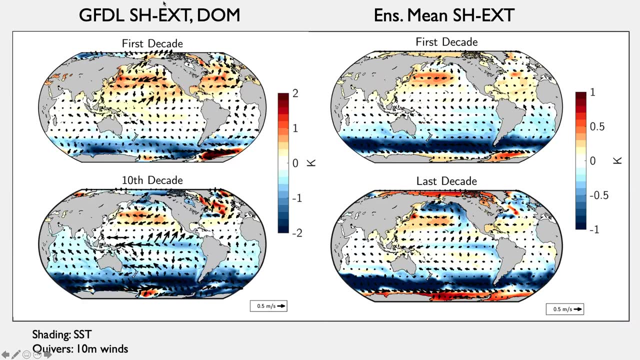 say something about the the importance of ocean circulation in, in advecting heat around, basically, And what's important is that the slab ocean has coupled feedback- things like WES feedback- as well as does the dynamical ocean. Okay, so this is the dynamical ocean model. This is just GFDL. This is again. 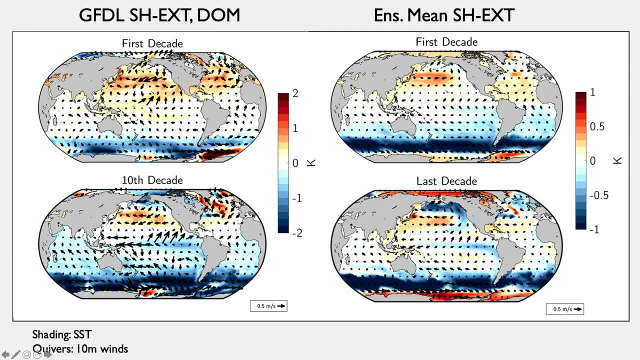 the ensemble mean from all the models. I just wanted to show you that GFDL looks a lot like the ensemble mean, just not as smooth. It's just a stronger version of the ensemble mean, basically- And I want to compare the dynamical ocean model to the slab ocean model. So this is the slab response. 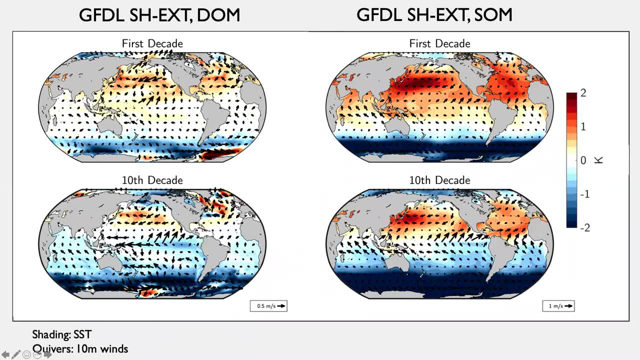 And basically what we can see is that the slab is much more of that energetic framework. It's just the atmosphere adjusting to that inter-hemispheric energy gradient, where you have cooler southern hemisphere and warmer northern hemisphere, and it's adjusting accordingly The dynamical ocean model. 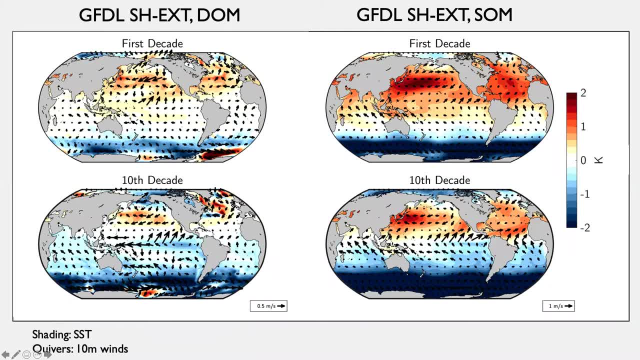 is able to do a lot more because obviously it has ocean heat transport And, as a result, the wind variability associated with that SST change is feeling something different as well, For example, in the tropical North Atlantic. you can see that the SST response. 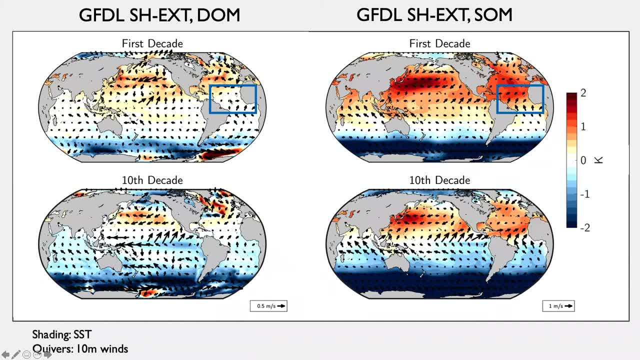 is much stronger in the slab ocean, but in the dynamical ocean it's dampened And I'll show you a little bit later. but that dampening is due to Ekman infection, which isn't present in slab ocean models, Also in the 10th decade. here, if we look at the wind field in the slab, 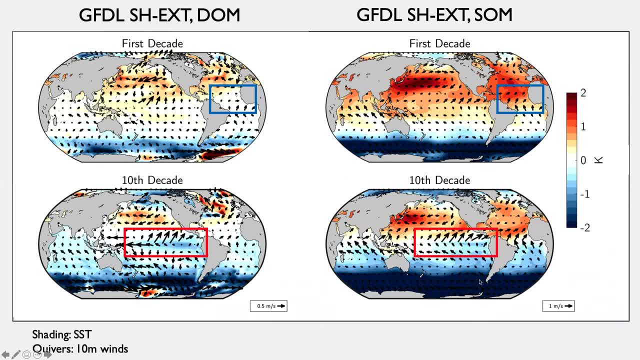 you get that cross-equatorial wind that is much more related to that zonal mean energetic framework, whereas in the dynamical ocean you get that divergent flow that looks a lot more like La Nina and it seems to be due to the importance of having ocean circulation. 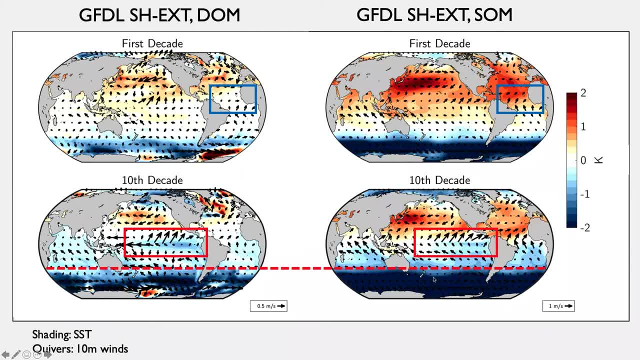 And one other thing I wanted to point out is just the latitudinal extent of the coldest anomalies, in this case In the slab. the temperature anomalies are able to extend much further equatorward in this case, So that also suggests that ocean circulation is dampening the extent. 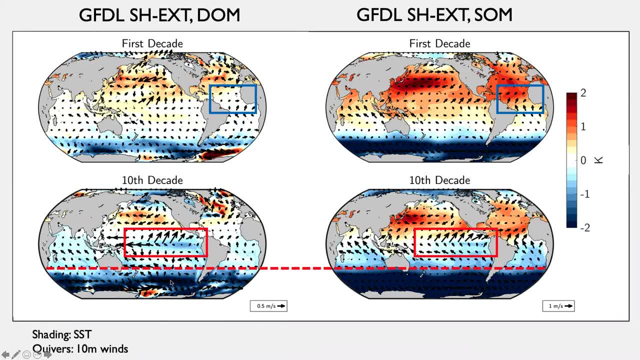 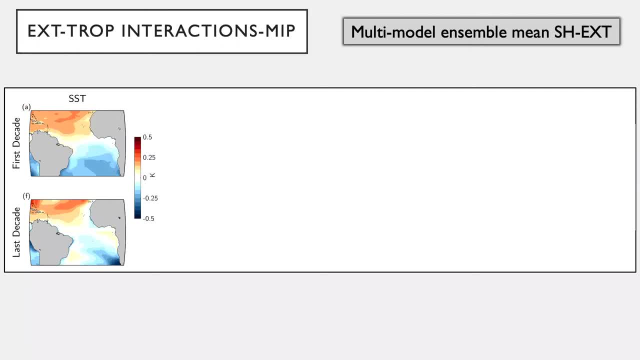 to which these anomalies can escape the high latitudes. So I want to focus on the Atlantic, just as a region, to illustrate the power of this tool. Again, this is all preliminary. I haven't quite analyzed it in depth, but I wanted to just give you a sense of the direction we're going with. 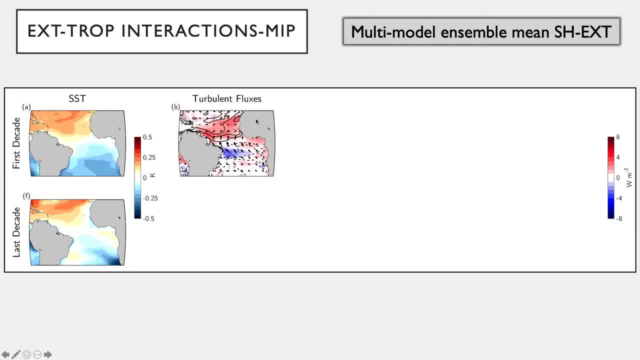 this. So we're going to compare the first decade to the last decade and we can look at turbulent fluxes, radiation, in this case Ekman adduction, and we can calculate everything else that's going on in the ocean as a residual. And this is again back in the multi-model mean sense. So blue here is. 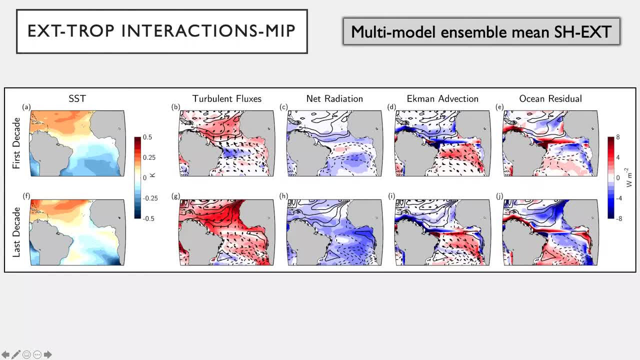 cooling and red is a warming And we can look at that as well in the last decade. So a couple things to point out is that in the first decade you can see this nice cross-equatorial wind field again and you get a meridional dipole, in this case, of the turbulent heat fluxes. 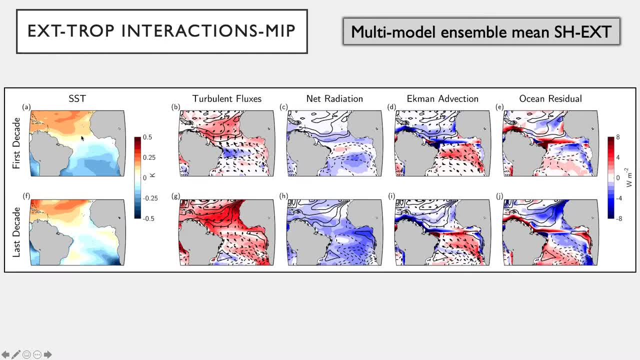 that are helping to maintain this cross-equatorial SST gradient. So again, WES feedback is effective in maintaining in a quasi-equilibrium sense cross-equatorial SST gradient, But because we have a dynamical ocean, it's dampened by Ekman adduction. 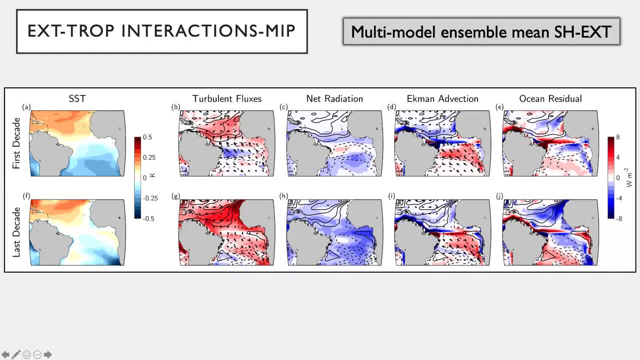 So this is actually a well-known thing- that Ekman adduction dampens the tropical response to high-latitude forcing in this case. So it would be stronger and that's why it's stronger in this lab. One other thing I want to point out is the increased role for net radiation. 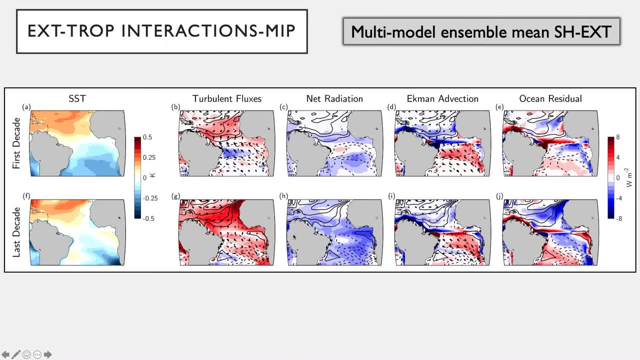 You can see that you get broad cooling due to radiation changes throughout the tropics, which is helping to dampen. It accentuates the anomalies in the South Atlantic, but it dampens them in the North Atlantic, So we can look at why that is. I said all this. 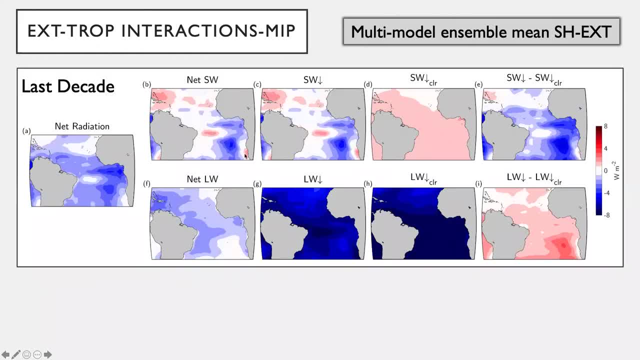 but we can look at why that is by breaking down the radiation into its individual terms. A couple things to highlight. If we look at, say, the shortwave, this is just a net shortwave- downward shortwave clear, sky cloudy- This is the net down minus net clear. So this gives you. 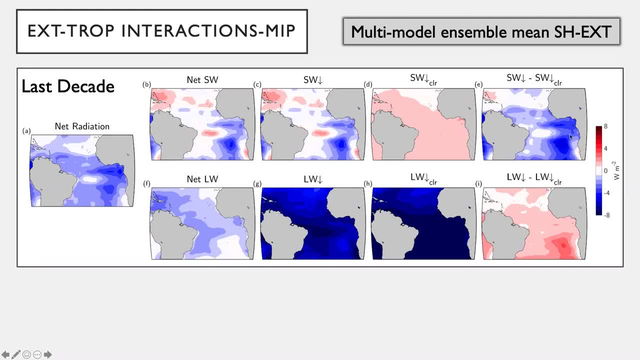 the effects of things like low clouds. You can see that as you cool the South Atlantic, you increase marine stratocumulus. basically You increase low cloud fraction, which reduces shortwave. So this is evidence again of low cloud SST. 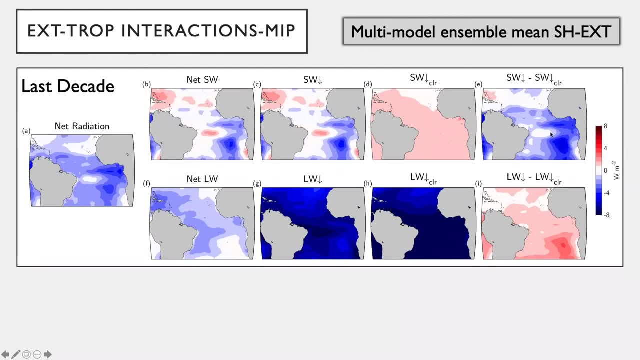 Feedback. This seems like it's an important regional air-sea interaction that maintains some of these SST anomalies in the Southeast Atlantic. Another thing that is really interesting is this broad cooling from downward longwave, And this looks a lot like water paper feedback. 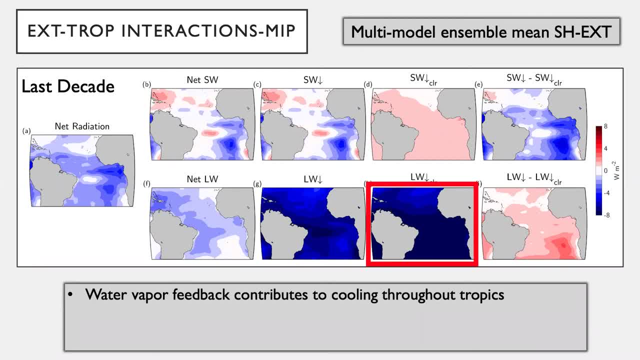 where, if you cool the world basically uniformly- well, not uniformly, There are patterns- But if you cool the tropics, you reduce the amount of moisture in the water, column from Clausius Clapeyron, which reduces downward longwave radiation. So that is another cooling effect. 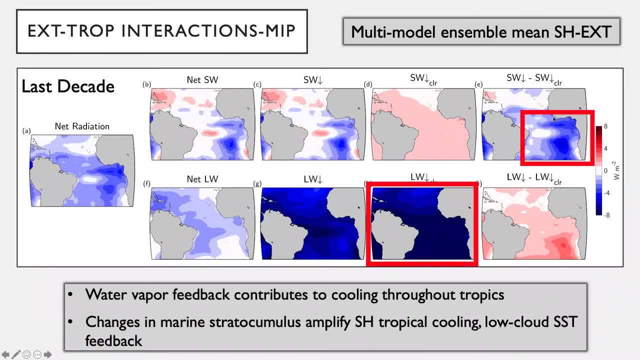 throughout the tropics. is this water paper feedback? And then again, the effect of clouds is pretty evident in both the cloudy shortwave and the cloudy longwave as well. So with that, I think I'm out of time. Well, we have about 10 minutes for questions and discussion. 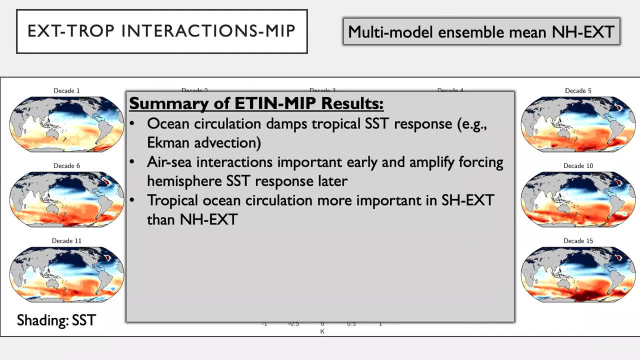 I'll just summarize here Ocean circulation. it seems to be important in dampening tropical SST responses through eckmann advection. Air-sea interactions are certainly important early through getting the signal down into the deep tropics. I think if I look at the first 20, 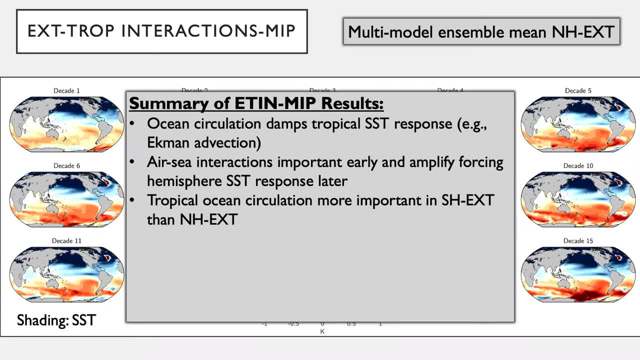 years of each of these model simulations, I might see more evidence of, say, that first component of WES feedback, that propagating component, as being important. But it is. WES feedback is certainly important in maintaining these tropical SST gradients And then the tropical ocean. 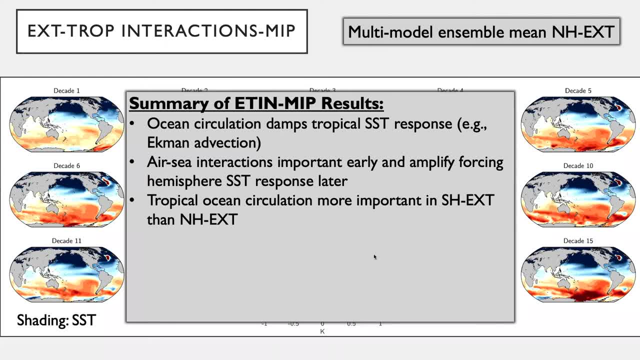 circulation seems to be more important in the Southern Hemisphere experiment and less important than the Northern Hemisphere experiment later on. The next steps. again I'd like to isolate sort of that quick response in the first 20 years which I'm getting that data soon And then we're also. 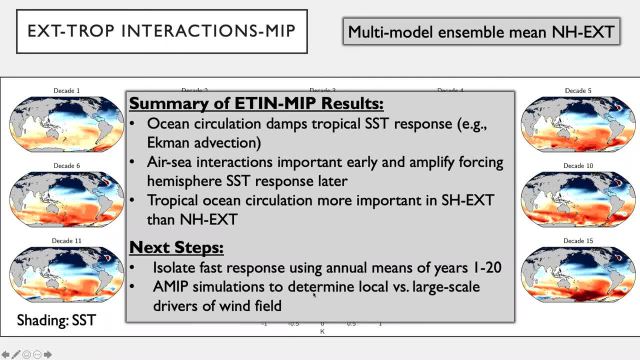 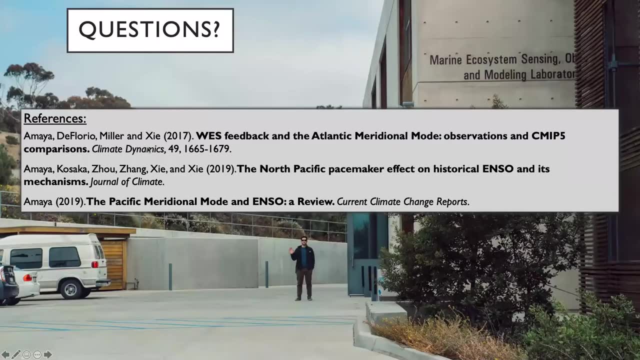 running some AMET simulations to determine the local effect of SST versus sort of that large scale inter-hemispheric SST effect on the wind field, to again see if air-sea interactions are important and where regionally they are important. All right, So with that, here are just some. 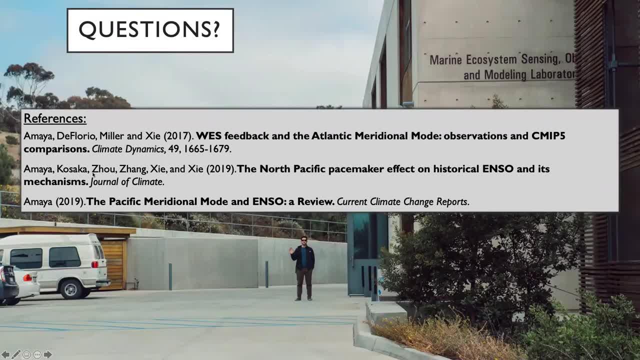 literature that I'm going to show you- And then I'm going to move on to the next slide- Came mostly out of my PhD. that can help further explain what I discussed in the first part of the talk. We're working on results And I'm hoping to write that up in the coming months. 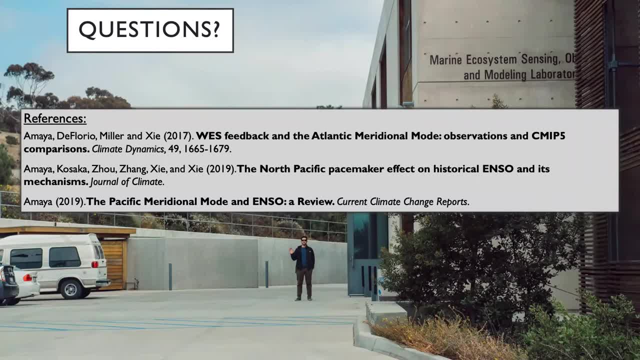 And I'm happy to chat with anybody who has any comments or questions about it. So with that, I will take any questions. Thanks, Great, Thanks a lot for an excellent talk. So if you have any questions, raise your hands. OK, we've already got some, So, Jerry, I will. 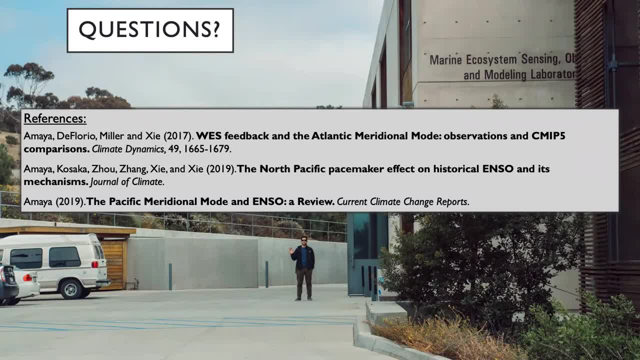 unmute you OK, thanks, And thanks for the nice talk, Dylan. I was just curious about this EtinMIP. How did they decide what latitudes they put in where they cut off the incoming solar? That's a good question. Truthfully told, I'm not 100% sure that that Kong et al paper. 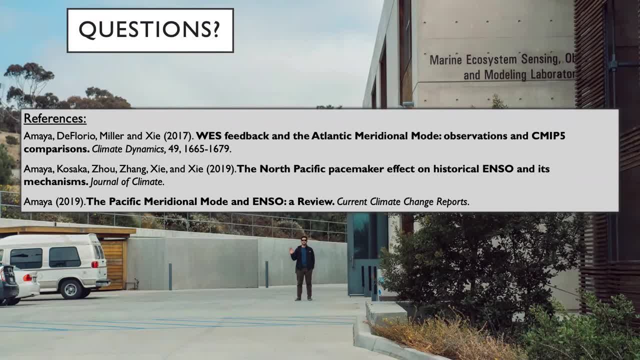 that 2020 paper is a BAMS paper, where they summarize all of the EtinMIP modeling framework. I can't remember their justification, to be honest with you. I'm sure they had a good reason. I know that historically, people have cut it off at like 60 to 45, something like that, But I think that 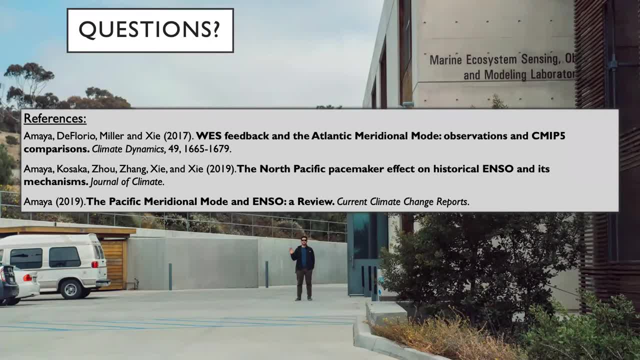 paper would have the explanation. OK, thanks Clara. Yes, Thanks, Dylan. Such a good talk. I wanted to come back to your PMM results. I was just interested in your thoughts about future changes, possible changes in PMM strength and or polarity with global warming and if there might be…. 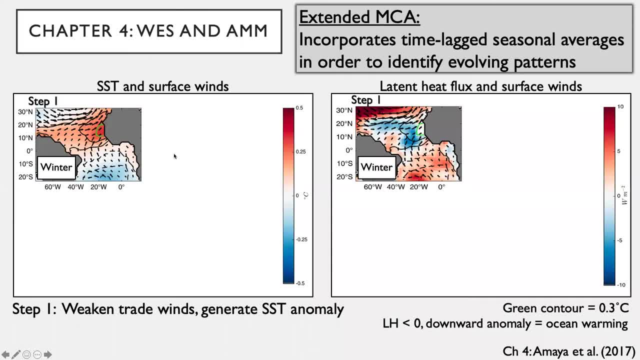 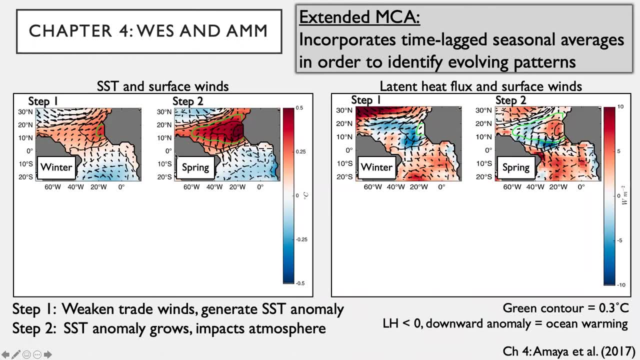 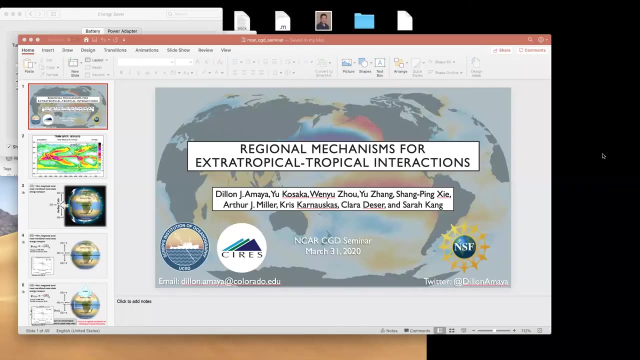 Yeah, that's a great question- Let me just finish So- and if there might be then some reason to investigate whether models projections of changes in Vaiunatien endsten varse and in the relative proportion of central positives… of Central Pacific events, whether that. 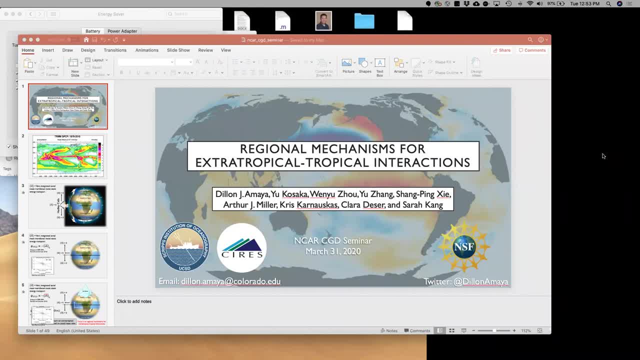 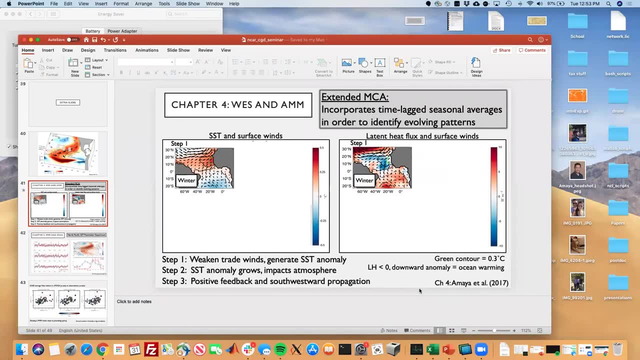 might be tied to future changes in the PMM. That is a very good question. I know people have looked at thermodynamically how WES feedback will change in a warmer world And the summary of it. that's what I was trying to get to here on the extra slides. 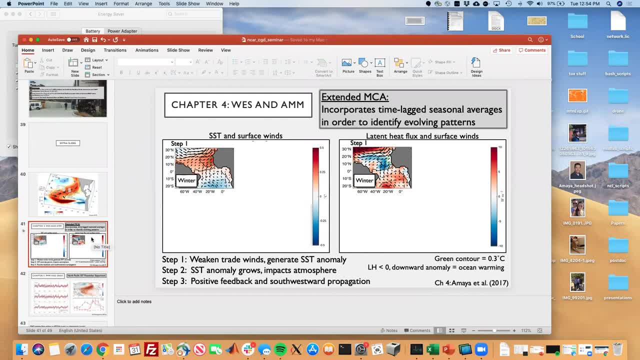 I'm wondering if I have It. doesn't look like I have it, But if you look at the WES parameter, which is the change in heat flux for a given change in zonal wind anomaly that increases under global warming for good thermodynamic reasons, 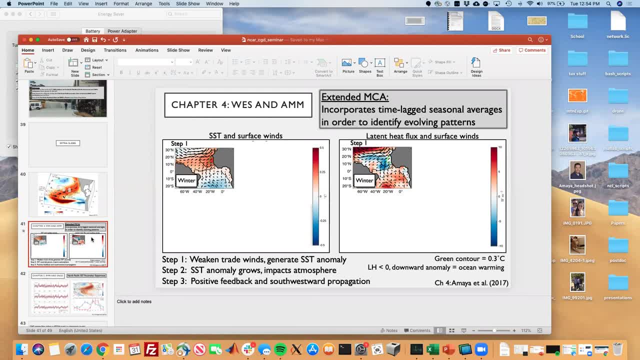 So people have argued that the PMM will become an increasingly important part of ENSO under global warming. What people haven't done- that I've seen at least- is taken the step that you've just taken, which is really interesting- that the projected increase in CP ENSO. 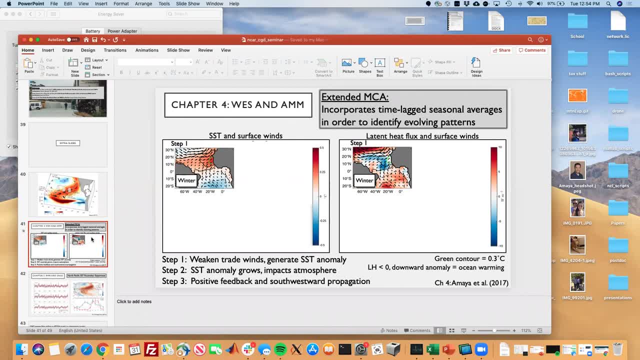 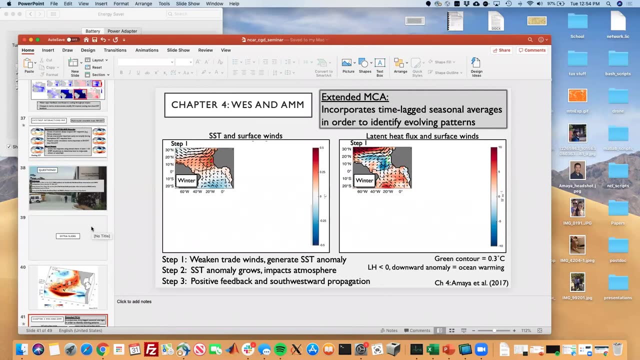 versus EP ENSO could be due to this effect. I don't know. That's an excellent question. Thanks, Haiyan. My question is about the first thank you for the nice talk, Dylan, And I'm wondering about your Hohemuller diagram. 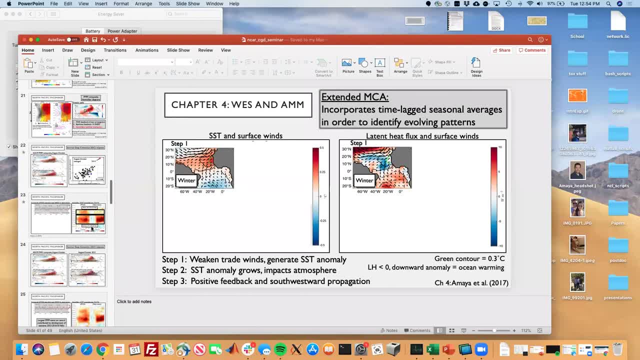 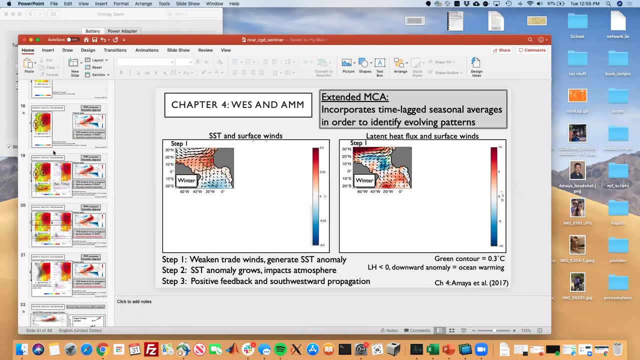 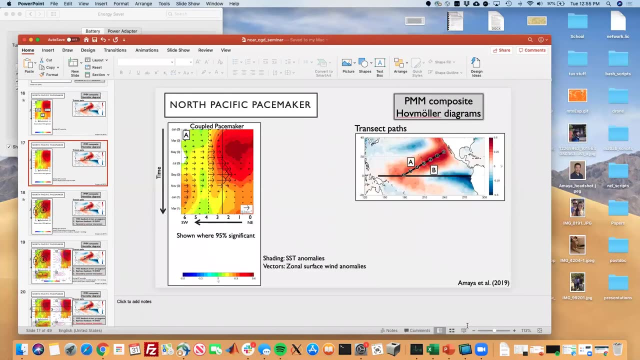 And I'm wondering why it takes nine months for the signals to propagate to the. You kind of hinted that the SST anomalies propagate to the equator, But I am wondering, since it looks like the wind anomalies started to appear in May earlier way- earlier than SST. 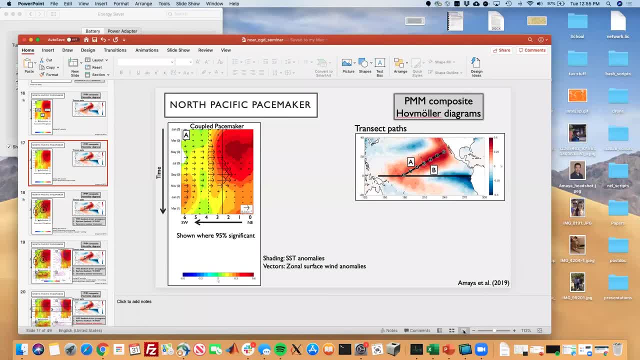 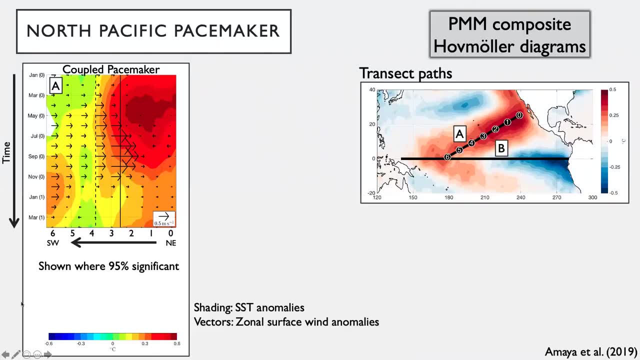 whether the wind anomalies are caused by just remote response to the heating associated with the PMM or it is really SST anomalies propagating to the equator. OK, You cut out just a little bit, but I think I understood the gist of your question. 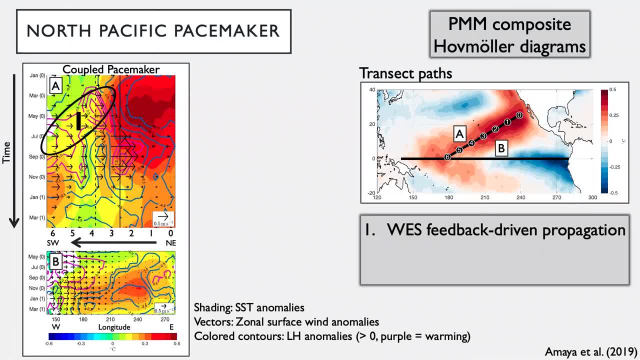 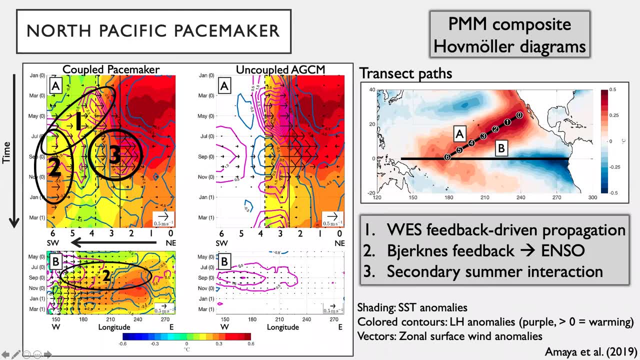 If I don't answer it, let me know and I'll try again. I just want to get ahead to this plot here. So you're wondering why we get wind anomalies as early as May. if the SST anomalies are here, They don't arrive until later. 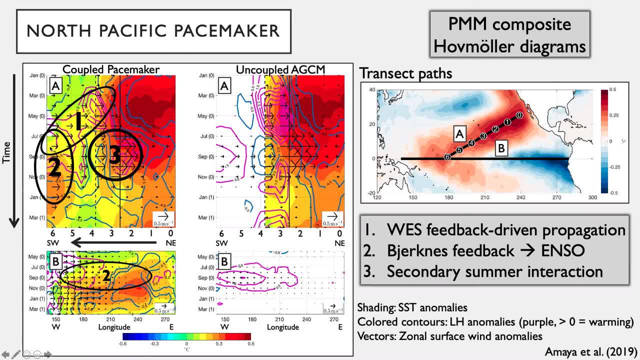 Is that what your question was? Yeah, I'm wondering what cause of the west feedback can happen really fast. It doesn't need to take, It's just a model for. Yeah, I think basically what's happening here and comparing to the uncoupled run is useful. 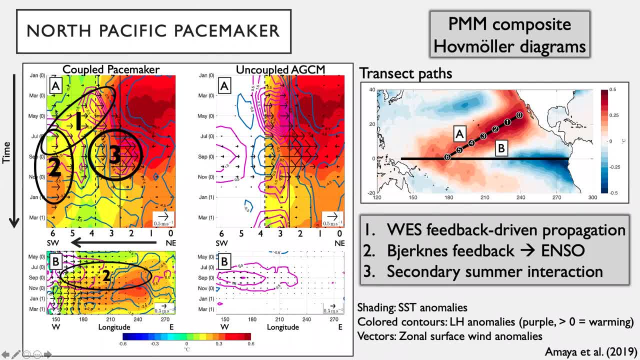 The wind anomalies here are being generated by- I mean, I can't say for sure exactly which SSTs, but my hunch is that they're being driven by the warm SST anomalies that are at higher subtropical latitudes. So this is still that WES feedback component, where 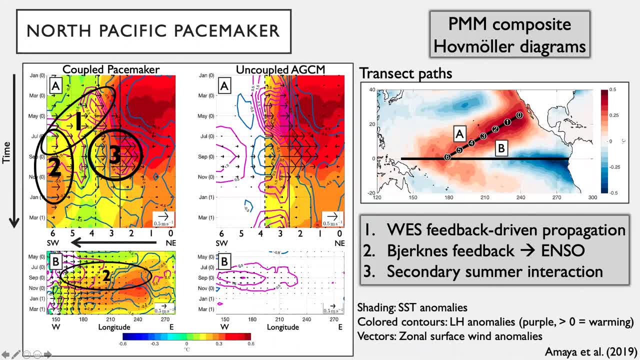 if you remember from the schematic, we just had that lobe of warm anomalies And that's that. That's what's going on here, And these winds are being driven in across the equator by this warmth here, And it's not this warmth up here because you 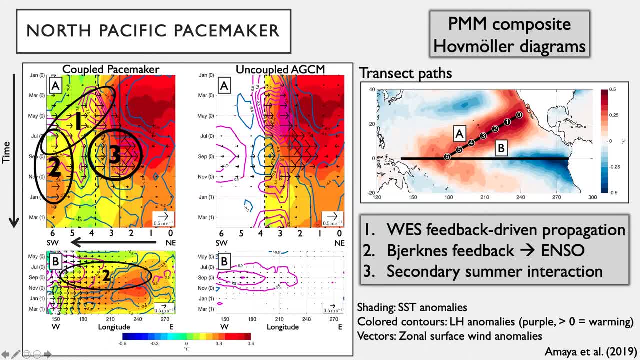 don't get it in the uncoupled run. You don't get any of these winds in the uncoupled run. So I think these winds have to be responding to SSTs that are not being restored by the model They have to be from SSTs that are 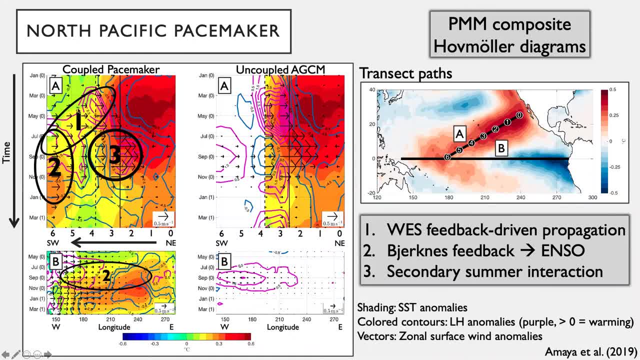 on this side of the dashed line And my hunch is that they're coming from the warmth that is here, which is WES driven, So I do think that the wind anomalies around the dateline are totally consistent with WES feedback. 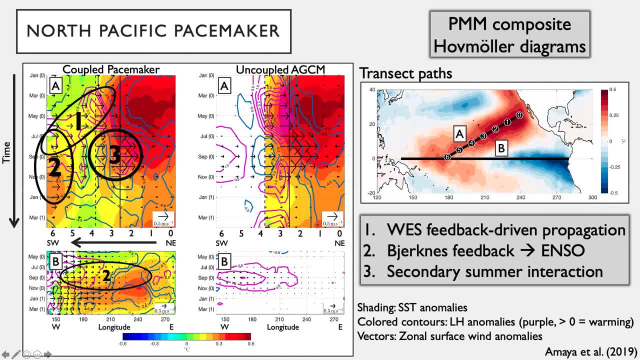 But the SST signal just takes some time to get down there in this sort of composite sense. But I agree with you that WES, feedback-driven propagation, doesn't necessarily take. in this case it takes. it goes from about March till about July, So it doesn't take however long. that is four months. 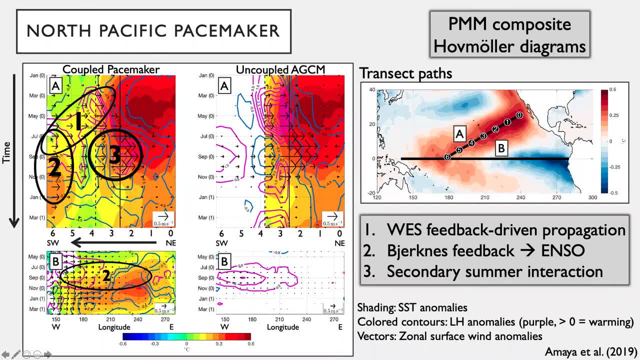 In reality it could take a month or maybe a couple of weeks. I'm not sure It is a much faster process than what this implies. Thank you, Mm-hmm. OK, So next we have Cecile Penland. 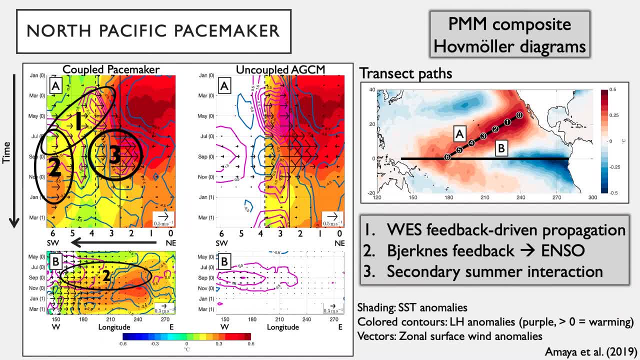 There we are. I have a comment and a question. I really think you've done a lovely job of showing how the WES mechanism accounts for the upper branch of the optimal structure that Prashant and I found in 95. But there was a lower branch too to that. 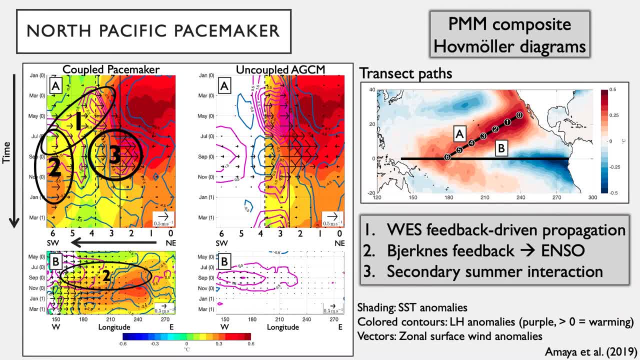 But it's not the optimal structure And I'm wondering if that's when the negative branch of the PMM is somewhat interrupted. And I would call your attention to the other oceans, In particular, during 2014-15, there was a very strong contribution from the Bermuda. 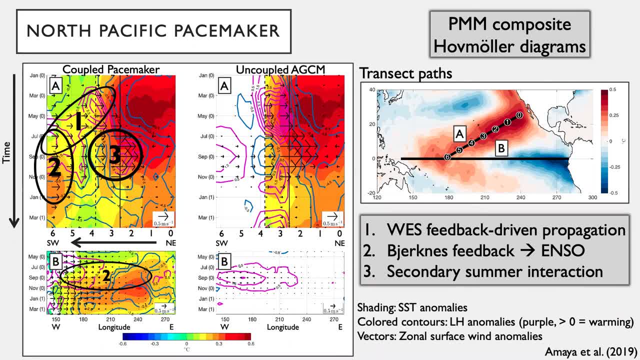 High, which made that negative part of the PMM much stronger. But it's significant. It's significant It interrupted the development of the El Nino during that section. Also there's a huge Rossby wave response in the southern hemisphere that can affect the trade winds in the southern tropical Pacific in the east. 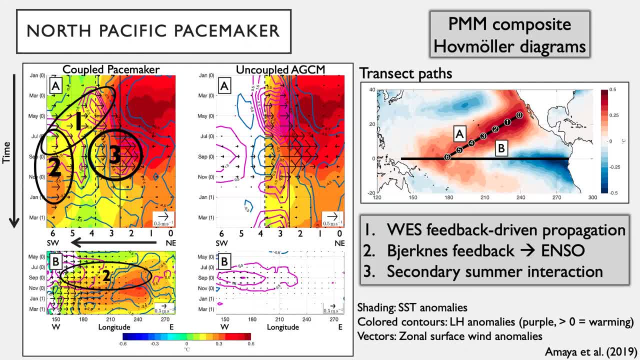 And I just want to call your attention to the other half of the optimal structure. that is not explained by your mechanism. But the question I have is about the multi-model ensembles, just uniform bias, negative bias of the SST in the western Pacific. 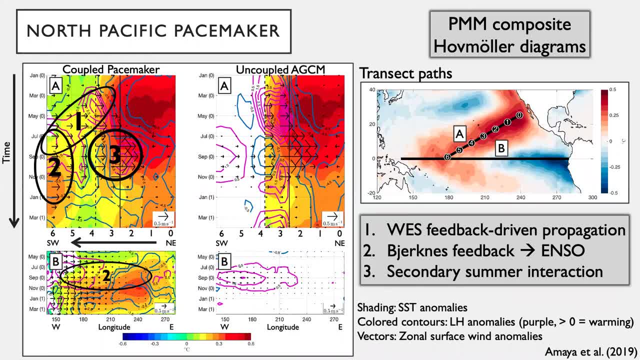 And according to your results, could that be due to overly strong Ekman pumping? Are you referring to S and MIP? Yes, I mean the short answer is yes. Again, the short answer is: I'm not sure. I'd have to look. 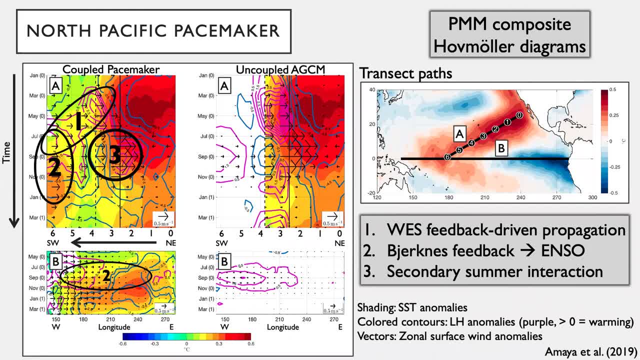 That is a good question Whether – I mean, it might be one way to – I'm not sure – I guess my point is that I'm not sure that S and MIP is the framework to diagnose that particular problem, because they are being perturbed in a weird way. 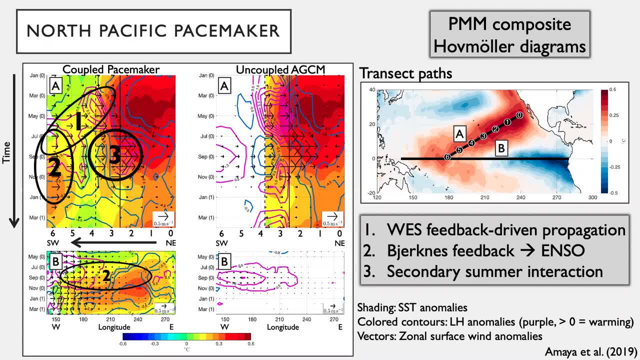 I think maybe if you had a MIP of just control simulations, that might be the best way. That would be the way I would go about answering that question if I was going after it was to get some unperturbed simulations. But I'm not sure about the Ekman bias. 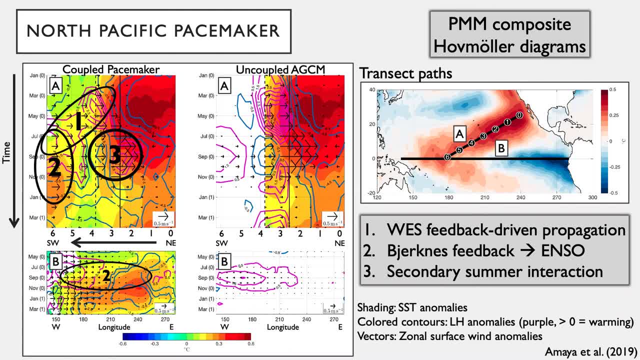 And I just want to respond to your comment about the southern lobe. I totally agree that the southern – sort of the cooling calf of the meridional mode is important, But I guess historically people have not focused on it as much because most of the meridional mode work initially was in the Atlantic. 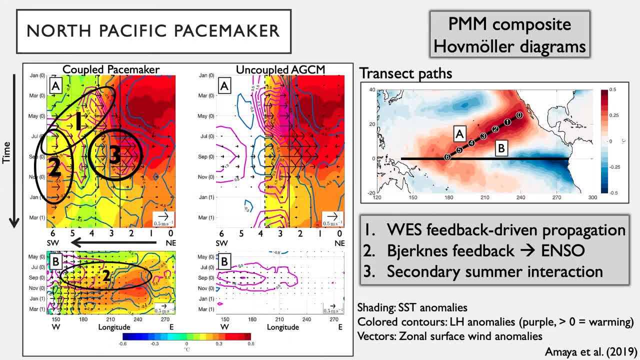 And when they focused on sort of that southern lobe versus northern lobe, they found that that southern lobe – Yeah, The southern lobe can be often statistically independent of that northern lobe, which is a little confusing given the coupling between that northern hemisphere warming and the southern hemisphere cooling. 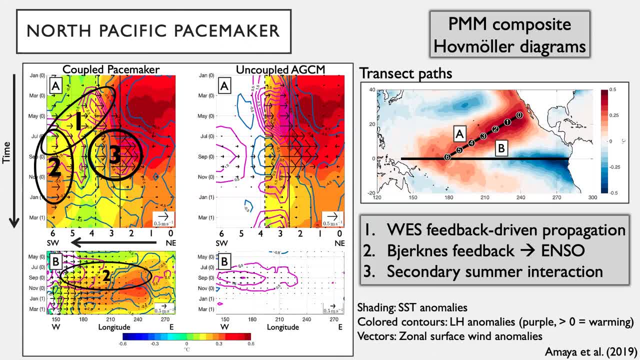 But I guess my point is that the southern hemisphere lobe can also have a mind of its own which makes it harder to sort of look at the large-scale dynamics relative to that northern lobe. But that is a good point to sort of keep both of those in mind. 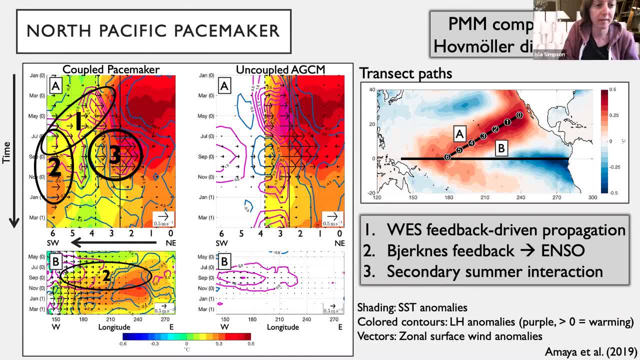 Okay, We have two more questions, Sally. Hi Dylan, Nice talk. I'm just wondering for the AtomIMP. you mentioned cloud changes. Do you have an idea of what's driving the cloud changes? Is it like SST only, or is it stability or advection? 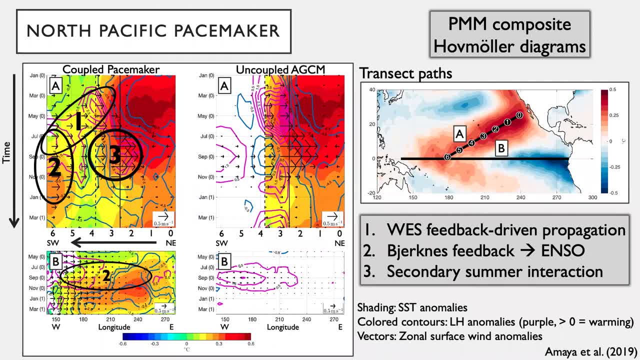 Again, good question. My guess is that it's local SST And our AMIP simulations that we have running right now. they're very similar, Okay, So for example, right now, where we're forcing an atmospheric model with the multi-model ensemble, need SST that will be able to tell us if local SST is important. 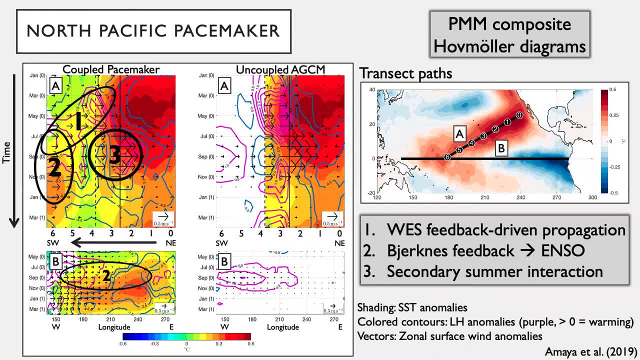 Basically, if we can see the same low cloud changes in the AMIP simulation as we do in the dynamical model, that'll be one way to sort of diagnose that. But my hunch is local. SST is important. Okay, Cool, Thanks. 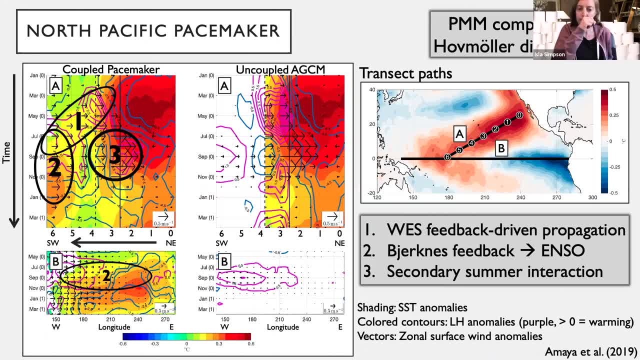 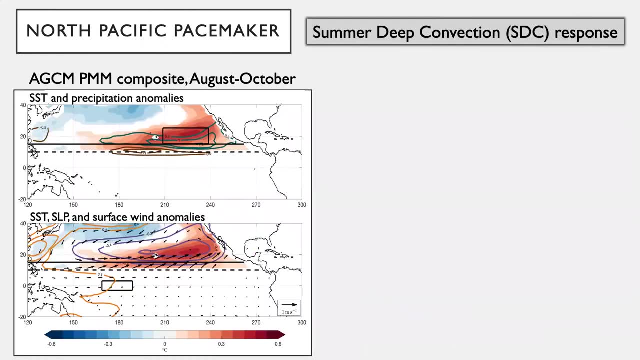 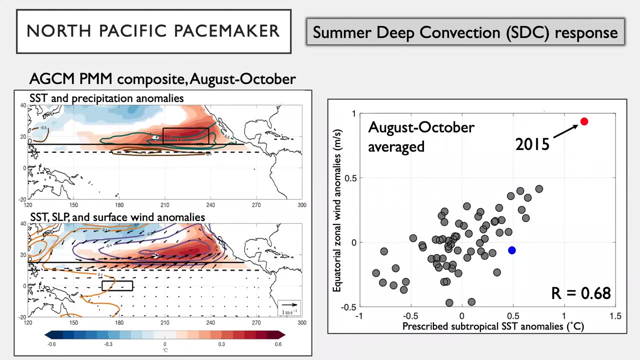 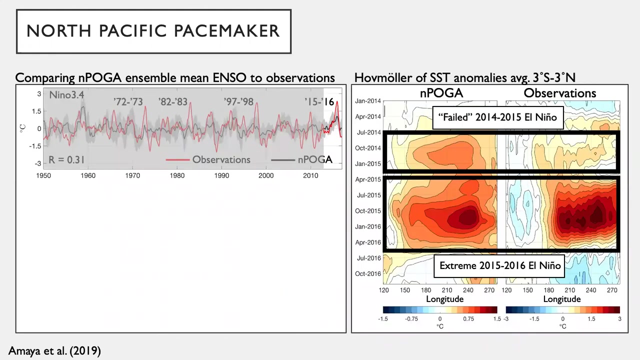 And then Clara. Okay, This is about the AtomIMP. So I wanted to respond to Jerry's question about so why those idealized solar constant perturbations were placed at such high latitudes. I think one motivation actually came from the work that Jen Kay had done on showing the sensitivity to southern ocean cloud SST interactions and how, in the presence of ocean dynamics, you can actually see that. 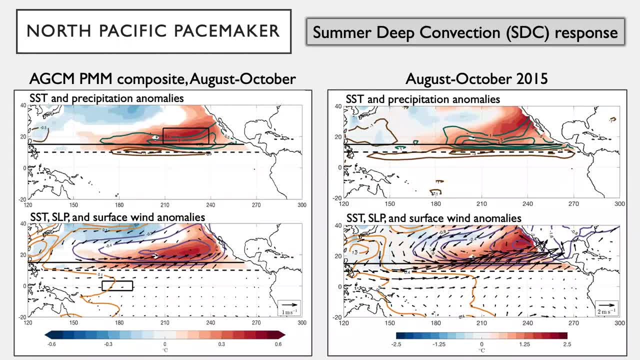 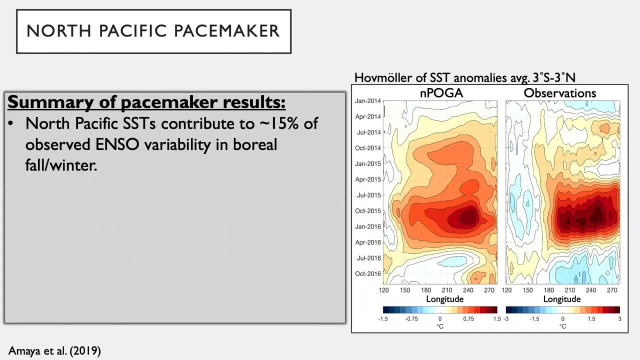 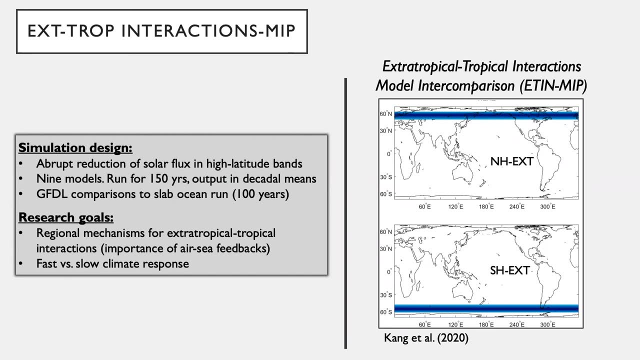 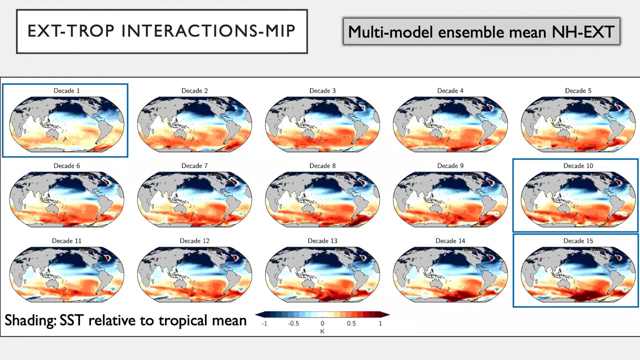 And in the case of ocean dynamics, you can actually get a tropical response. So I think that was one motivating factor for why those perturbations were placed at such high latitudes. But my question, Dylan, for the AtomIMP, the slide that had the northern hemisphere experiment with the first and last decade- yeah, just the first and last decade- with a wind field on it. 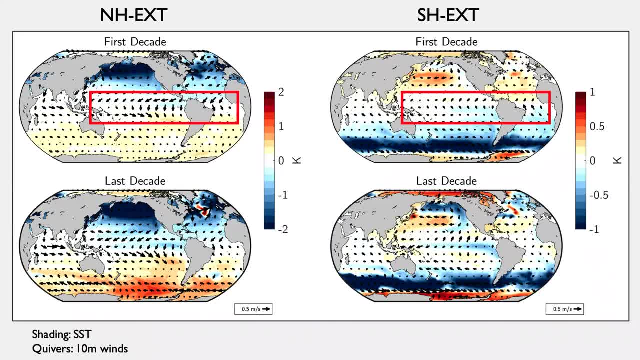 Yeah, There we go. Yeah, I was really interested. the lower left plot, the last decade for the northern hemisphere experiment that the wind changes. the easterly wind anomalies over the southern ocean are so prominent and probably helped to cause that warming over the southern ocean. 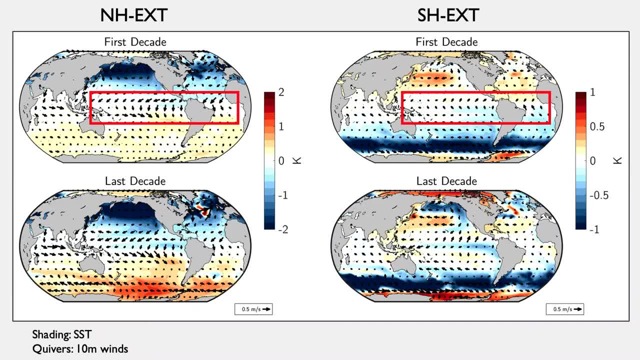 And obviously they're not present in the first decade, And I wondered if you had any thoughts about what might be producing that response. Yeah, it's a good question. I think you guys can see my cursor, I hope. I think the easterlies here might be associated with this sort of broad- I guess it's cyclonic circulation in the southern hemisphere. 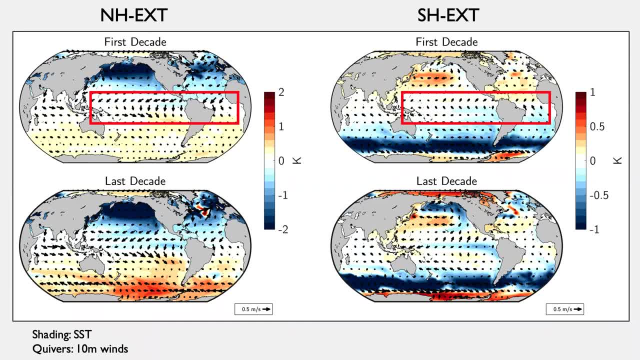 And I'm wondering- I'm sort of interpreting this on the fly here, but I'm wondering if that might be related to the PSA. So maybe this Latinx Like pattern is driving some sort of standing teleconnection that is driving the circulation response. 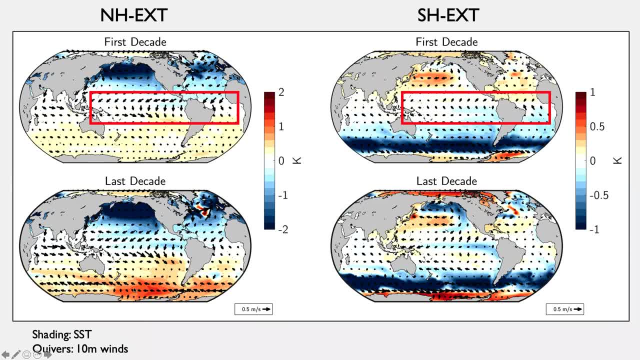 But it is also associated with, like a broad, zonally uniform easterly change, So it could be related to- I think you and I had looked at- the zonal stream function, the mass stream function and the ferrule cell is weakened in the opposite hemisphere. 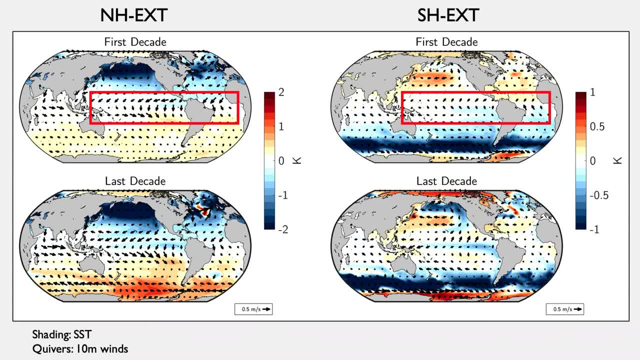 So in the southern hemisphere the ferrule cell is weakened, So that would also weaken the westerlies in the southern ocean, So that It could be related to some eddy dynamics. I'm not sure. Well, it's very interesting, right to have such a prominent signal at high altitudes. 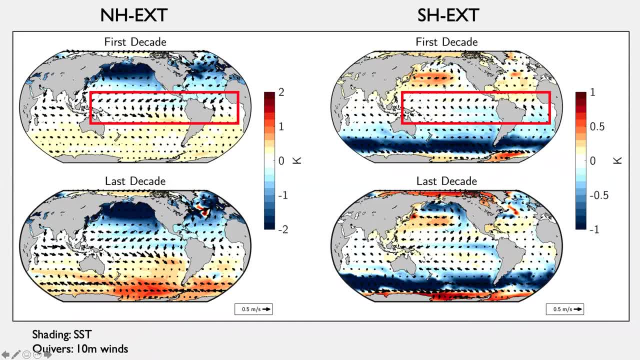 Yeah, definitely. And also if you in the southern hemisphere experiment, it's kind of hard to see because the areas are black, but you do get an increase in the westerlies, I would say a marked increase. even though the forcing is in the southern hemisphere, you still get a strong surface wind response. 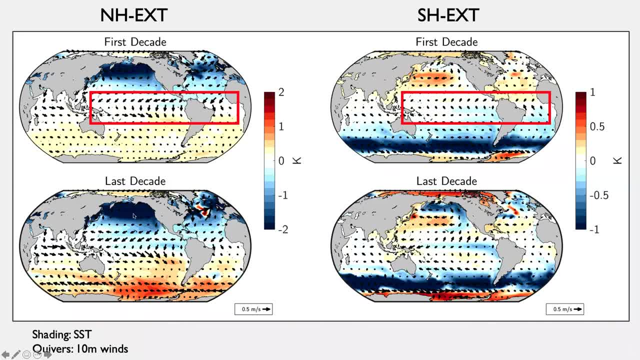 Whereas in the northern hemisphere it's not. Again, it's hard to see, but the winds aren't really. they're really not that strong relative to the opposite case, But you do see the opposite hemisphere wind response for sure. Thanks. 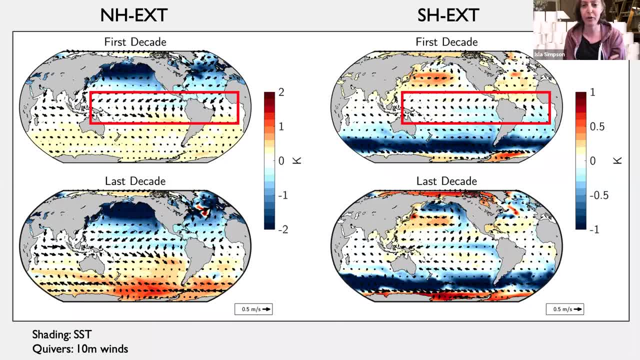 Great. Well, we're just a little afternoon now, so I guess we'll leave it there, unless anyone has any other burning questions, And thanks, Dylan, for a great talk, And so we'll see you all again next week. We have Alison Wing from FSU who is going to talk about 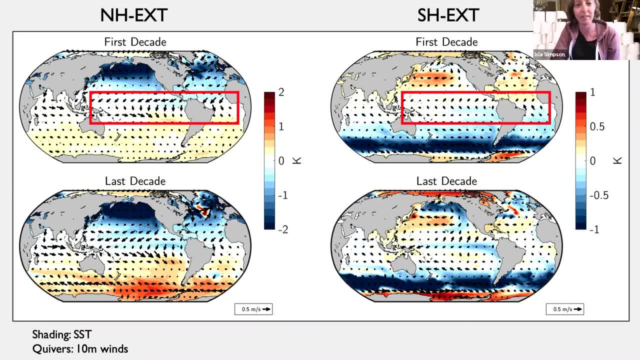 convective aggregation and climate sensitivity next Tuesday. So have a good week And thanks again, Dylan. No problem, Thanks everybody, Thanks.